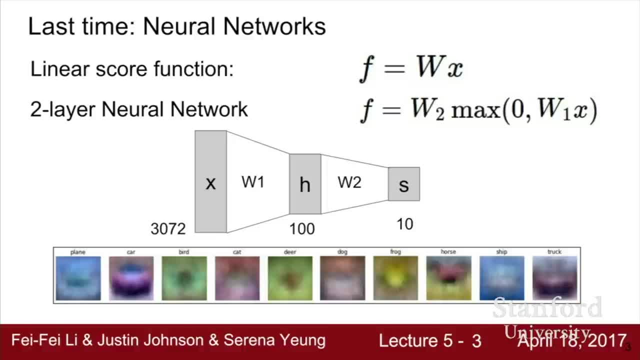 to learn intermediate templates that are looking for, for example, different types of cars- right, A red car versus a yellow car, and so on- And to combine these together to come up with a final score function for a class. Okay, so today we're going to talk about convolutional neural networks. 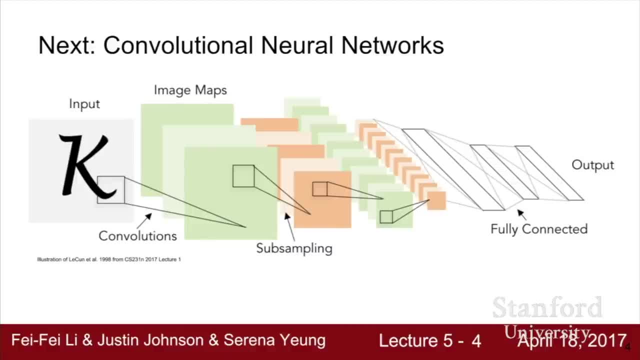 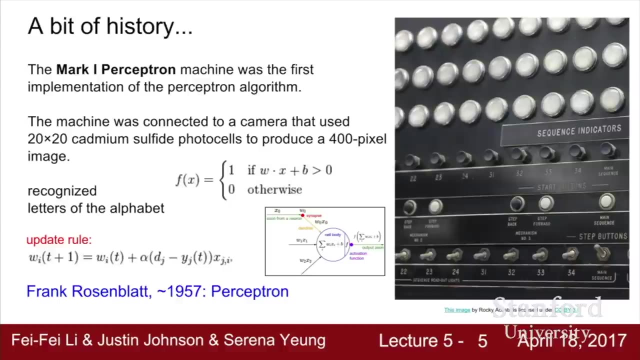 which is basically the same sort of idea, But now we're going to learn about convolutional layers, that reason on top of basically explicitly trying to maintain a spatial structure. So let's first talk a little bit about the history of neural networks and then also how convolutional neural networks were developed. 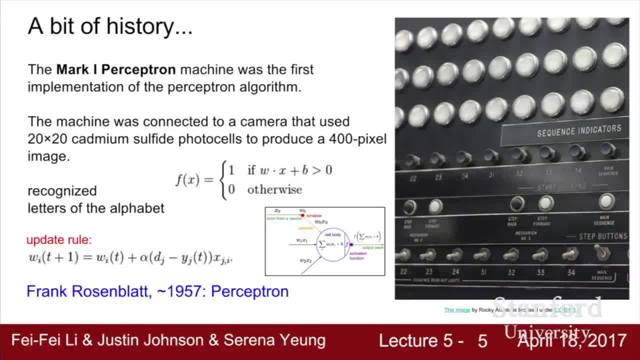 So we can go all the way back to 1957 with Frank Rosenblatt, who developed the Mark 1 Perceptron machine, which was the first implementation of an algorithm called the Perceptron, which has sort of a similar idea of getting score functions. 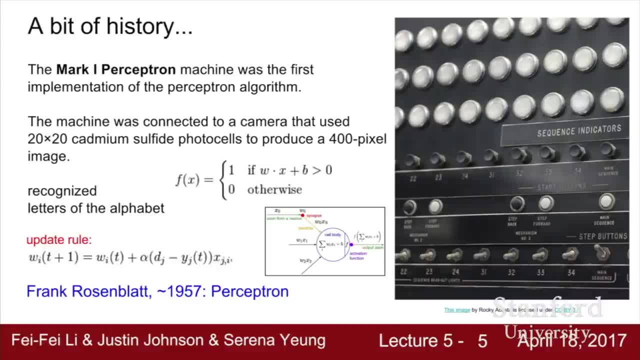 right, Using some, you know w times, x plus a bias, But here the outputs are going to be either one or a zero, And then, in this case, we have an update rule, So an update rule for our weights w, which also look kind of similar to the type 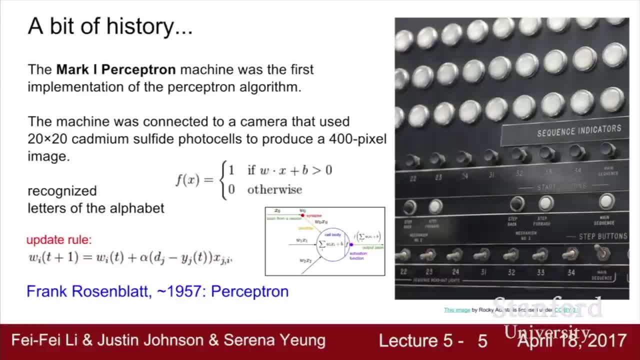 of update rule that we're also seeing in back prop. But in case in this case there was no principled back propagation technique yet, We just sort of took the weights and adjusted them in in the direction towards the target that we wanted. 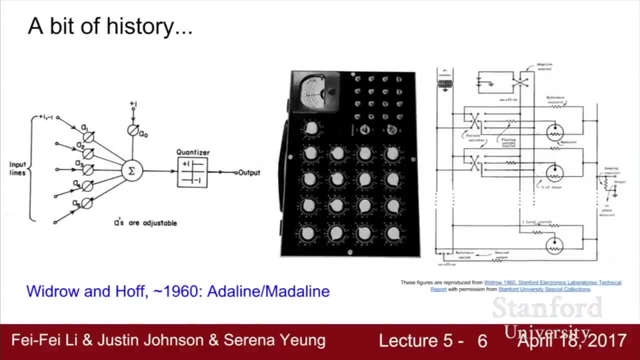 So in 1960 we had Woodrow and Hoff, who developed Adeline and Madelaine, which was the first time that we were able to get to start to stack these, these linear layers, into multilayer perceptron networks. And so, you know, this is starting to now look kind of like this idea of 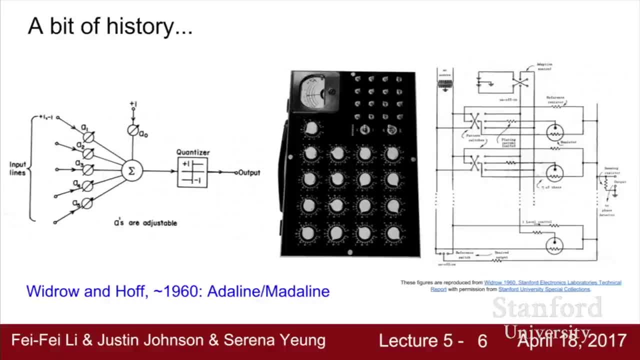 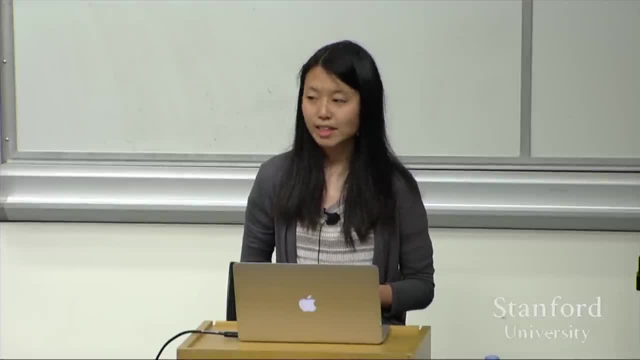 of neural network layers, But we still didn't have back prop or any sort of principled way to train this, And so the first time back prop was really introduced was in 1986 with Rommelhart. And so here we can start seeing, you know, these kinds of equations with the chain. 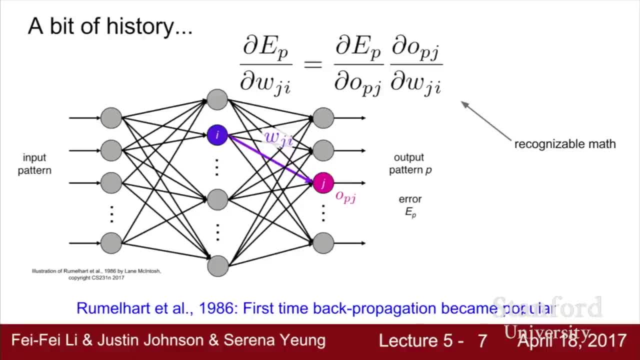 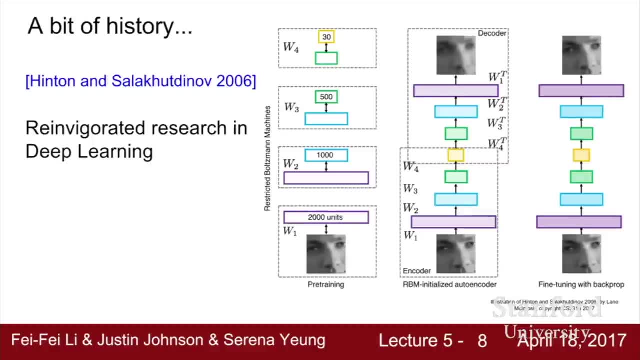 rule and the update rules that that we're starting to get familiar with Right, And so this is the first time we we started to have a principled way to train these kinds of network architectures, And so after that, you know, there still wasn't able to scale to very large neural 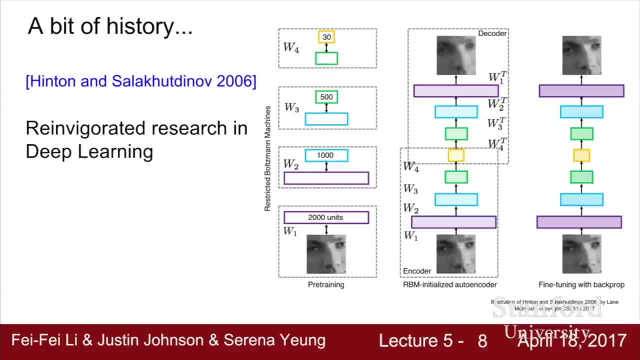 networks, and so there was, there was sort of a period in which there wasn't a whole lot of Of new things happening here or or a lot of popular use of these kinds of networks, And so this really started being reinvigorated around the 2000s. 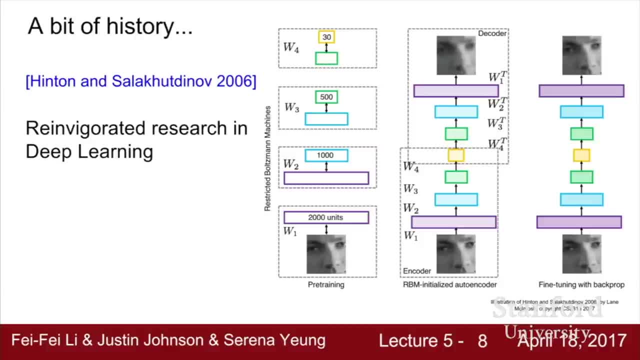 So in 2006,, there was this paper by Jeff Hinton and Ruslan Solukhodinov, Which basically showed that we could train a deep neural network and show that we could do this effectively. But it was still not quite the sort of modern iteration of neural networks. 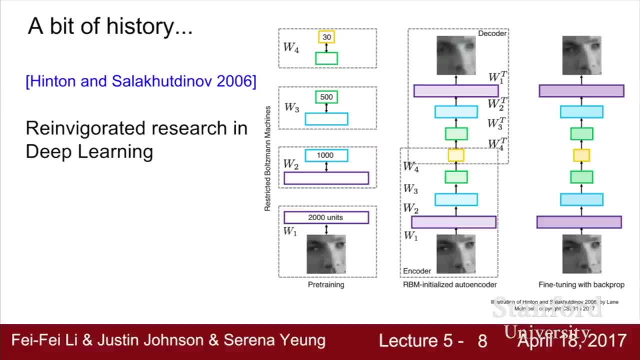 It required really careful initialization in order to be able to do back-prop, And so what they had here was they would have this first pre-training stage where you model each hidden layer through this kind of through a restricted bolt Boltzmann machine. 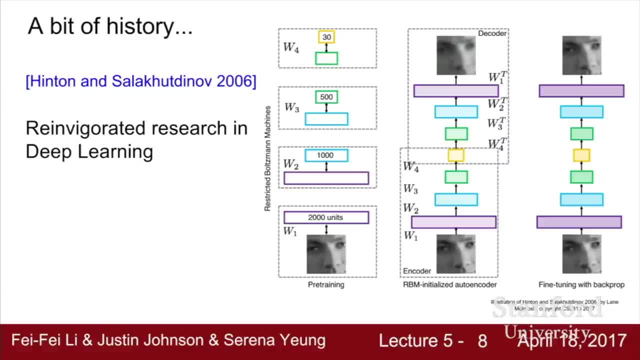 And so you're going to get some initialized weights by training each of these layers iteratively, And so once you get all of these hidden layers, you then use that to initialize your, your, you know, your- full neural network And then from there, you, you do back-prop and fine-tuning of that. 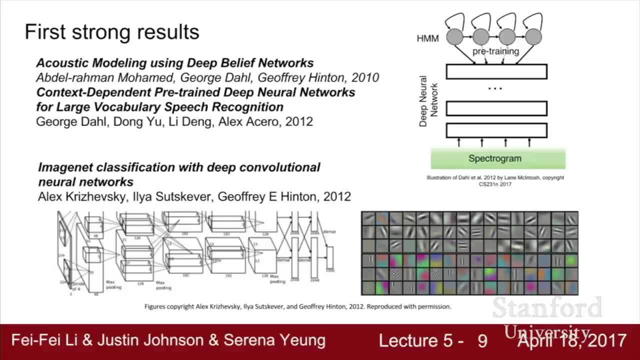 And so when we really started to get the first really strong results using neural networks and what sort of really you know sparked the whole craze of of starting to use use these kinds of networks really widely, was at around 2000,. 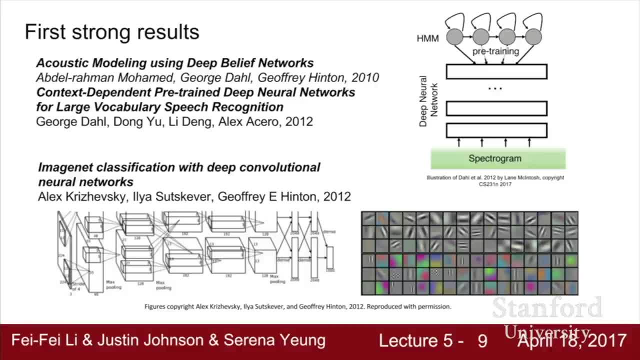 2012, where we had first the strongest results using for speech recognition, And so this is work out of Jeff Hinton's lab for acoustic modeling and speech recognition And then for image recognition. 2012 was the landmark paper from Alex Krzyzewski. 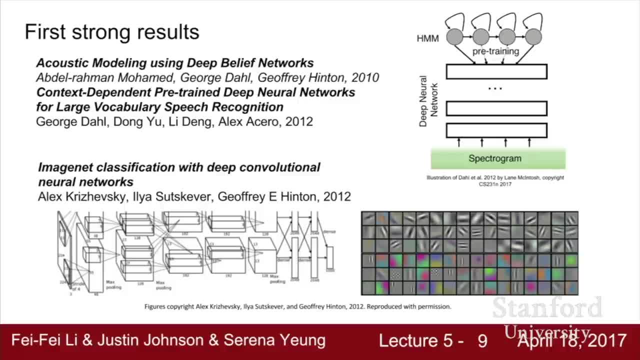 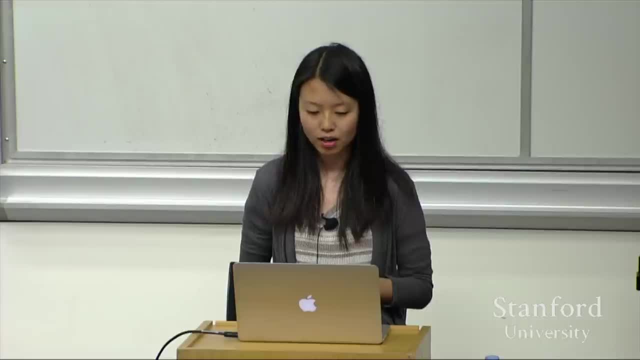 in Jeff Hinton's lab, which which introduced the first convolutional neural network architecture that was able to do get really strong results on ImageNet classification, And so it took the ImageNet image classification benchmark and was able to dramatically reduce the error on on that benchmark. 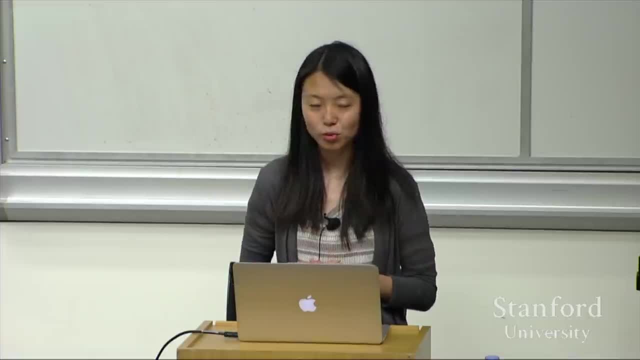 And so since then, you know, ComNets have been have gotten really wide, Widely used in all kinds of applications. So now let's step back and take a little a look at at what gave rise to com, convolutional neural networks specifically. 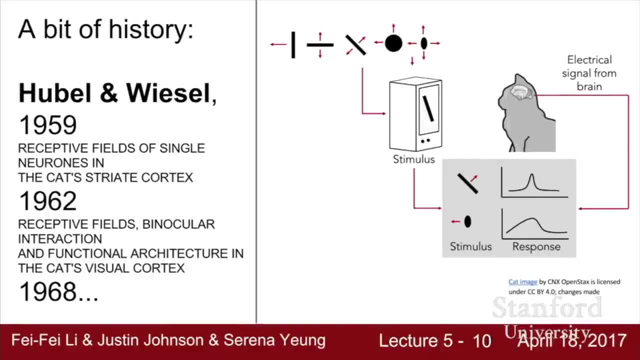 And so we can go back to the 1950s, where Hubel and Wiesel did a series of experiments trying to understand how how neurons in the visual cortex worked, And they they studied this specifically for cats, And so we talked a little bit about this in lecture one. 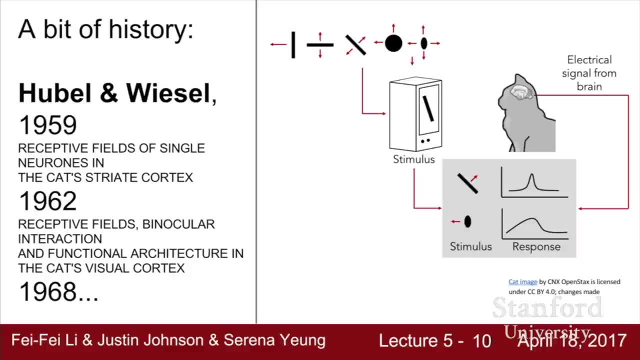 But basically in these experiments they put electrodes in the cat, into the cat brain, and they gave the cat different visual stimulus right, And so things like you know, different kinds of edges, oriented edges, different sorts of shapes, and they measured the response of the neurons. 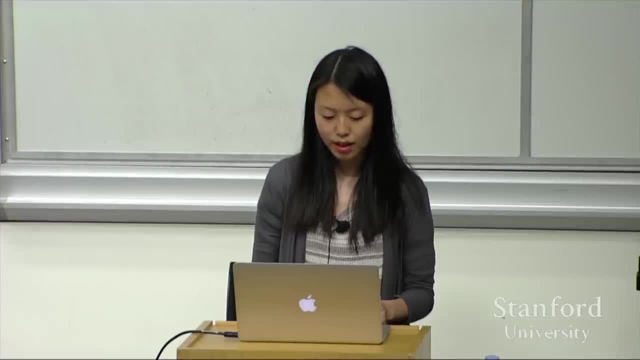 to this, these stimuli, And so there are a couple of important conclusions that they were able to make and observations, And so the first thing they found that you know, there's sort of this topographical mapping in the cortex, So Nearby. 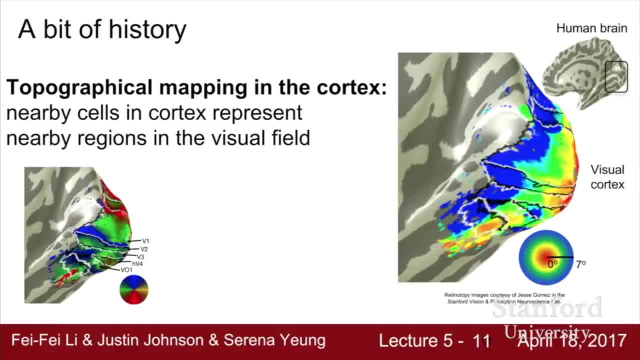 Nearby cells in the cortex also represent nearby regions in the visual field And so you can see, for example on the right here, where, if you take kind of the spatial mapping and and and map this onto a visual cortex, there's more peripheral regions. are these blue areas you know, farther away from the center? 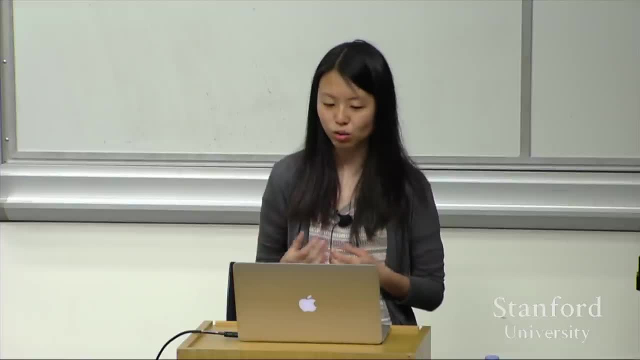 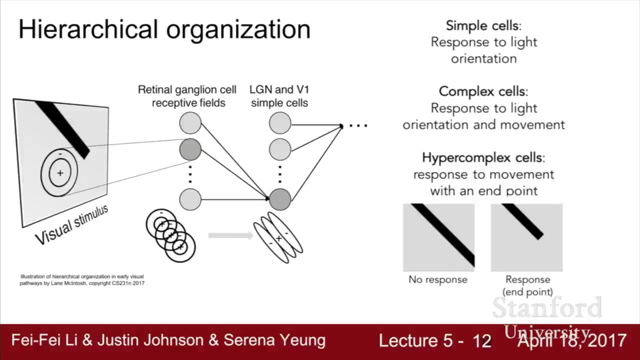 And so they also discovered that these neurons had a hierarchical orgs organization. And so if we look at different types of visual, visual stimuli, they were able to find that at the earliest layers, retinal ganglion cells were responsive to things that looked kind of like. 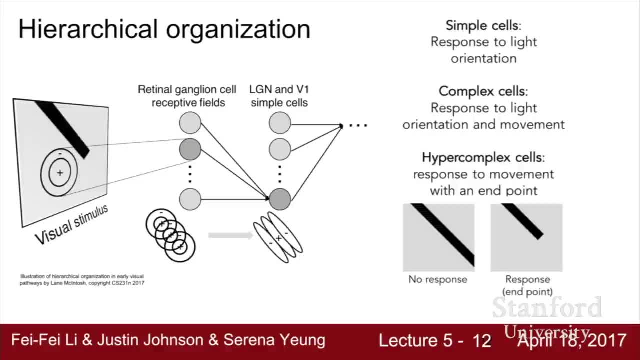 circular regions of spots, And then on top of that there are simple cells, and these simple cells are responsive to oriented edges, so different orientation of the light stimulus. And then, going further, they discovered that these were then connected to more complex cells. 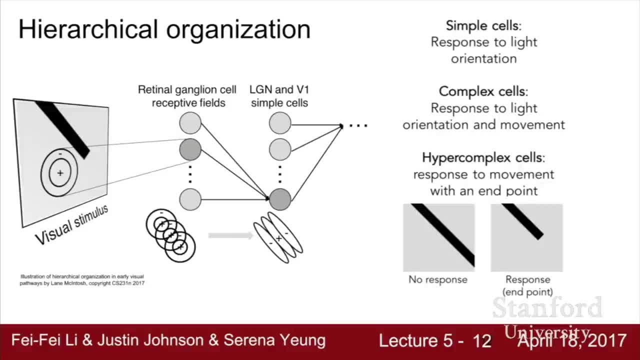 which were responsive to both light orientation as well as movement And so on. and you get increasing complexity. For example, hypercomplex cells are now responsive to movement with kind of an end point right, And so now you're starting to get the idea of corners. 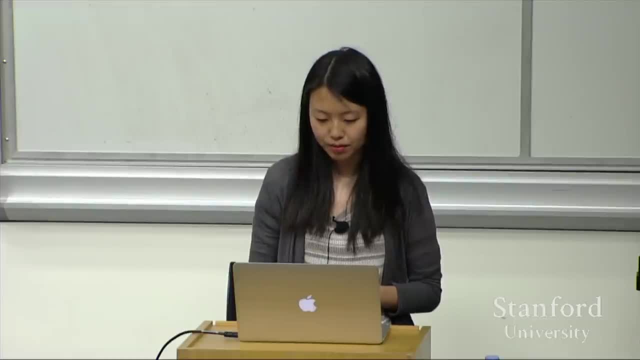 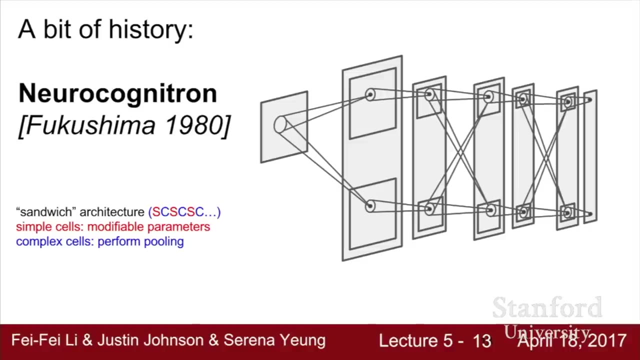 and then blobs and so on. And so then, in 1980, the neocognitron was the first example of a network architecture, a model that had this idea of, you know, simple and complex cells that Hubel and Wiesel had discovered. 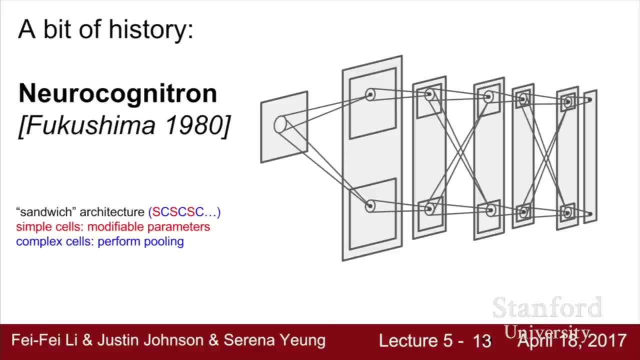 And in this case Fukushima, put these into these alternating layers of simple and complex cells, where you had these simple cells that had modifiable parameters and then complex cells on top of these that performed this sort of pooling, so that it was invariant to you know. 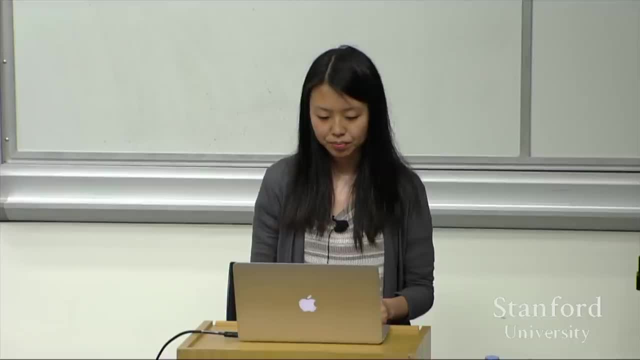 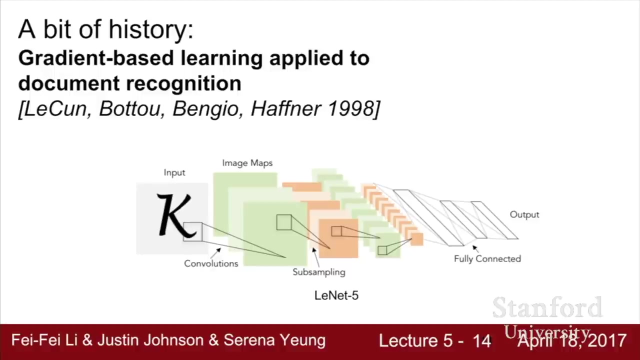 different minor modifications from the simple cells, And so this is work that was in the 1980s right, And so by 1998, Yann LeCun basically showed the first example of applying backpropagation and gradient-based learning to train convolutional neural networks. 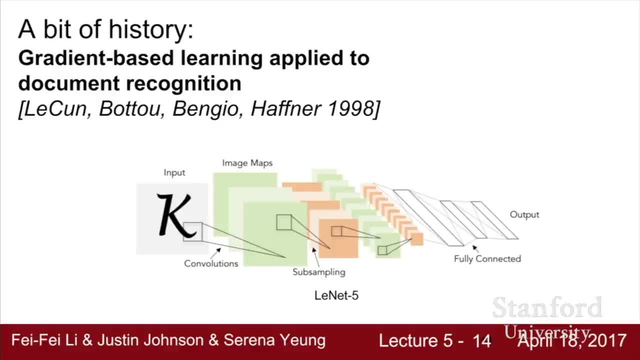 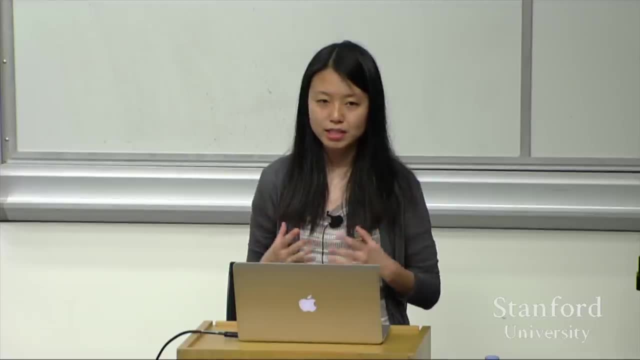 that did really well on document recognition And specifically they were able to do a good job of recognizing digits of zip codes, And so these were then used, you know, pretty widely for zip code recognition in the postal service. But beyond that it wasn't able to scale yet to more, you know. 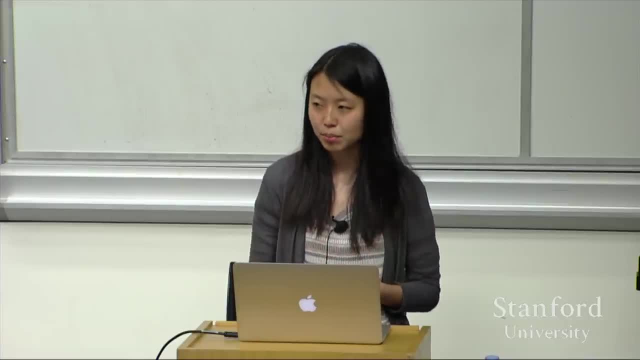 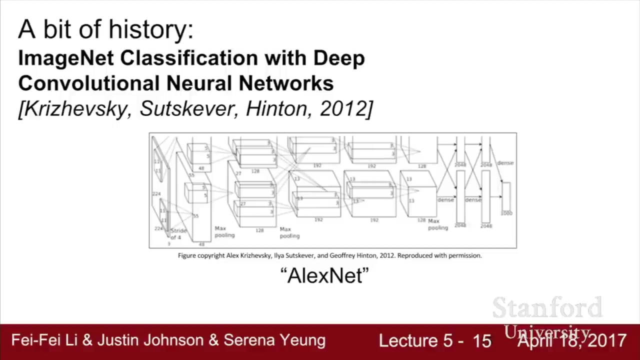 challenging and complex data. right Digits are still fairly simple and a limited set to recognize, And so this is where Alex Krashevsky, in 2012, gave the modern incarnation of convolutional neural networks And his network we sort of colloquially call AlexNet. 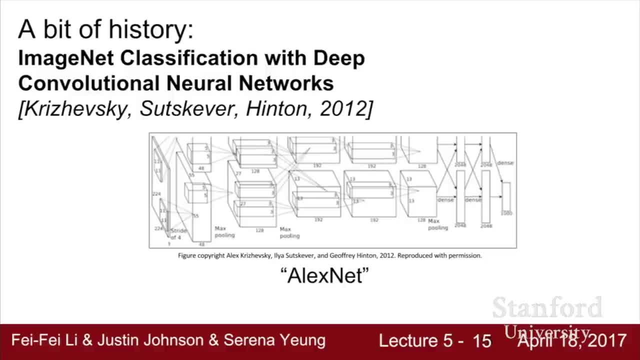 But this network really didn't look so much different than the convolutional neural networks that Yann LeCun was dealing with. They're now, you know, they were scaled now to be larger and deeper and able to. the most important parts were that they were now able to take advantage. 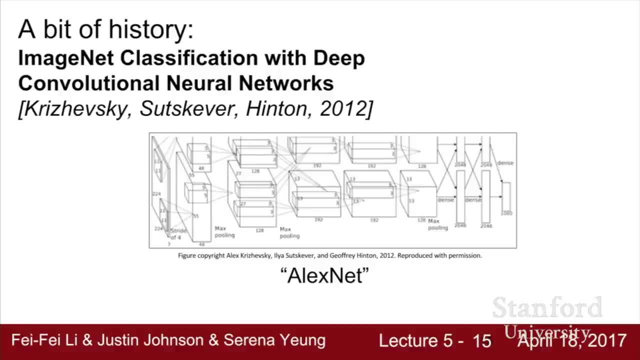 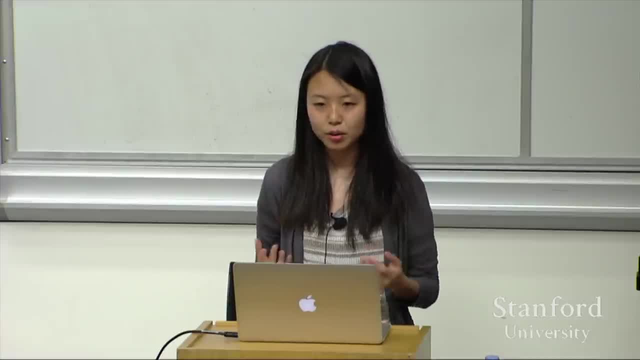 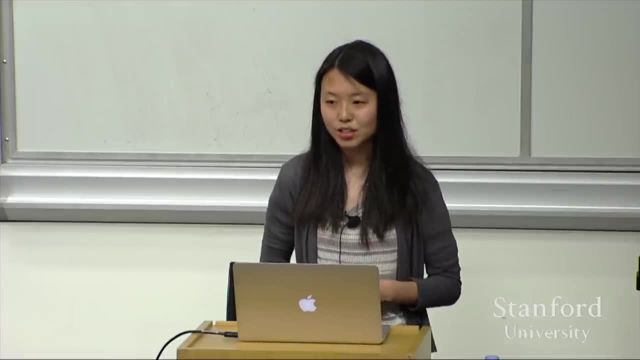 of the large amount of data that's now available, you know, in web images, in the ImageNet data set, as well as take advantage of the parallel computing power in GPUs, And so we'll talk more about that later, But fast-forwarding today, so now you know. 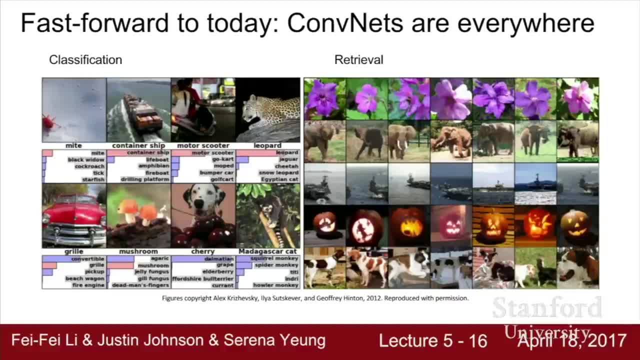 ComNets are used everywhere, And so we have the initial- you know- classification results On ImageNet from Alex Krashevsky. this is able to do a really good job of image retrieval. You can see that you know when you're trying. 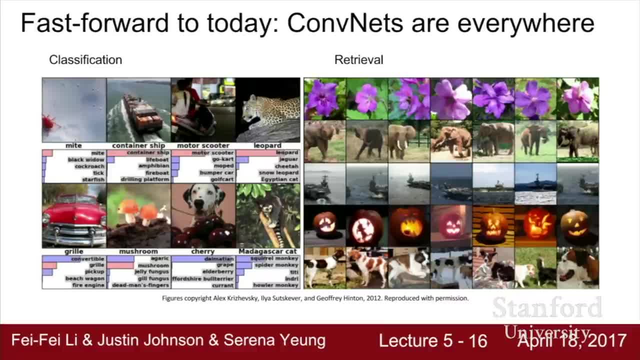 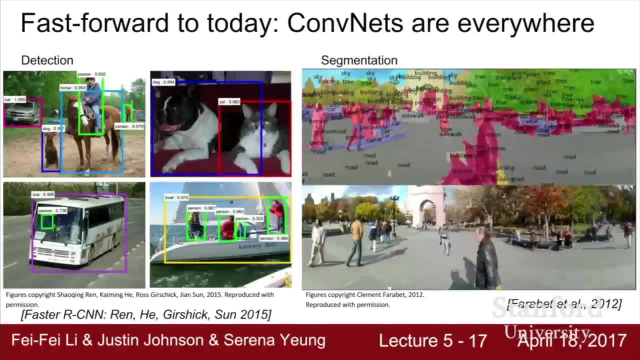 to retrieve a flower, for example. the features that are learned are really powerful for doing similarity matching. We also have ComNets that are used for detection, So we're able to do a really good job of localizing. you know where in an image is, for example. 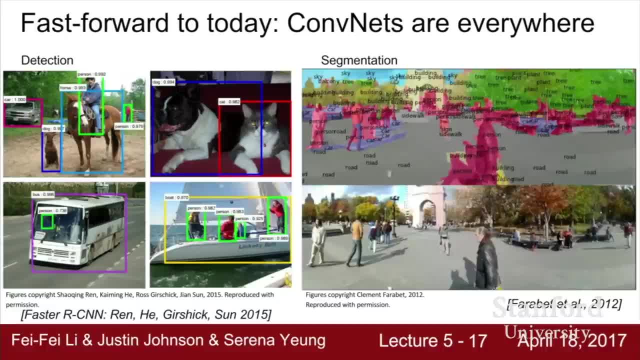 a bus or a boat and so on and draw precise bounding boxes around that We're able to go, even you know, if you want you know even deeper beyond that to do segmentation right. So these are now richer tasks where we don't. 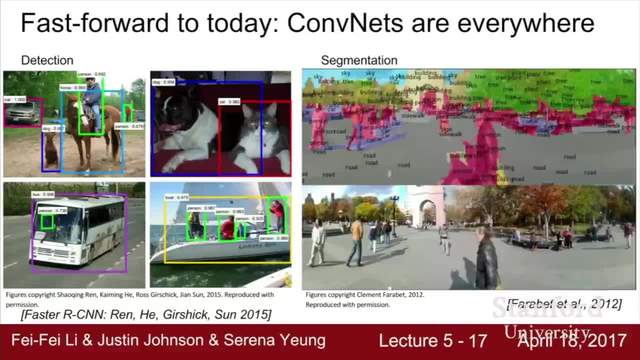 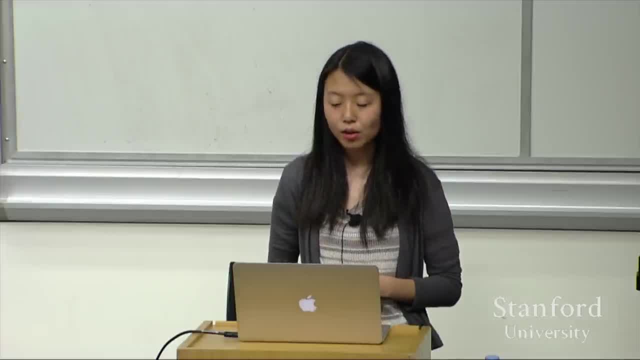 we're not looking for just the bounding box, but we're actually going to label every pixel in the outline of, you know, trees and people and so on, And these kind of algorithms are used in, you know, for example, self-driving cars. 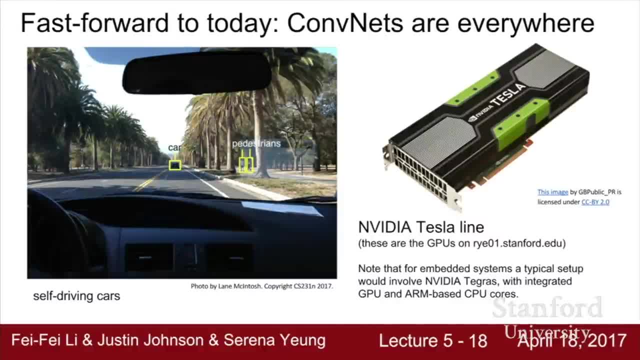 And a lot of this is powered by GPUs, as I mentioned earlier, that's able to do parallel processing and able to efficiently train and run these ComNets. And so you know, we have modern, powerful GPUs, as well as ones that you know work in embedded systems. 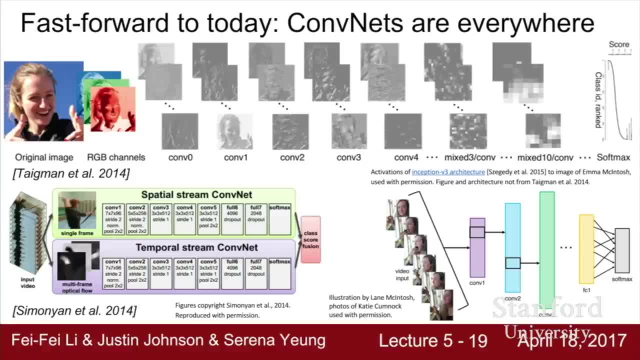 for example, that you would use in a self-driving car. So we can also look at many some of the other applications that ComNets are used for. So, face recognition right, We can put an input image of a face and get out. 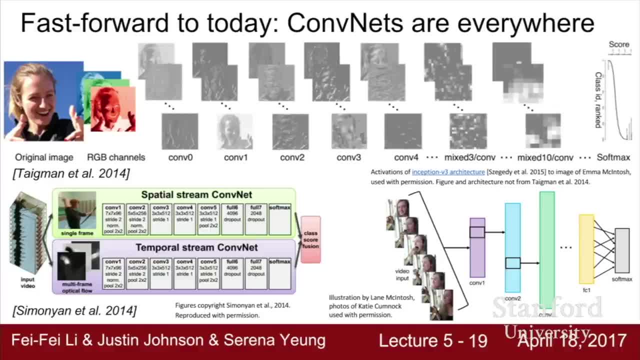 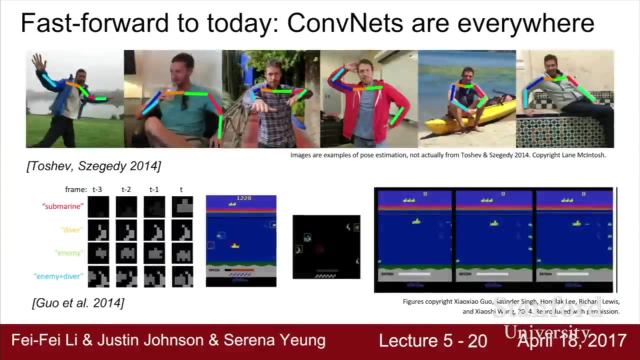 a likelihood of who this person is. ComNets are applied to video, And so this is an example of a video network that has that looks at both images as well as temporal information, And from there is able to classify videos. We're also able to do pose recognition. 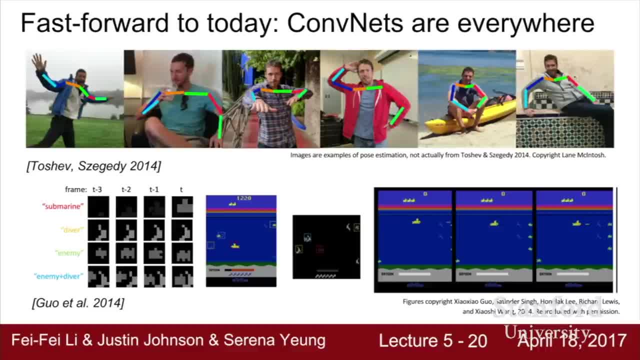 being able to recognize, you know, shoulders, elbows and different joints. And so here are some images of our fabulous TA Lane in various kinds of pretty non-standard human poses. But ComNets are able to do a pretty good job. 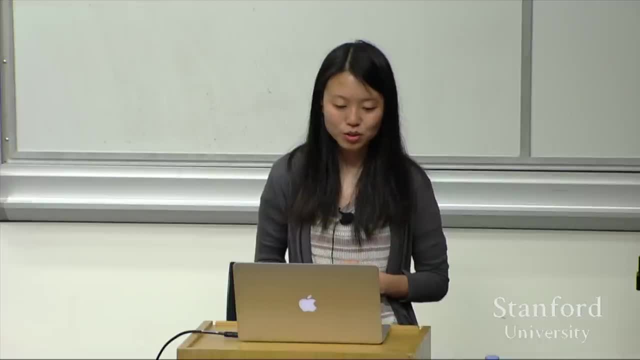 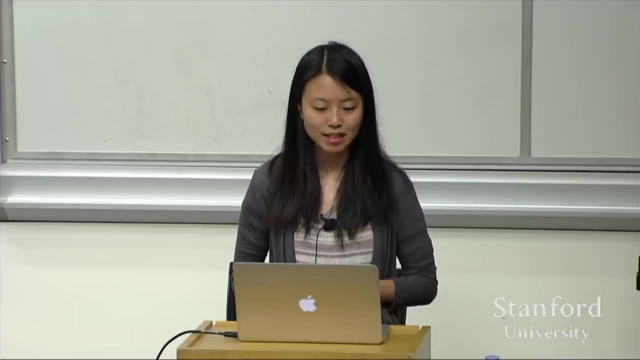 of pose recognition. these days They're also used in in game playing. So some of the work in reinforcement learning, deep reinforcement learning that you may have seen playing Atari games and Go and so on, And ComNets are an important part of all of these. 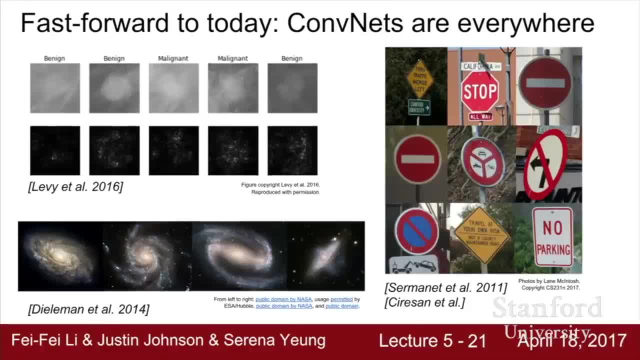 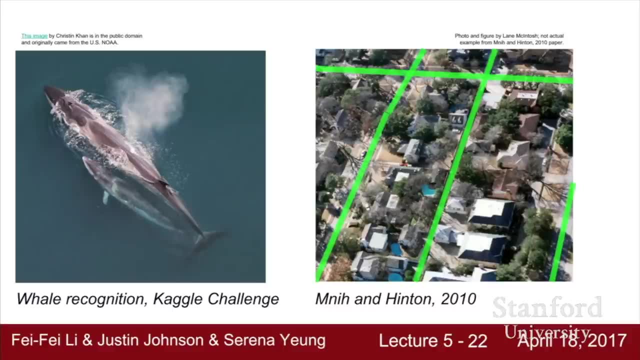 Some other applications. So they're being used for interpretation and diagnosis of medical images, for classification of galaxies, for, you know, street sign recognition. There's also whale recognition. This is from a recent Kaggle challenge. We also have examples of looking at aerial, aerial maps. 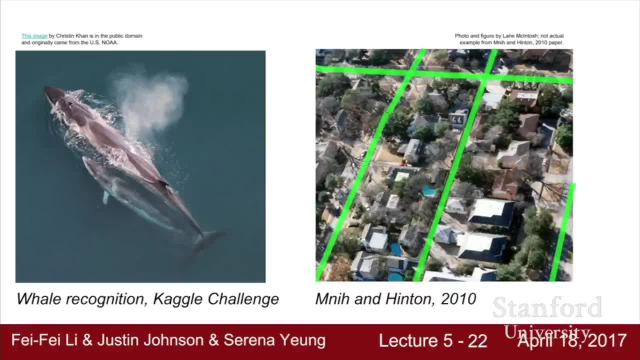 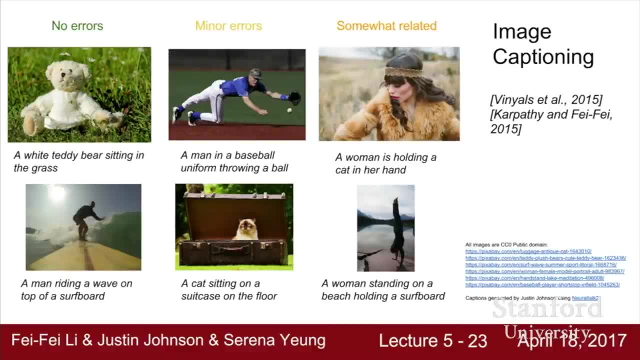 and being able to draw out where are the streets on these maps, where are buildings, and being able to segment all of these And then, beyond recognition of, you know, classification, detection, these types of tasks. we also have tasks like image captioning. 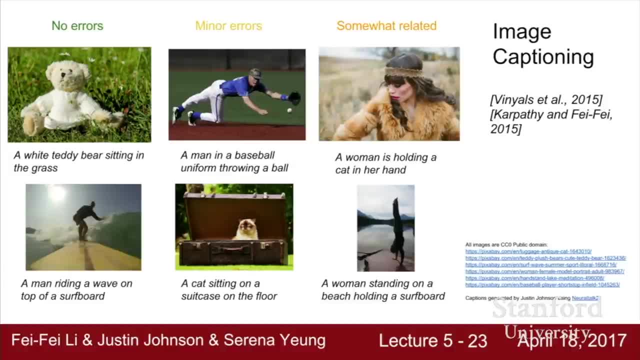 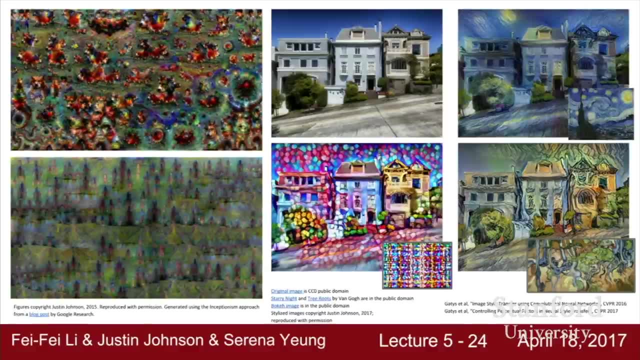 where, given an image, we want to write a sentence description about what's what's in the image, And so this is something that we'll go into a little bit more later in the class. And we also have, you know, really, really fancy. 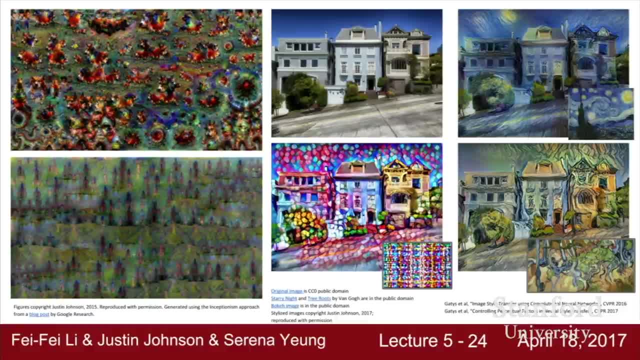 and cool kind of artwork that we can do using neural networks And so on. the left is an example of Deep Dream where we're able to take images and kind of hallucinate- you know, hallucinate different kinds of objects and concepts in the image. 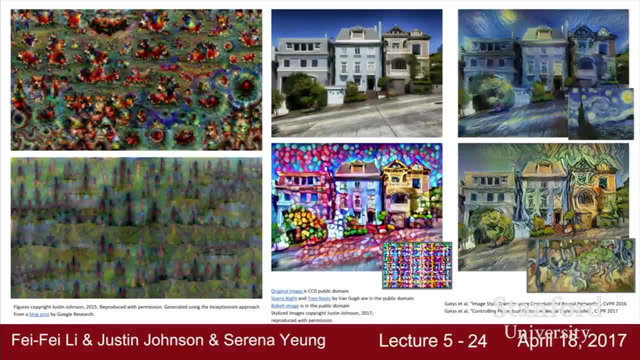 There's also neural style type work, where we take an image and we're able to- we're able to re-render this image using a, you know, a style of a particular artist and artwork, right, And so here we can take, for example, Van. Gogh. 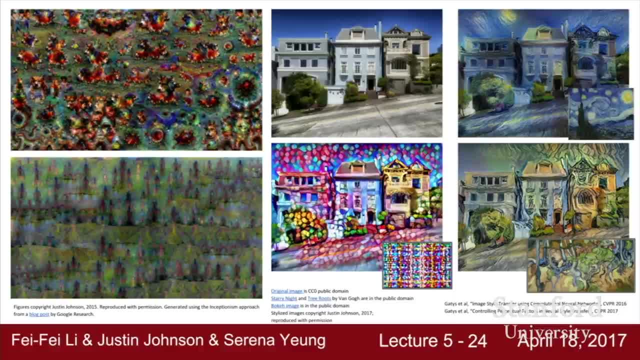 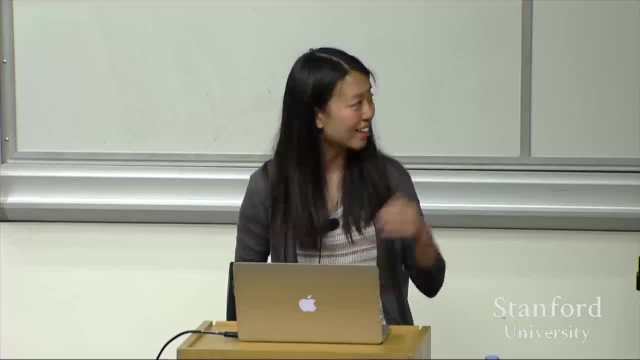 on the right Starry Night and use that to redraw our original image using that style, And Justin has done a lot of work in this and so, if you guys are interested, these are images produced by some of his code and you guys should talk to him more about it. 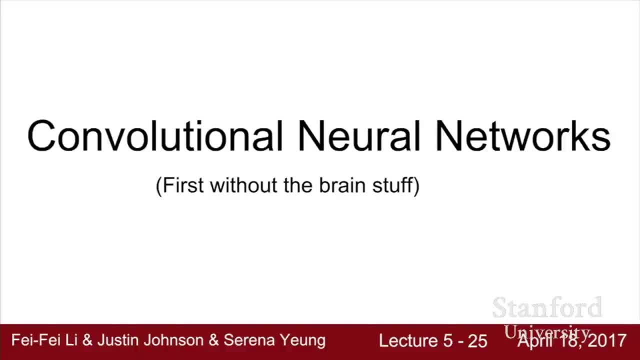 Okay. So basically, you know this is just a small sample of where Comnets are being used today, but there's really a huge amount that can be done with this right, And so you know, for your guys' projects. 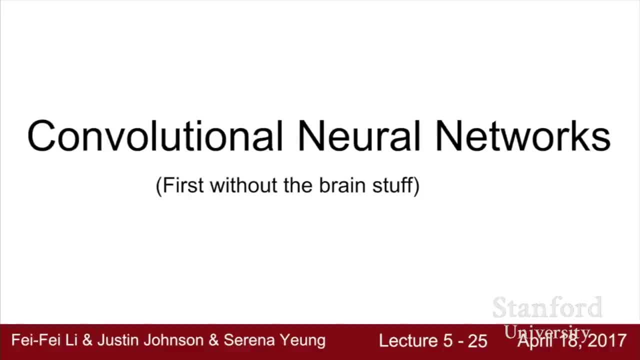 sort of you know, let your imagination go wild, and we're excited to see what sorts of applications you can come up with. So today we're gonna talk about how convolutional neural networks work. And again, the same as with neural networks. 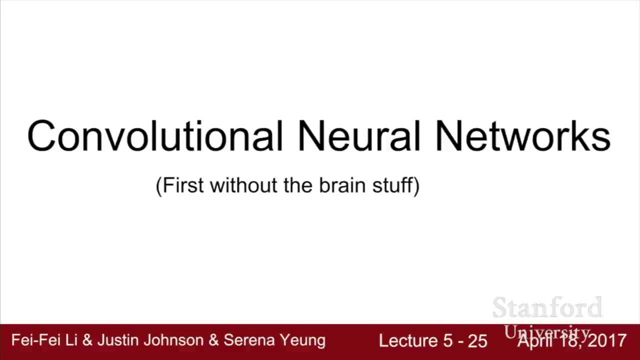 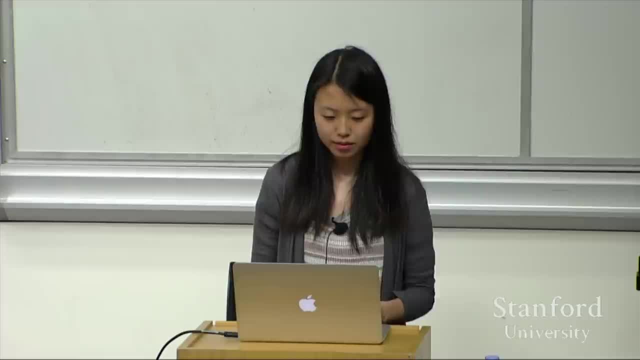 we're gonna first talk about how they work from a functional perspective, without any of the brain analogies, and then we'll talk briefly about some of these connections. Okay, so last lecture we talked about this idea of a fully connected layer. 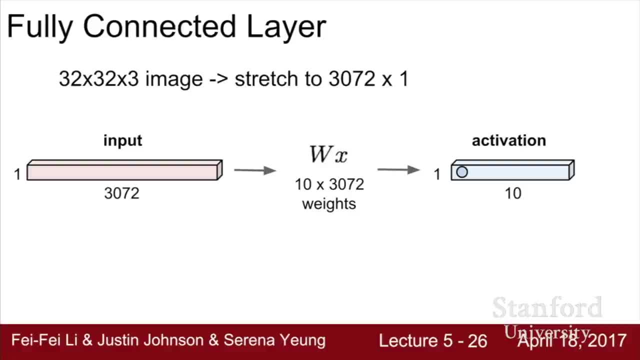 And how you know, for a fully connected layer. what we're doing is we operate on top of these vectors, right? and so let's say we have, you know, an image, a 3D image, 32 by 32 by three. so some of the images. 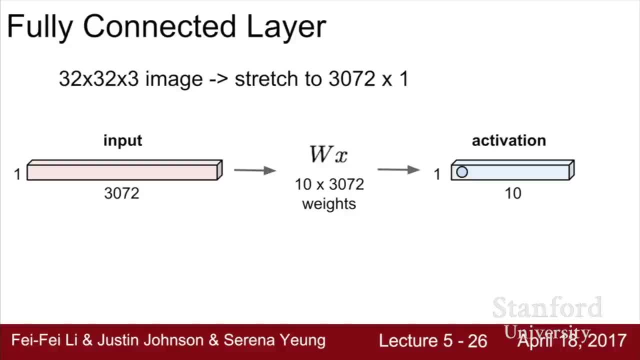 right, Some of the images that we were looking at previously. We'll take that. we'll stretch all the pixels out right, And then we have this 3,072 dimensional vector, for example, in this case, And then we have these weights, right. 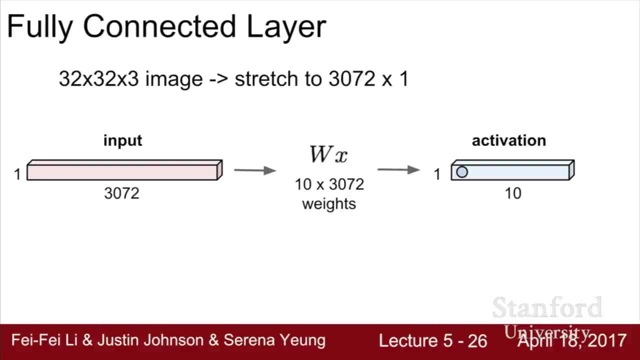 So we're gonna multiply this by a weight matrix, And so here, for example, our W, we're gonna say, is 10 by 3,072.. And then we're going to get the activations, the output of this layer, right. 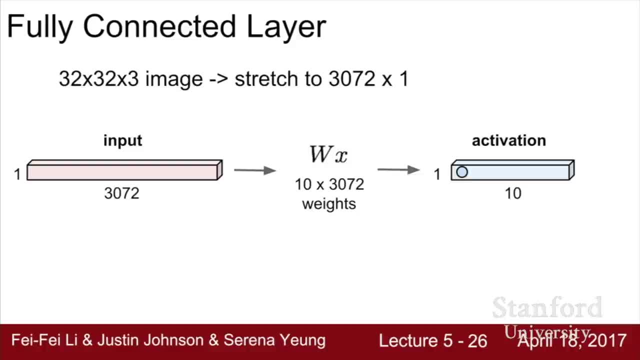 And so, in this case, we take each of the each of our 10, right, And so, in this case, we take each of the each of our 10, 10 rows, and we do this dot product with the 3,072 dimensional input. 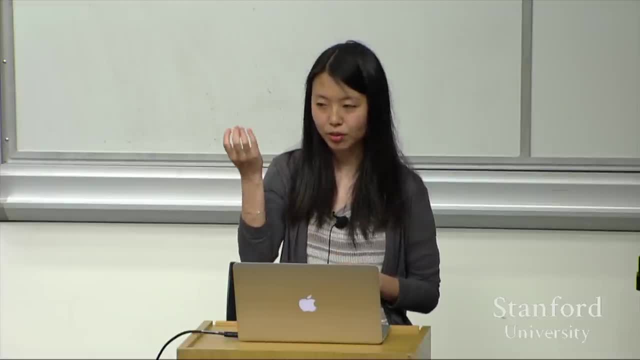 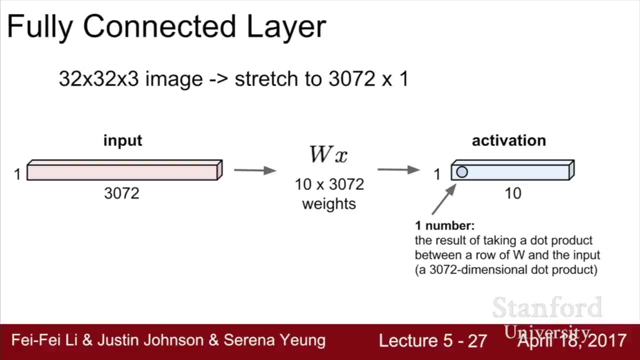 And from there we get this one number, That's, that's kind of the, the value of that neuron, And so in this case we're going to have 10 of these, these neuron outputs, And so a convolutional layer. so the main, main difference between this and 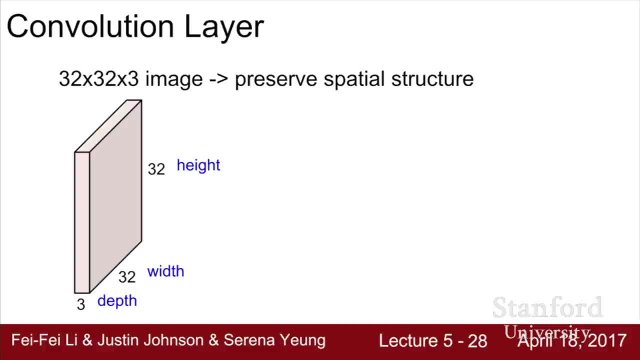 the fully connected layer that we've been talking about is that here we want to preserve spatial structure And so taking this 32 by 3, this cornice 32 by 32 by 3 image that we had earlier, instead of stretching this all out into one long vector. 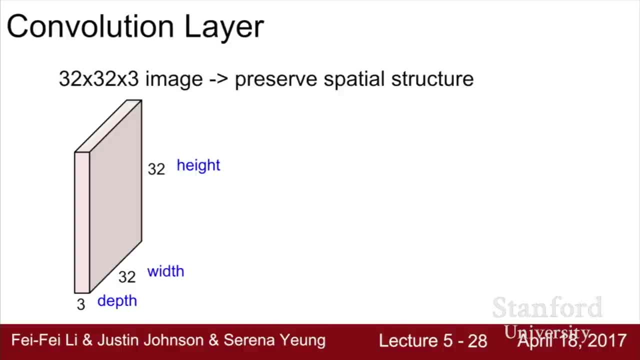 we are now going to keep the structure of this image right, This three-dimensional input, And then what we're going to do is our weights are gonna be these small filters, So in this case, for example, a 5 by 5 by 3 filter, and 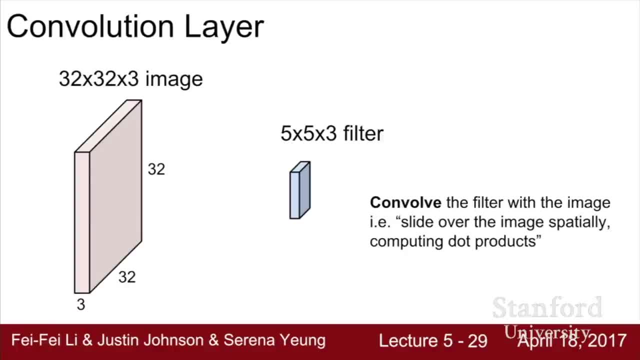 we're going to take this filter and we're going to slide it over the image spatially And and compute dot products at every spatial location, And so we're we're going to go into detail of how exactly this works, And so we're going to go into detail of how exactly this works. 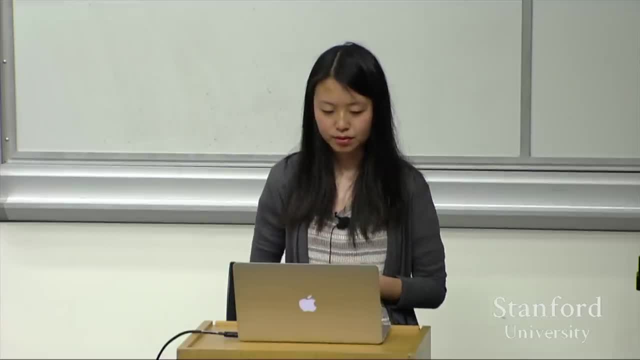 Again, thisましょう will name these five by five dot products. And, as I said, what we're doing here, we're bubbling it up. every space must be So. our filters, first of all, always extend the full depth of the input volume. 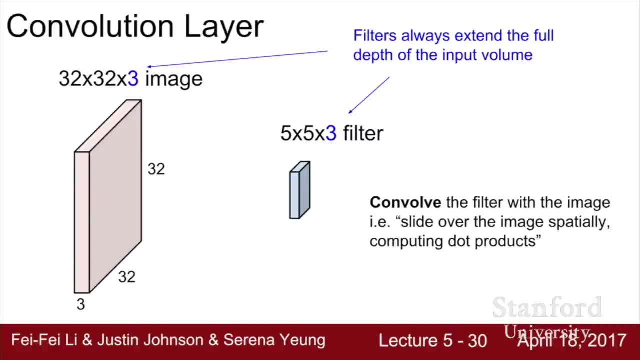 And so they're going to be just a smaller spatial area. so, in this case, five by five, right, instead of our full 32 by 32 spatial input. But they're always gonna go through the full depth. So here we're going to take five by five, by three. 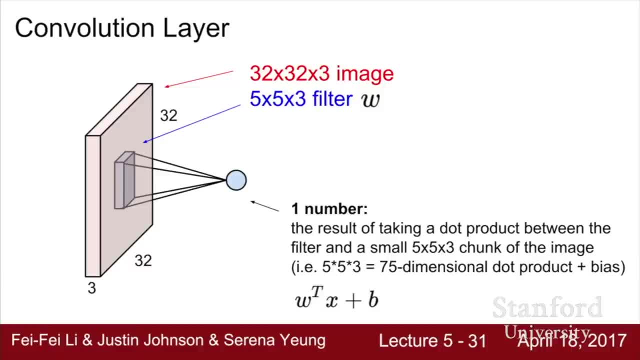 And then we're going to take this filter and again we're gonna take this filter and at a given spatial location we're going to do a dot product between this filter and then a chunk of the image. So we're just going to overlay this filter. 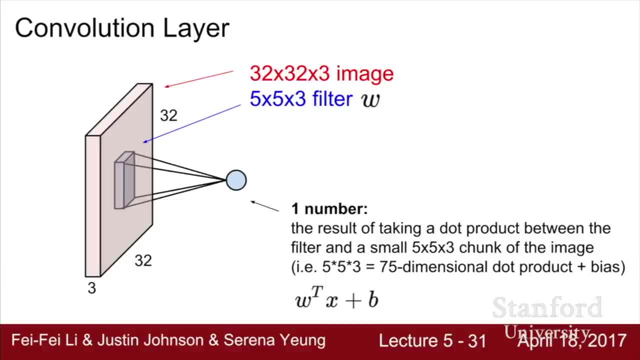 on top of a spatial location in the image right, and then do the dot product, the multiplication of each element of that filter with each corresponding element in that spatial location that we've just plopped it on top of, And then this is going to give us a dot product. 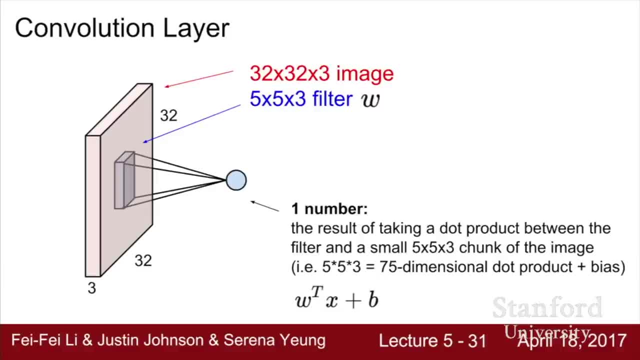 So in this case we have five times five times three. This is the number of multiplications that we're going to do right, plus the bias term. And so this is basically taking our filter w and basically doing w, transpose times x and plus bias. 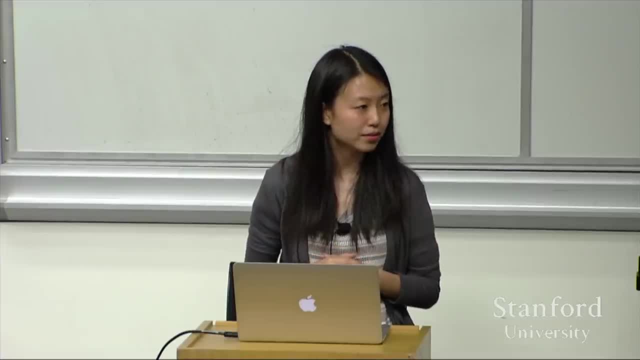 So is that clear how this works? Yeah, so the question is: when we do the dot product, do we turn the five by five by three into one vector? Yeah, and in essence that's what you're doing. You can, I mean, you can- think of it. 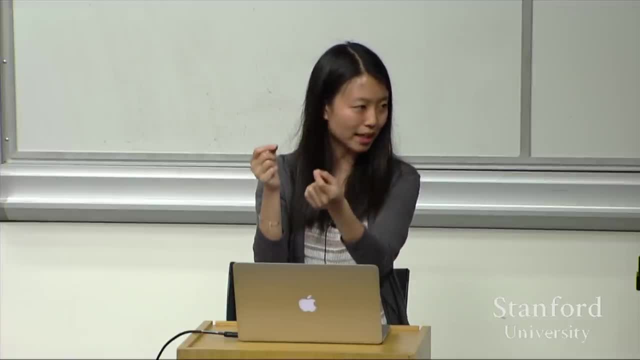 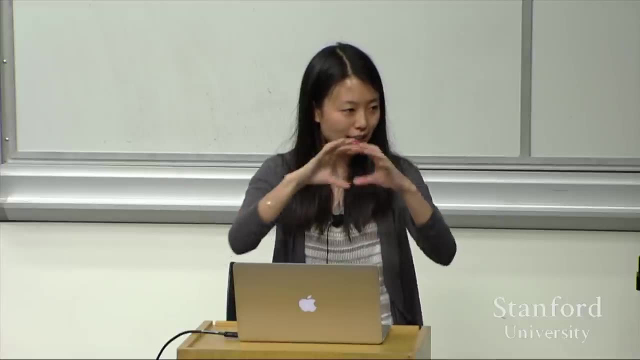 as just plopping it on and doing the element-wise multiplication at each location. but this is gonna give you the same result as if you stretched out the filter at that point, stretched out the input volume that it's laid over and then took the dot product. 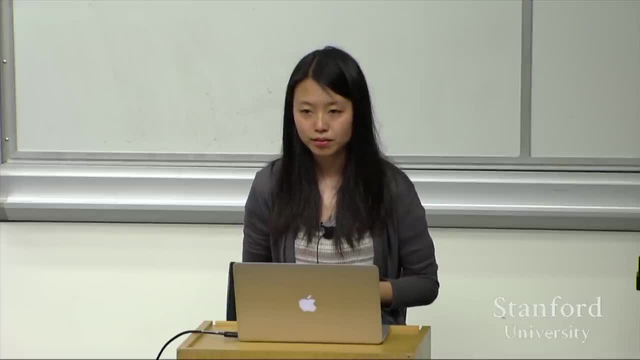 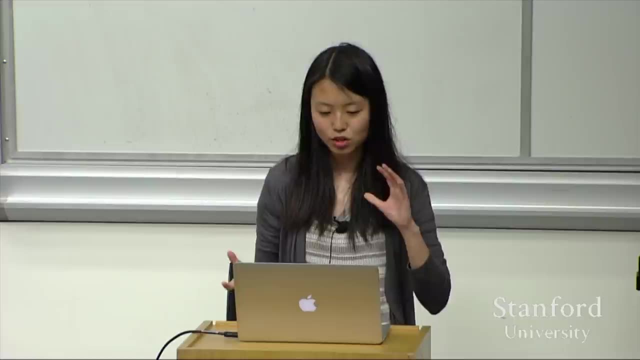 And that's what's written here. Yeah, question, Oh, this is so. the question is: any intuition for why? this is a w transpose And this is just not really. this is just the notation that we have here to make the the. 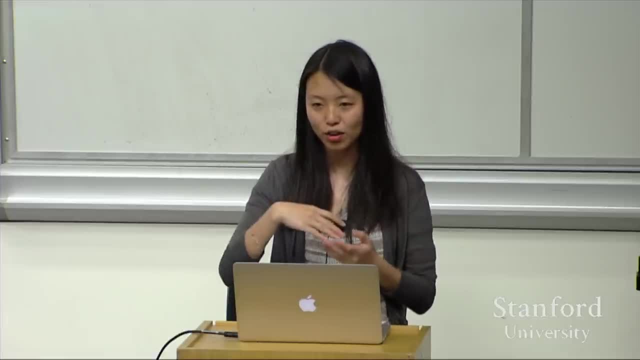 the math work out as a dot product. So it just depends on how you're representing w and whether, in this case, if we look at the w matrix, this happens to be each column, and so we're just taking the transpose to get a row out of it. 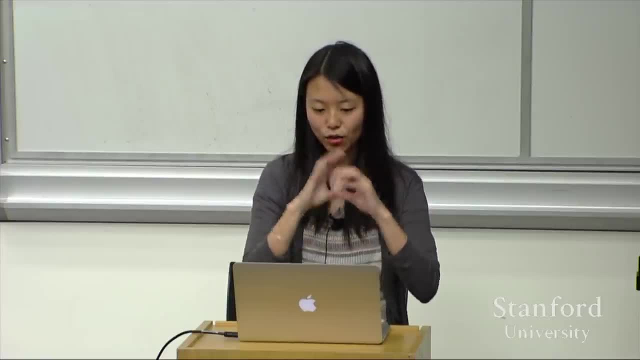 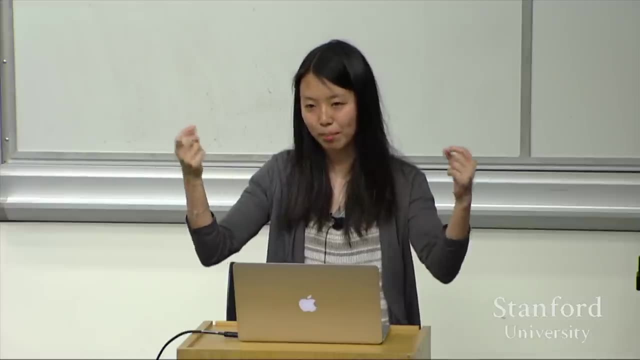 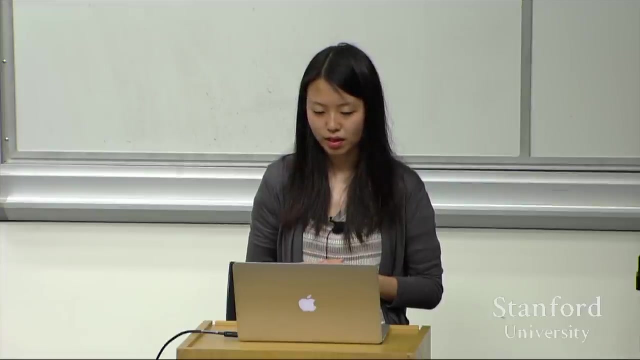 But there's no intuition here. We're just taking the filters of w and we're stretching it out into a 1D vector, And in order for it to be a dot product, it has to be like a one by n vector. Okay, so the question is: is w here, not five by five, by three? 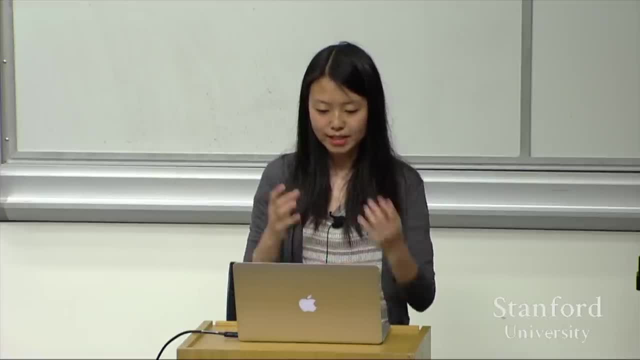 It's one by 75. So that's the case, right. If we're going to do this dot product of w transpose times x, we have to stretch it out first before we do the dot product. So we take the five by five by three. 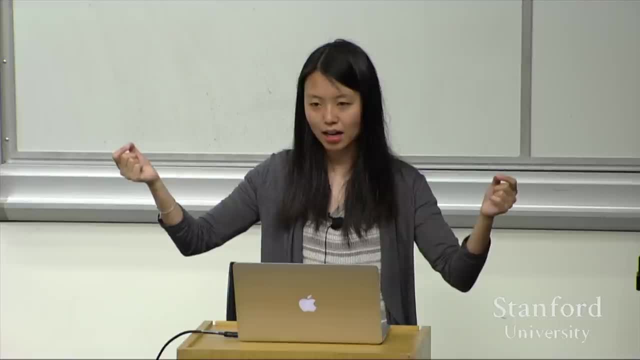 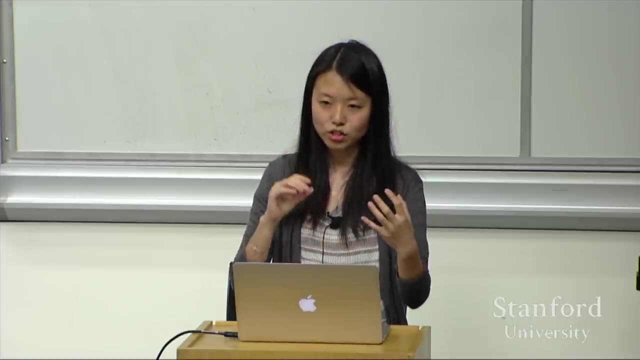 and we just take all these values and stretch it out into a long vector And so- again similar to the other question- the actual operation that we're doing here is plopping our filter on top of a spatial location in the image and multiplying. 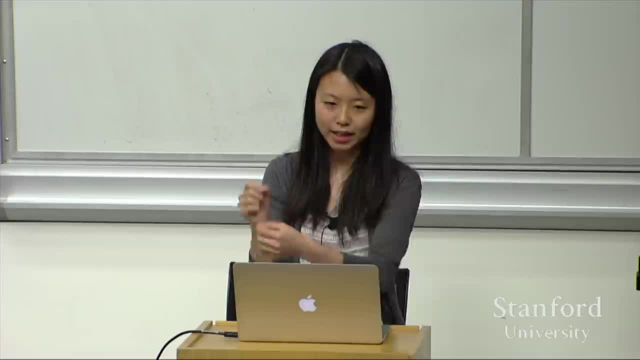 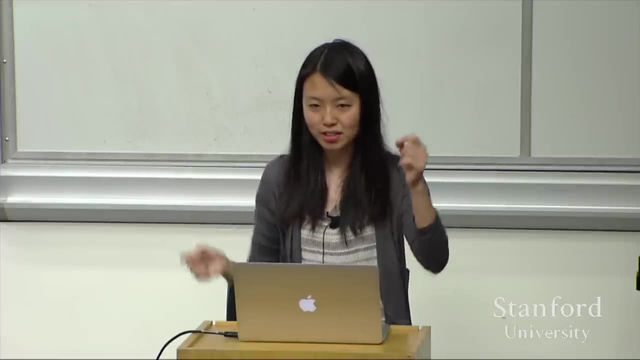 all the corresponding values together. But in order just to make it kind of an easy expression similar to what we've seen before, we can also just stretch each of these out. make sure that dimensions are transposed correctly so that it works out as a dot product. 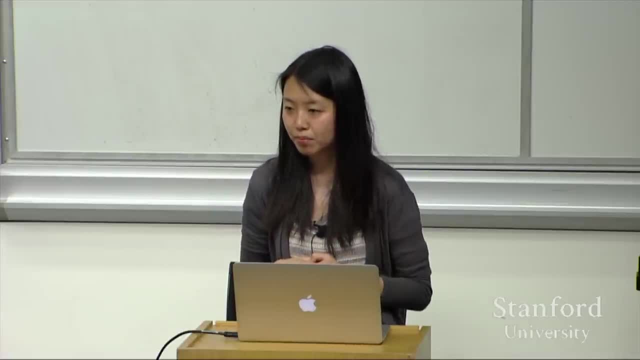 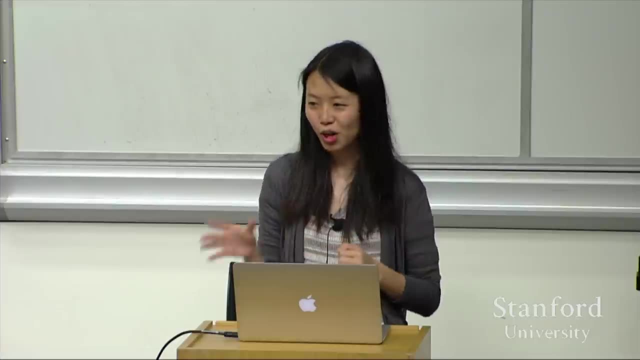 Yeah, question Okay. the question is: how do we slide the filter over the image? For the first one, we'll go into that next. Yes, Okay. so the question is: should we rotate the kernel by 180 degrees to better match the convolution? 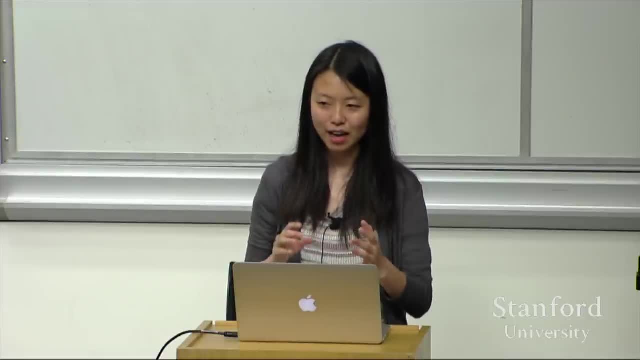 the definition of a convolution, And so the answer is that we'll also show the equation for this later, but we're using convolution as kind of a looser definition of what's happening. So for people from signal processing what we are actually technically doing, 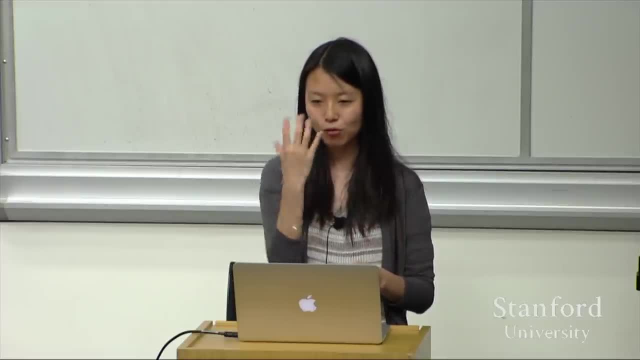 if you want to call this a convolution, is we're convolving with the flipped version of the filter, But for the most part, we just don't worry about this and we just do this operation, and it's like a convolution in spirit, Okay so, 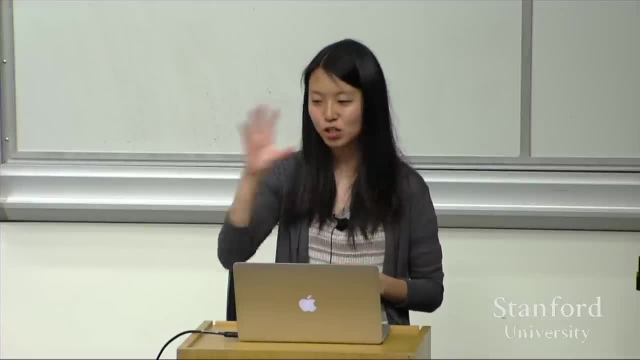 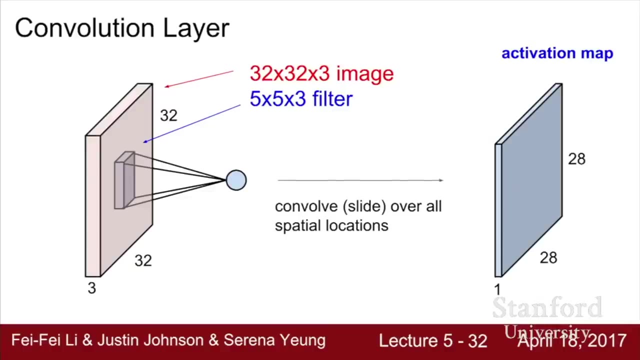 Okay. so we had a question earlier: How do we slide this over all the spatial locations? So what we're going to do is we're going to take this filter, We're going to start at the upper left-hand corner and basically center our filter on top of every pixel. 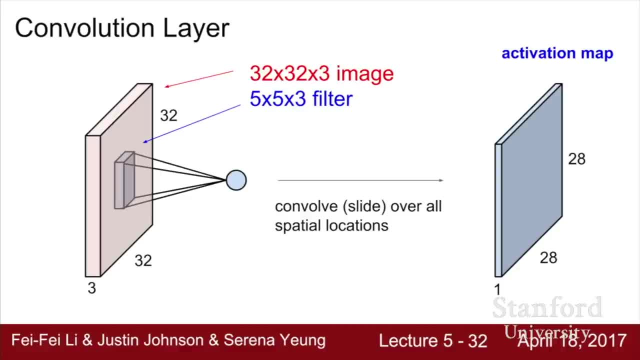 in this input volume and at every position we're going to do this dot product and this will produce one value in our output activation map, And so then we're going to just slide this around. The simplest version is just at every pixel. 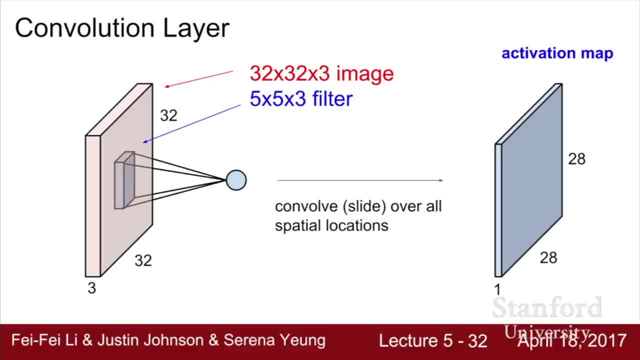 we're going to do this operation and fill in the corresponding point in our output activation. You can see here that the dimensions are not exactly what would happen. right, If you're going to do this? I had 32 by 32 in the input. 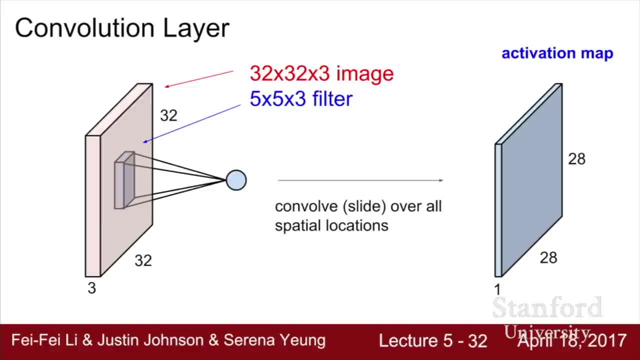 and I'm having 28 by 28 in the output, and so we'll go into examples later of the math of exactly how this is going to work out dimension-wise. but basically you have a choice of how you're going to slide this. 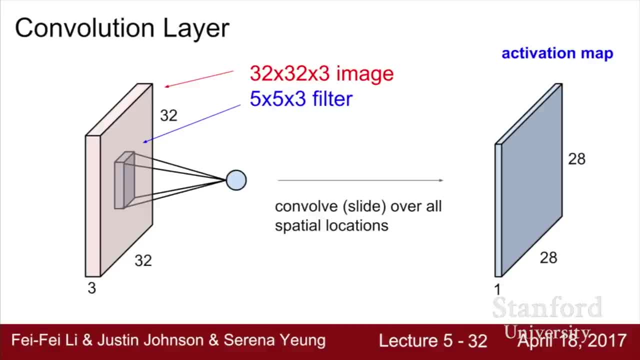 whether you go at every pixel or whether you slide. let's say, two input values over at a time, two pixels over at a time, and so you can get different sized outputs depending on how you choose to slide. But you're basically doing this operation in a grid fashion. 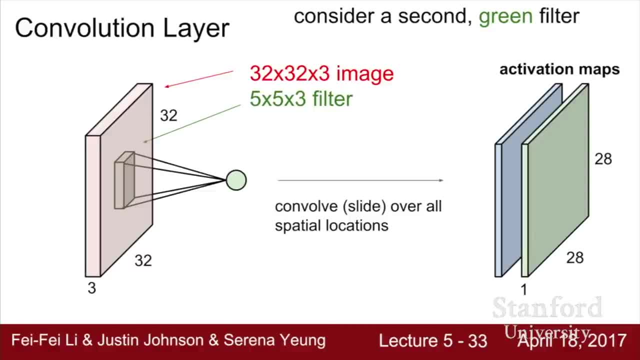 Okay, so what we just saw earlier, this is taking one filter, sliding it over all of the spatial locations in the image, and then we're going to get this activation map out right, which is the value of that filter, at every spatial location. 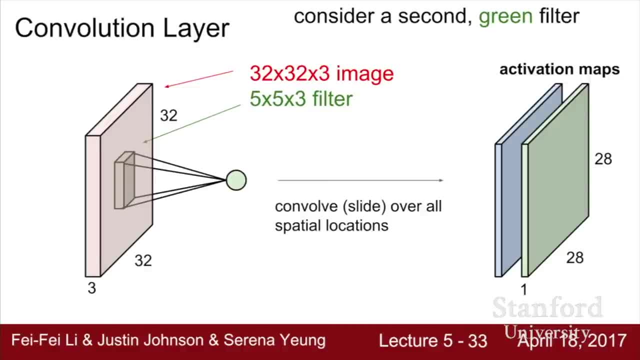 And so when we're dealing with a convolutional layer, we want to work with that with multiple filters, right, because each filter is kind of looking for a specific type of template or concept in the input volume, And so we're going to have a set of multiple filters. 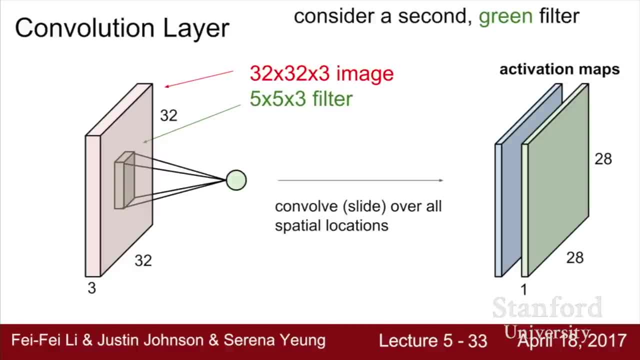 and so here I'm going to take a second filter, this green filter, which is again five by five, by three. I'm going to slide this over all of the spatial locations in my input volume, and then I'm going to get out. 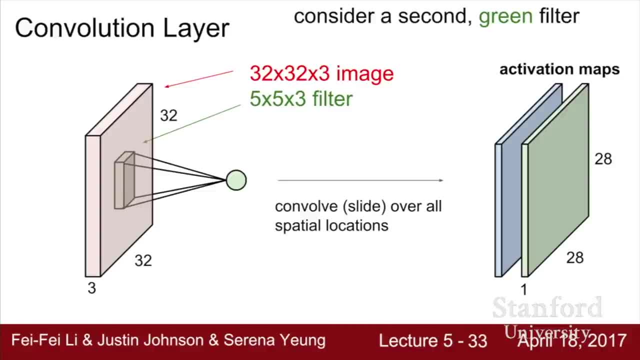 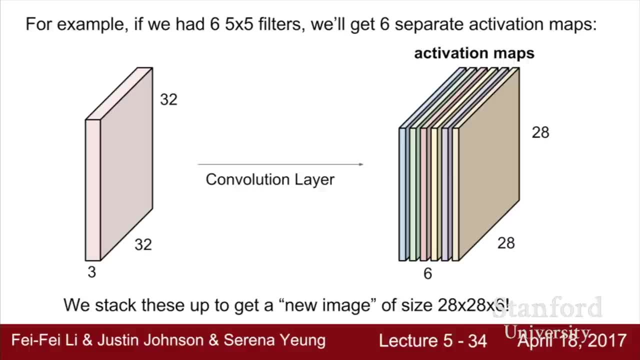 this second green activation map, also of the same size, And we can do this for as many filters as we want to have in this layer. So, for example, if we have six filters, six of these five by five filters, then we're going to get in total. 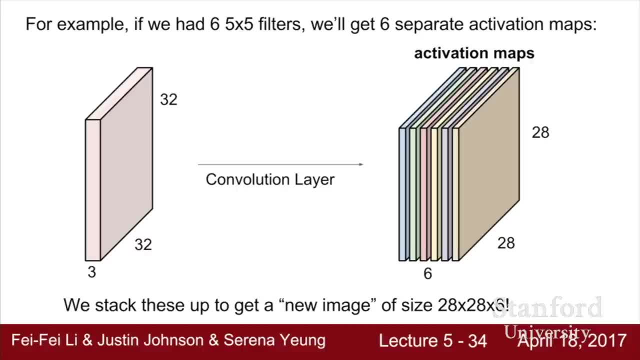 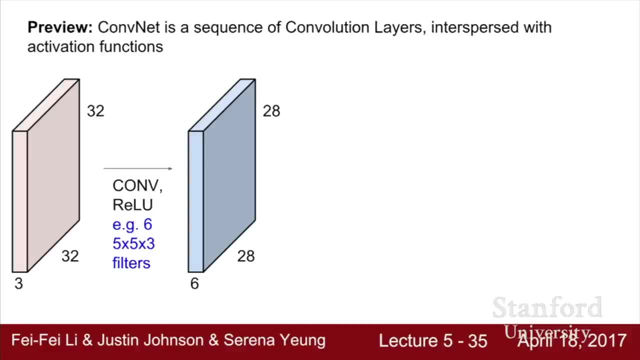 six activation maps out: All of so we're going to get this output volume. that's going to be basically six by 28, by 28.. Right, and so a preview of how we're going to use these convolutional layers in our convolutional network. 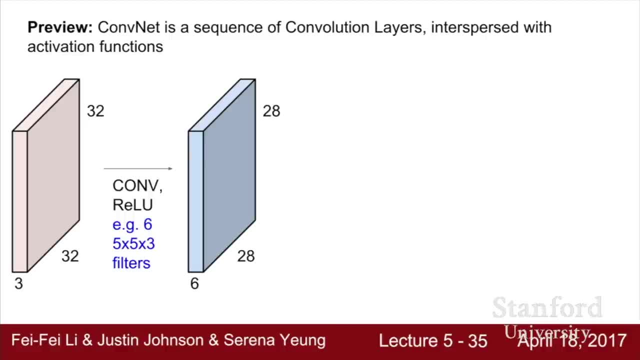 is that our ComNet is basically going to be a sequence of these convolutional layers stacked on top of each other, same way as what we had with the, you know, simple linear layers in the neural network, and then we're going to intersperse these. 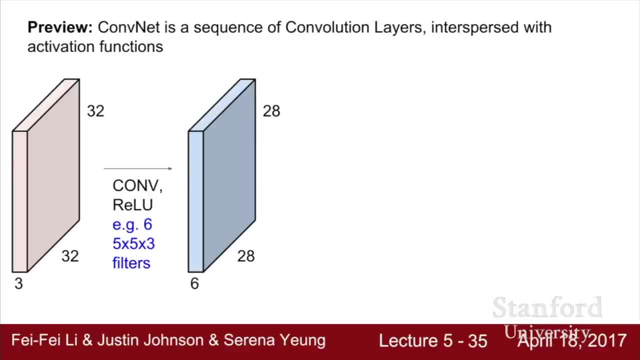 with activation functions. So, for example, a ReLU activation function, Right, and so you're going to get something like convolutional, Conv, ReLU, and usually also some pooling layers, and then you're just going to get a sequence of these, each putting 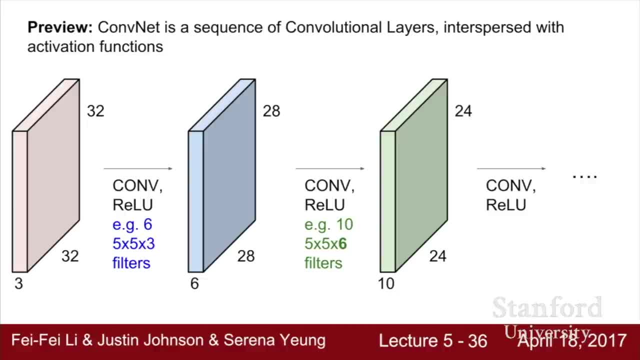 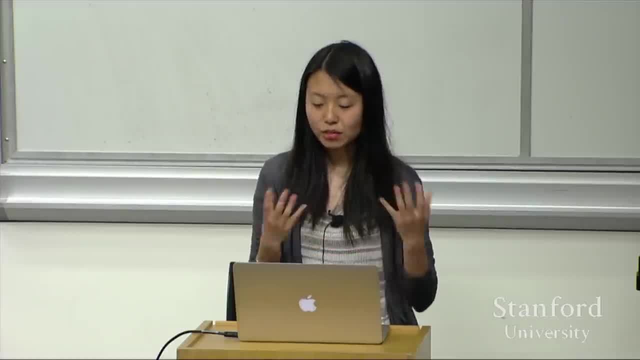 each creating an output that's now going to be the input to the next convolutional layer. Okay, and so each of these layers, as I said earlier, has multiple filters- right, many filters, and each of the filters is producing an activation map. 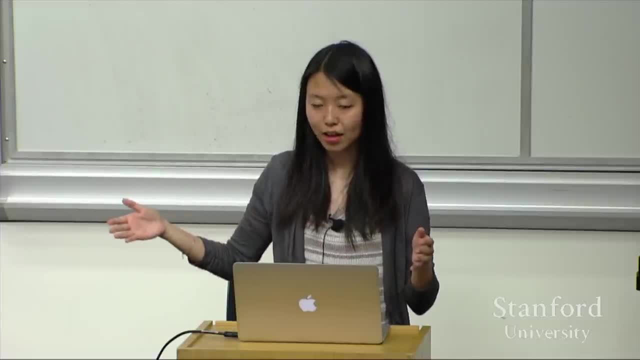 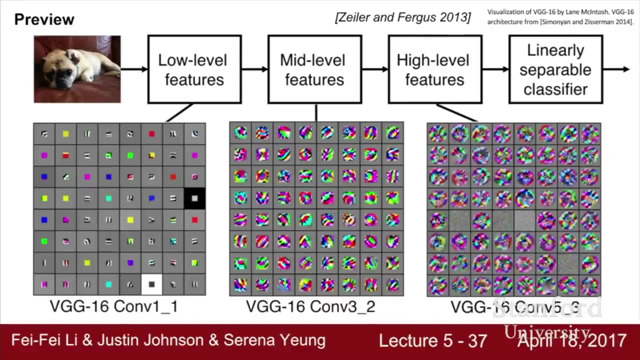 And so when you look at multiple of these layers stacked together in a ComNet, what ends up happening is you end up learning this hierarchy of filters, where the filters at the earlier layers usually represent low-level features that you're looking for. So things kind of like edges, right. 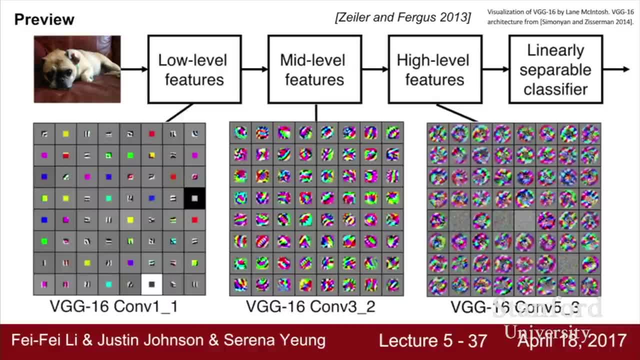 and then at the mid-level you're going to get more complex, more complex kinds of features- so maybe it's looking more for things like corners and blobs and so on- and then at higher-level features you're going to get things that are starting. 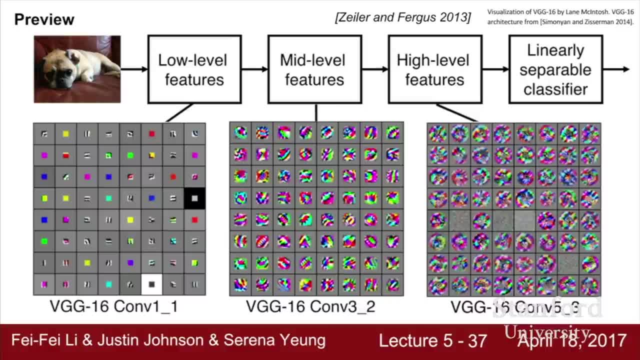 to more resemble concepts and blobs, And we'll go into more detail later in the class on how you can actually visualize all these features and try and interpret what your network, what kinds of features your network, is learning. But the important thing for now is just to understand. 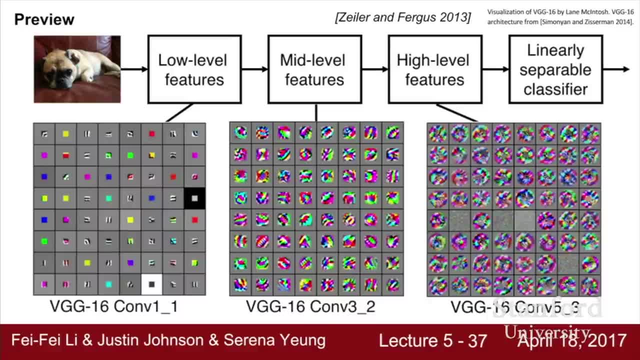 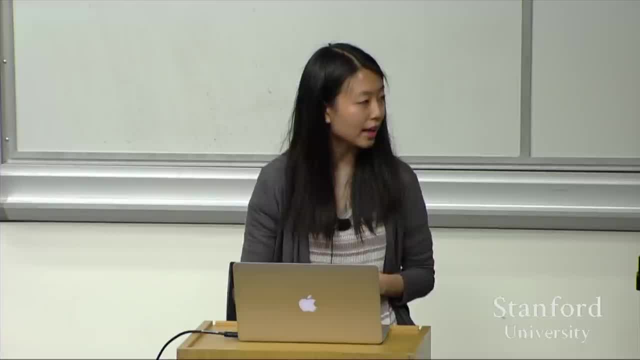 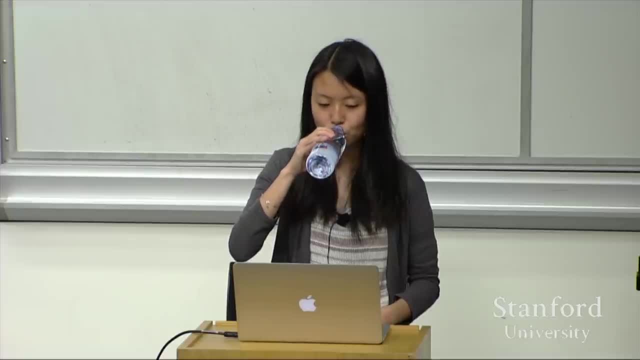 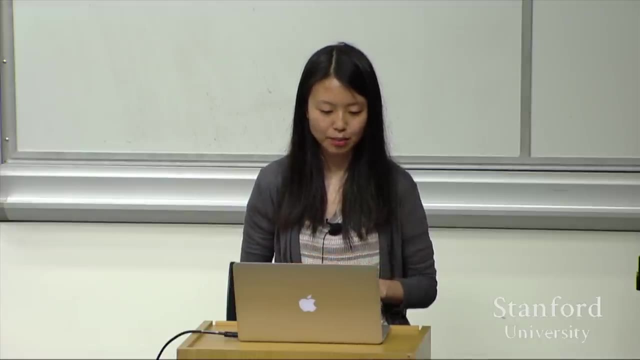 that what these features end up being, when you have a whole stack of these, is these types of simple to more complex features. Okay, so the question is: what's the intuition for increasing the depth each time? Here I had three filters in the original layer. 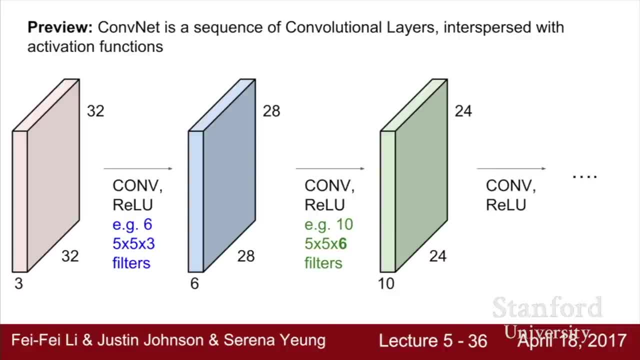 and then six filters in the next layer right, And so this is mostly a design choice. You know, people in practice have found certain types of these configurations to work better, and so later on we'll go into case studies of different kinds of convolutional neural network architectures. 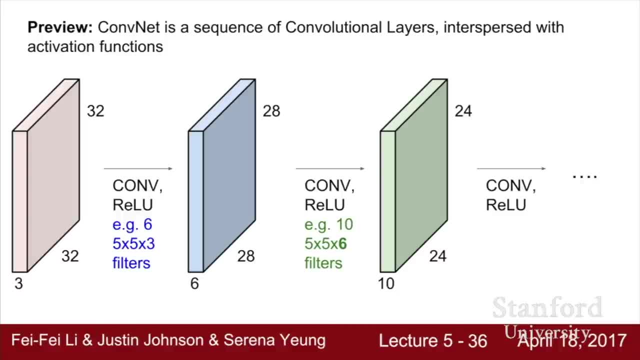 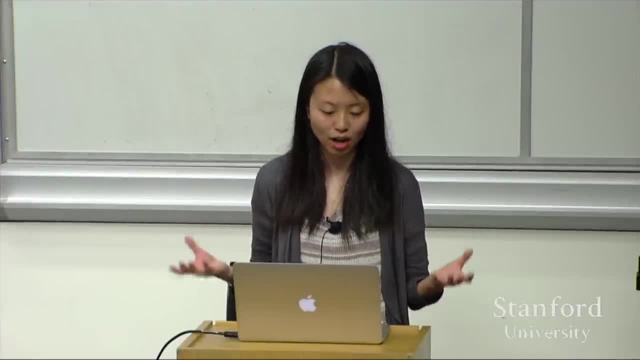 and design choices for these and why certain ones work better than others. But yeah, basically the choice of you're going to have many design choices in a convolutional neural network: The size of your filter, the stride, how many filters you have. 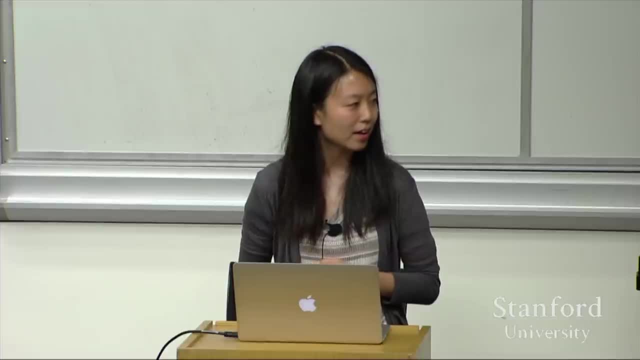 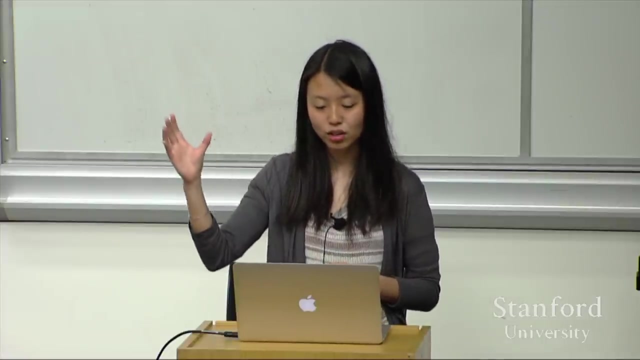 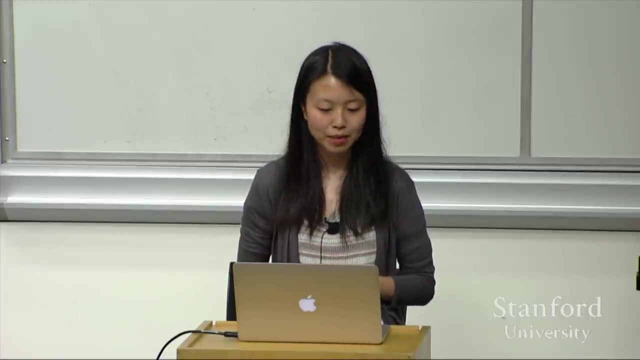 and so we'll talk about this all more later. Questions: Yeah, so the question is: as we're sliding this filter over the image spatially, it looks like we're sampling the edges and corners less than the other locations. Yeah, that's a really good point. 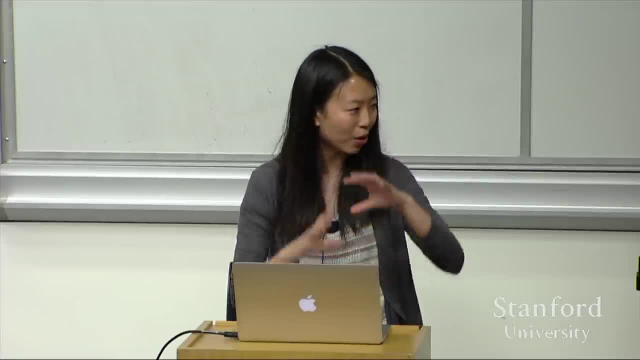 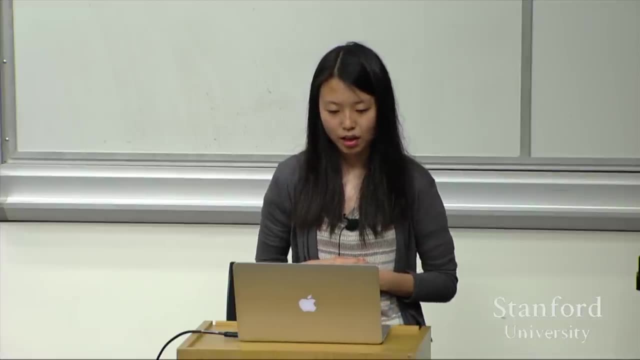 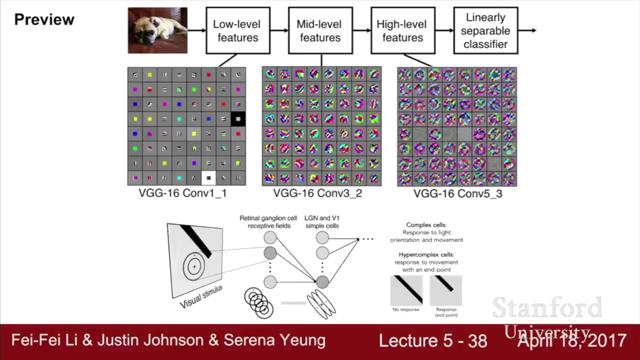 and we'll talk, I think, in a few slides, about how we try and compensate for that. Okay, so you know. so, each of these layers, convolutional layers that we have stacked together, we saw how we're starting with more simpler features. 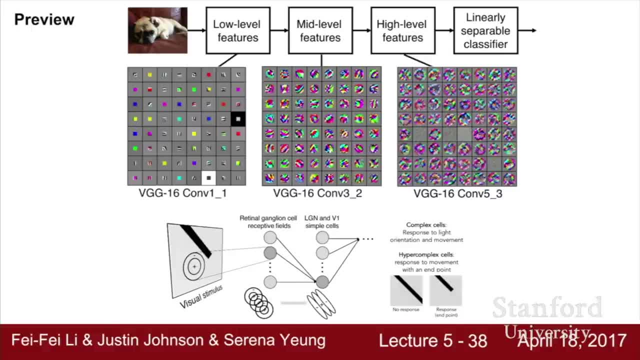 and then aggregating these into more complex features later on. And so in practice, this is compatible with what Tubal and Wiesel noticed in their experiments, right, that we had these simple cells at the earlier stages of processing, followed by more complex cells later on. 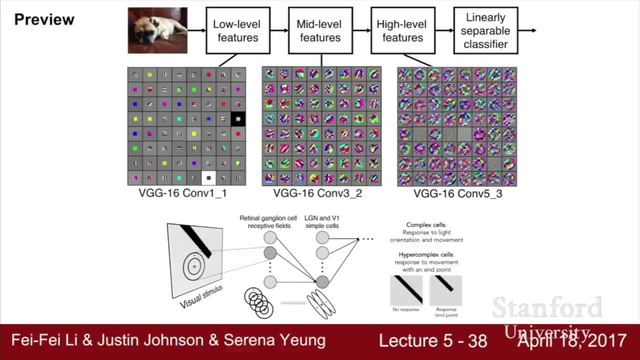 And so, even though we didn't try, we didn't explicitly, you know, force our comment to learn these kinds of features in practice. when you give it this type of hierarchical structure and train it using back propagation, these are the kinds of filters that end up being learned. 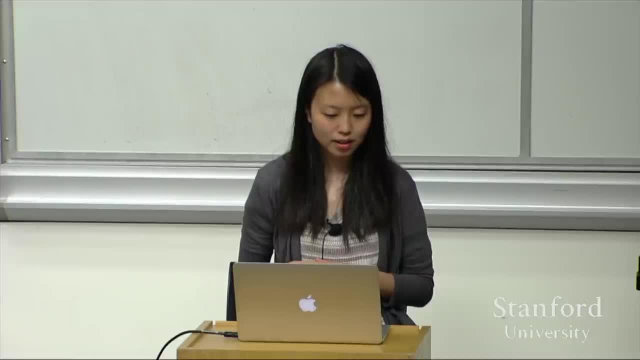 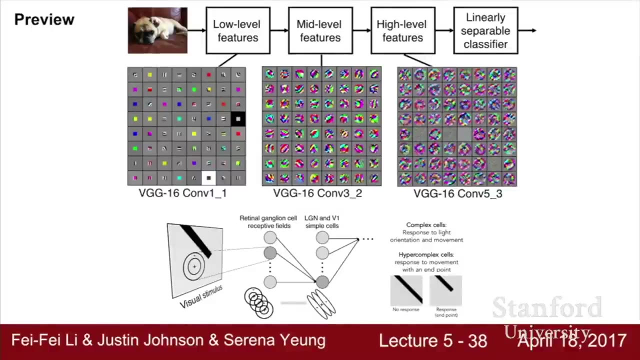 Okay, so, yeah. so the question is, what are we seeing in these visualizations? And so right, so in these visualizations, like if we look at this conv1, the first convolutional layer, each of these grid, each part of this grid, is a one neuron. 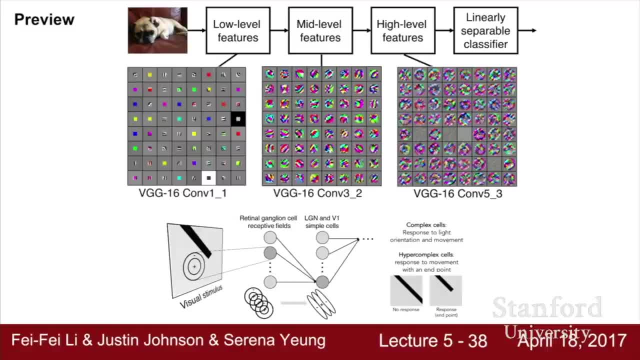 And so what we visualized here is the, what the input looks like that maximizes the activation of that particular neuron. So what sort of image you would get that would give you the largest value, make that neuron fire and have the largest value. 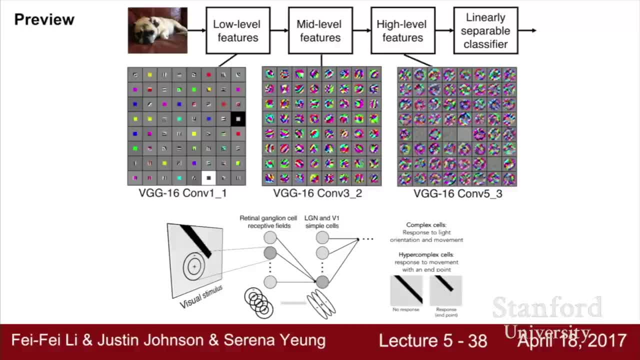 And so the way we do this is basically by, you know, doing kind of back propagation from a particular neuron activation and seeing what in the input will trigger, will give you the highest values of this neuron, And this is something that we'll talk about. 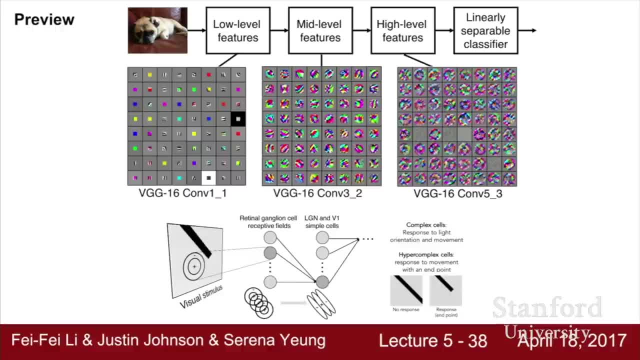 in much more depth in a later lecture about how we create all of these visualizations, But basically each element of these grids is showing what, in the input, would look like. that basically maximizes the activation of the neuron. So, in a sense, what is the neuron looking for? 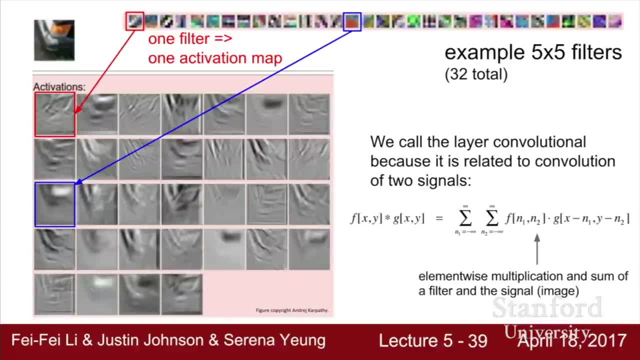 Okay, so here is an example of some of the activation maps produced by each filter, right, So we can visualize up here on the top we have this whole row of example, five by five filters, And so this is basically a real case from a trained commnet, where each of these 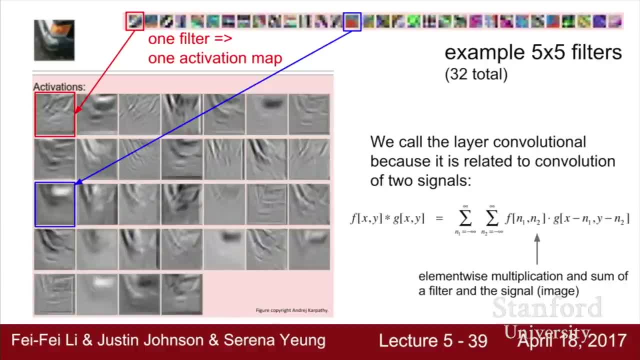 is what a five by five filter looks like, And then, as we convolve this over an image, so in this case I think it's like a quarter of a car, the car light, what the activation looks like, right, And so here, for example, if we look at this first one, 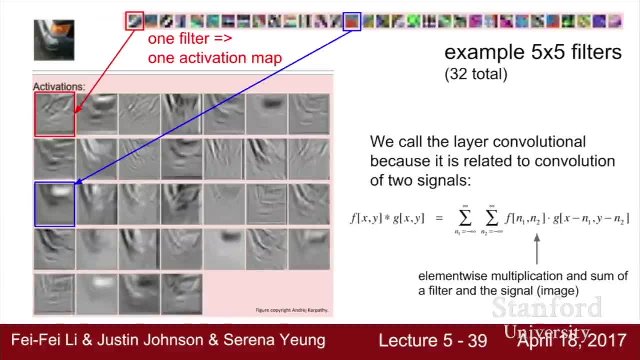 this red filter filter like with the red box around it. we'll see that it's looking for. the template looks like an edge right, an oriented edge, And so if you slide it over here for the image, it'll have a high value. 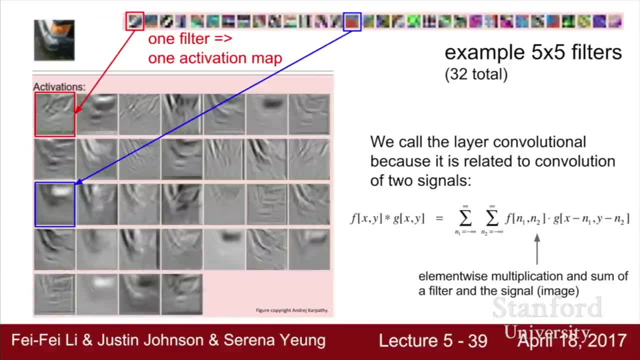 a more white value, where there are edges in this type of orientation, And so each of these activation maps is kind of the output of sliding one of these filters over and where these filters are causing where this sort of template is more present in the image. 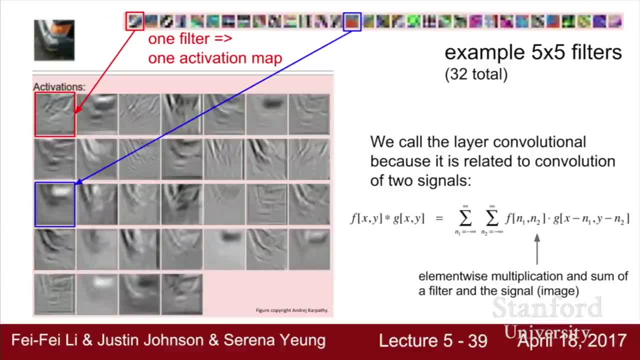 And so the reason we call these convolutional is because this is related to the convolution of two signals, And so someone pointed out earlier that you know this is basically this convolution equation over here for people who have seen convolutions before in signal processing. 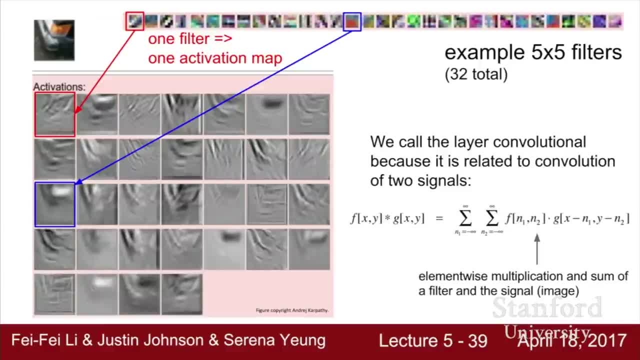 And in practice it's actually more like a correlation where we're convolving with the- you know, flipped version of the filter. But this is- yeah, this is kind of a subtlety- It's not really important for the purposes of this class. 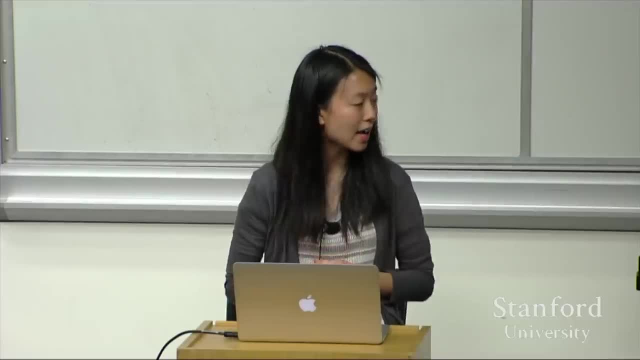 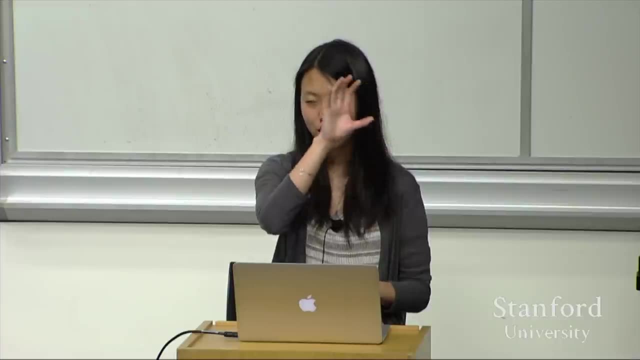 But basically, if you're writing out what you're doing, it has an expression that looks something like this, which is the standard definition of a convolution. But this is basically just taking a filter, sliding it spatially over the image and computing the dot product at every location. 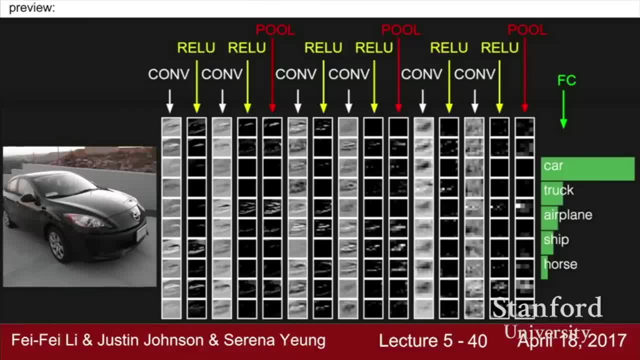 Okay, so you know, as I mentioned earlier, like what our total convolutional neural network is going to look like, is we're going to have an input image and then we're going to pass it through these sequence of layers, right? 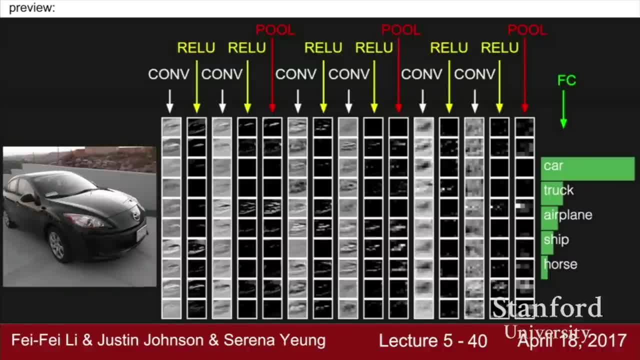 where we're going to have a convolutional layer first And then we're going to have our non-linear layer after that. So a ReLU is something that's very commonly used, that we're going to talk about more later, And then we have these comb ReLU, comb ReLU layers. 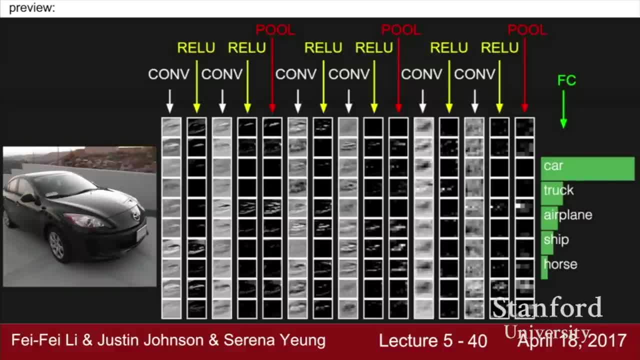 And then, once in a while, we'll use a pooling layer- that we'll talk about later as well- that basically downsamples the size of our activation maps And then, finally, at the end of this, we'll have take our last convolutional layer output. 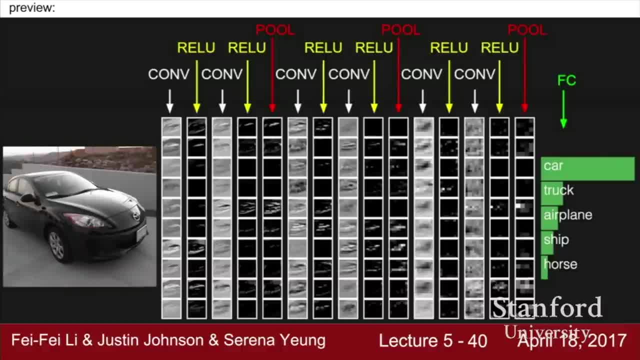 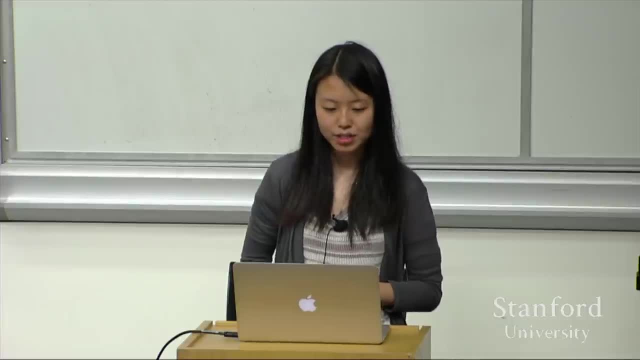 and then we're going to use a fully connected layer that we've seen before, connect it to all of these convolutional outputs and use that to get a final score function- basically like what we've already been working with. Okay, so now let's work out some examples. 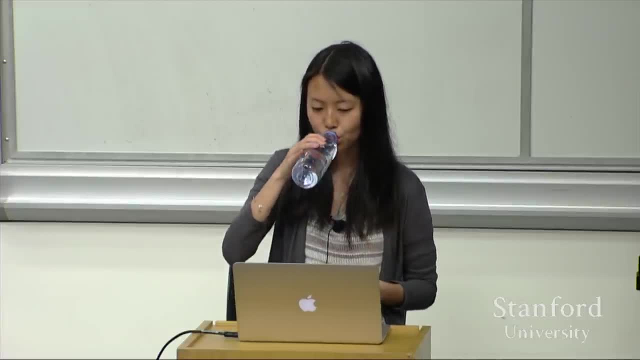 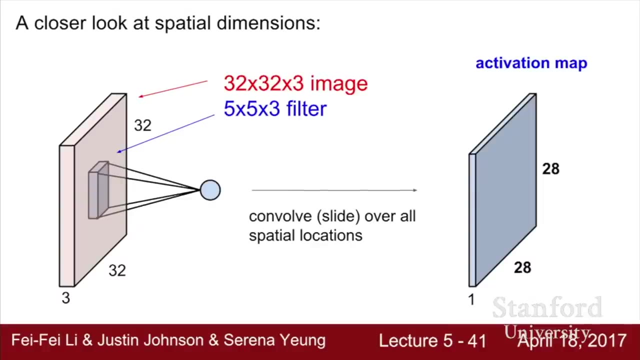 of how the spatial dimensions work out. So let's take our 32 by 32 by three image, as before, right, and we have our five by five by five by three filter that we're going to slide over this image And we're going to see how we're going to use that. 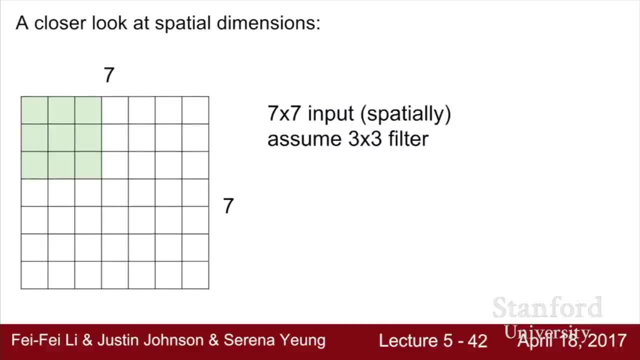 to produce exactly this 28 by 28 activation map. So let's assume that we actually have a seven by seven input, just to be simpler, and let's assume we have a three by three filter. So what we're going to do is we're going to take this filter. 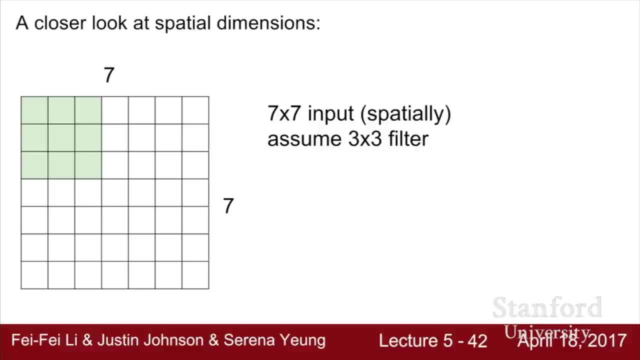 plop it out, plop it down in our upper left hand corner, right, and we're going to multiply, do the dot product, multiply all these values together to get our first value, And this is going to go into the upper left hand corner. 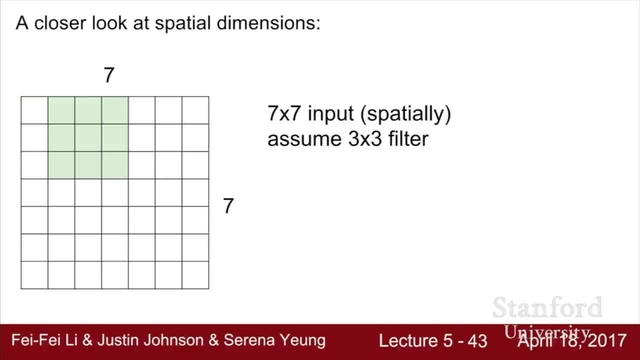 This is going to be the top ten value of our activation map Right, and then what we're going to do next is we're just going to take this filter, slide it one position to the right, and then we're going to get another value out from here. 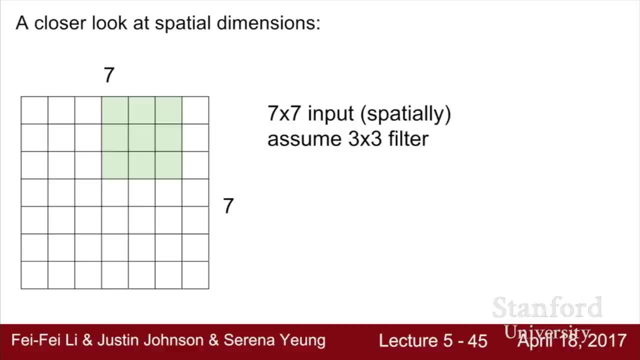 And so we can continue with this to have another value, another, and in the end, what we're going to get is a five by five output. right, because what fit was basically sliding this filter, a total of, you know, at five spatial locations horizontally. 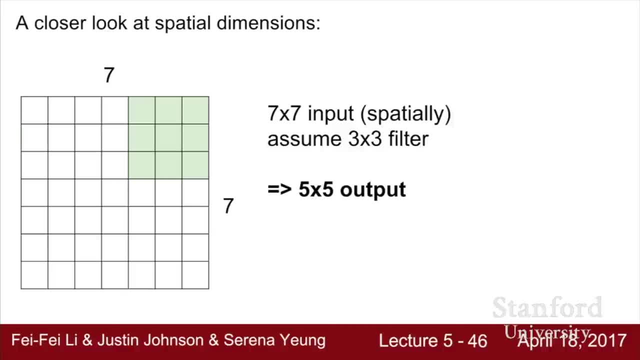 and five spatial locations vertically. Okay, so, as I said before, there's different kinds of design choices that we can make, Right? so previously I slid it at every single spatial location and the interval at which I slide I'm going to call the stride. 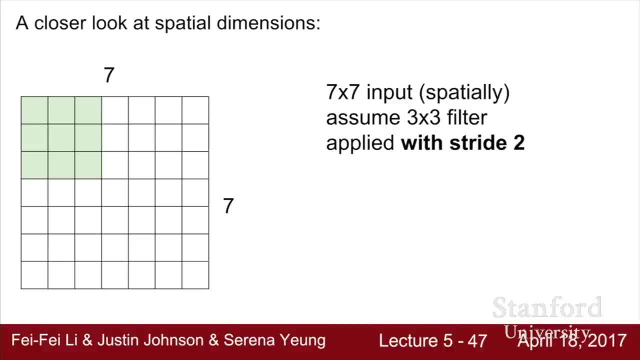 And so previously we used the stride of one, And so now let's see what happens if we have a stride of two. Right, so now we're going to take our first location, the same as before, and then we're going to skip, this time two pixels over. 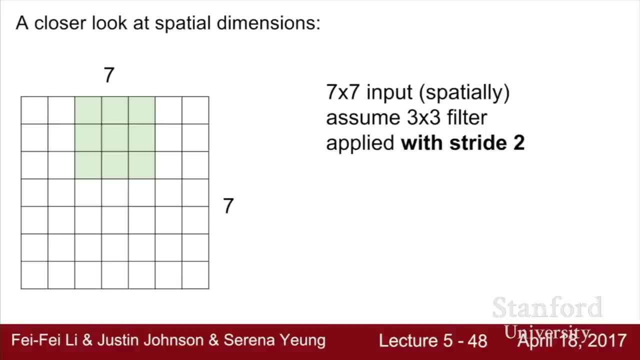 and we're going to get our next value centered at this location. Right, and so now, if we use a stride of two, we have in total three of these that can fit, and so we're going to get a three by three output. 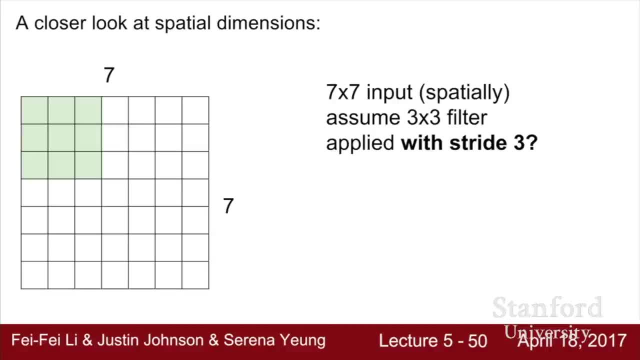 Okay, and so what happens when we have a stride of three? What's the output size of this? And so, in this case, right, we have three, we slide it over by three again, and the problem is that here it actually doesn't fit. 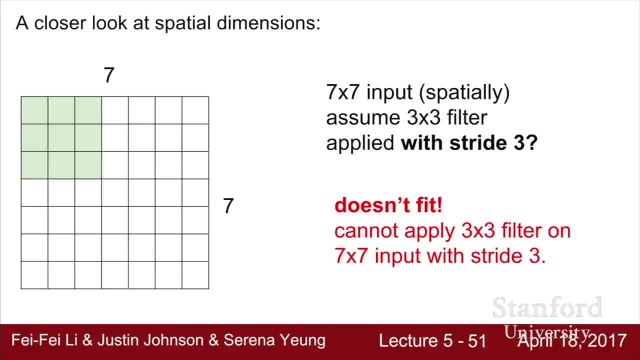 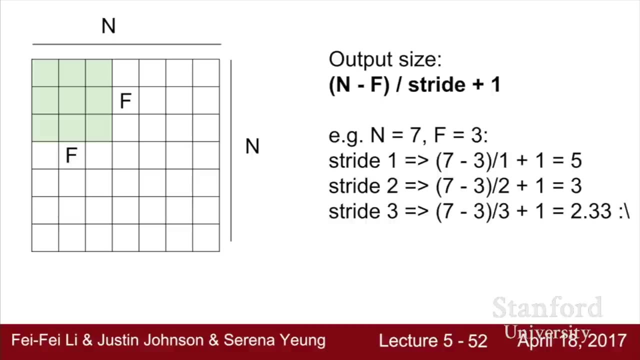 Right, so we slide it over by three, and now it doesn't fit nicely within the image. And so what we in practice? we just, it just doesn't work. We don't do convolutions like this because it's going to lead to asymmetric outputs happening. 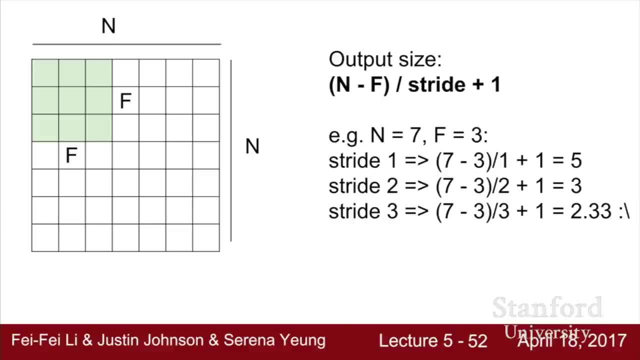 Right and so just kind of looking at the way that we computed how many, what the output size is going to be, this actually can work into a problem. So we have a nice formula where we take our dimension of our input n, we have our filter size, f. 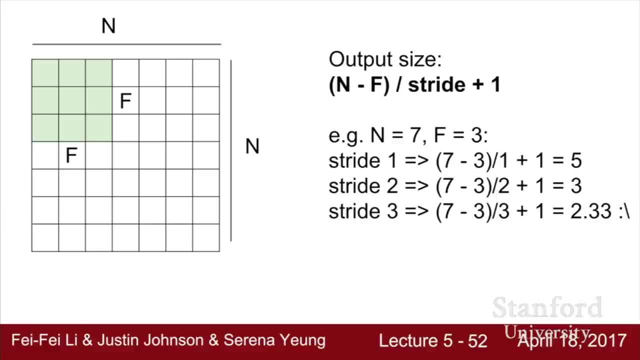 we have our stride at which we're sliding along and our final output size. each the dimension, spatial dimension of each output size is going to be n minus f divided by the stride plus one Right, and you can kind of see this as a. 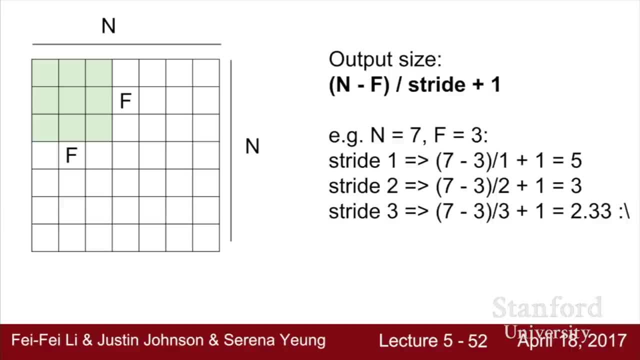 you know if I'm going to take my filter. let's say I fill it in at the very last possible position that it can be in and then take all the pixels before that. how many, how many instances of of moving by the stride can I fit in? 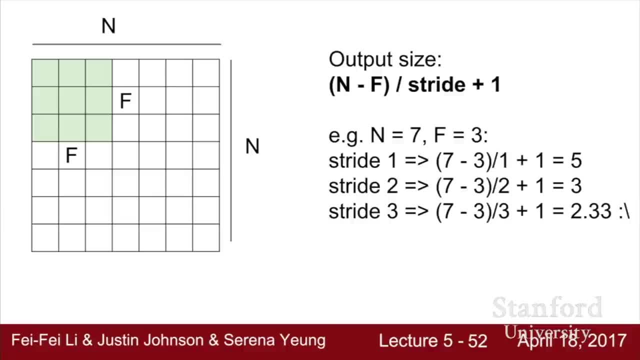 Right, and so that's how this equation kind of works out. And so, as we saw before, right if we have n equals seven and f equals three. if we want a stride of one, we plug it into this formula. we get five by five, as we had before. 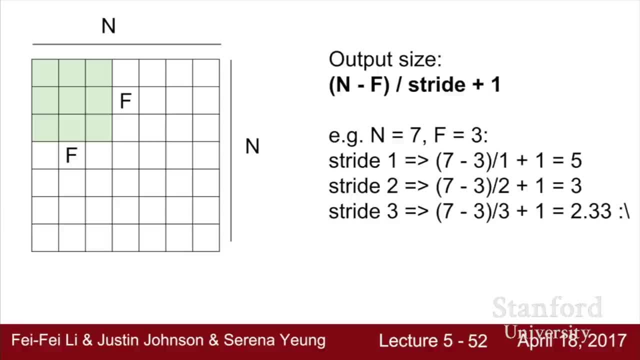 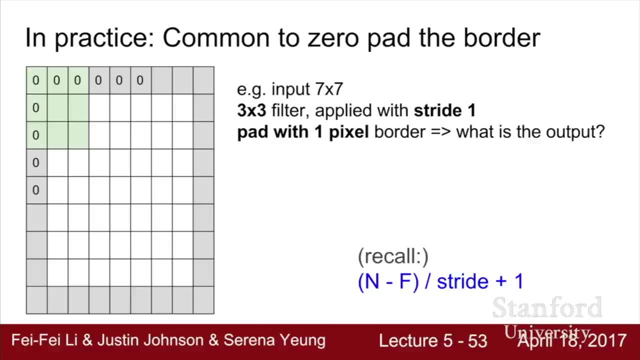 and the same thing for two, And with a stride of three, this doesn't really work out, And so in practice it's pretty common to zero, pad the borders in order to make the size work out to what we want it to, And so this is kind of related to a question earlier. 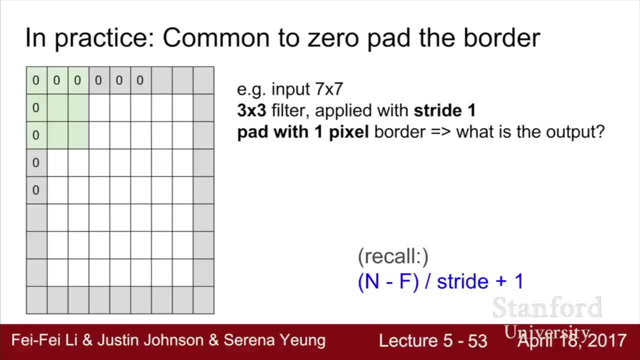 which is what do we do right at the corners, And so what in practice happens is we're going to actually pad our input image with zeros, and so now you're going to be able to place a filter centered at the upper right hand pixel location. 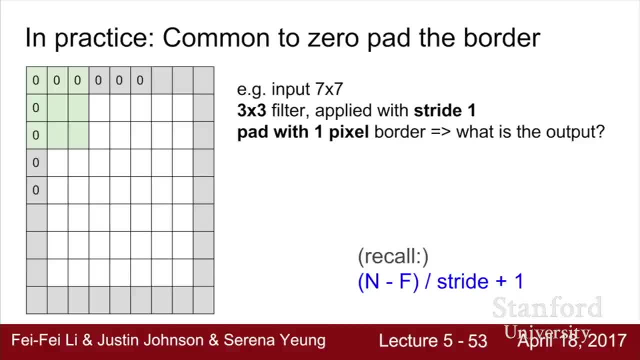 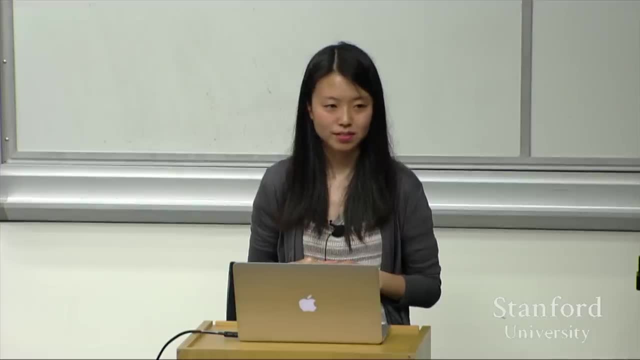 of your actual input image. Okay, so here's a question. So who can tell me if I have my same input? seven by seven, three by three, filters, slide one, but now I pad with a one pixel border. what's the size of my output going to be? 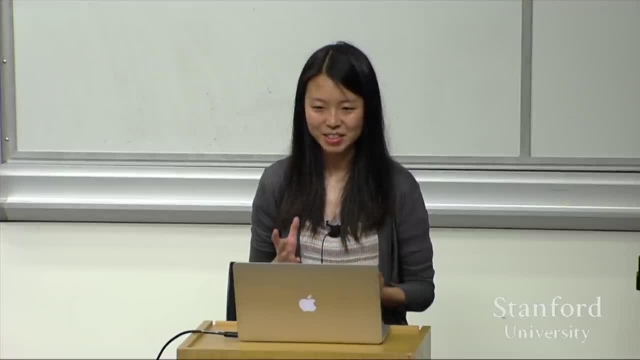 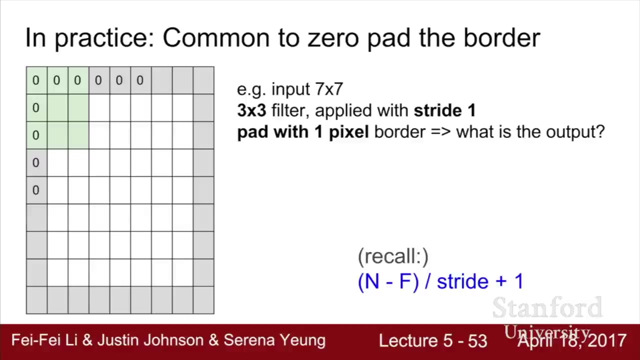 So I'm hearing, I heard some sixes. So remember, we have this formula that we have before. So if we plug in, n is equal to seven, f is equal to three right, and then our stride is equal to one. so what we actually get, 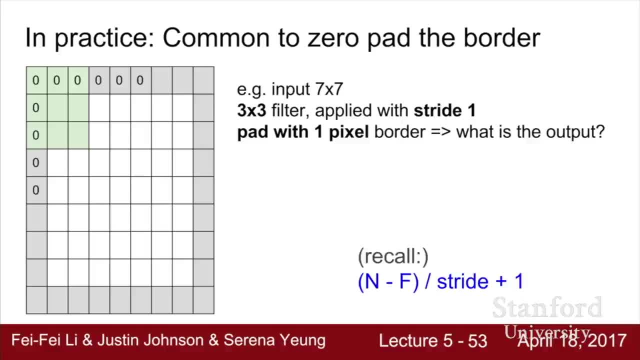 so actually this is giving us seven by four. so seven minus three is four. divided by one plus one is five, And so this is what we had before. So we actually need to adjust this formula a little bit. So this was actually. this formula is the case. 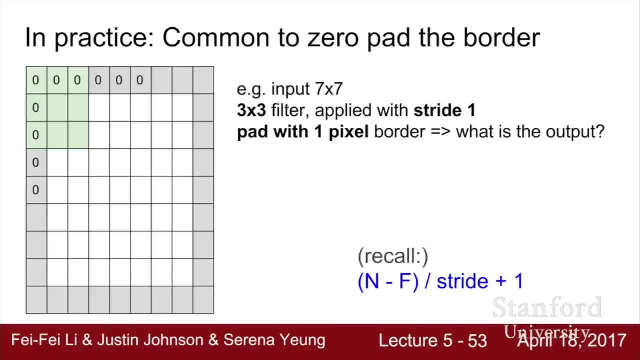 where we don't have zero padded pixels. But if we do pad it then if you now take your new output and you slide it along, you'll see that actually seven of the filters fit. so you get a seven by seven output And plugging in our original formula right. 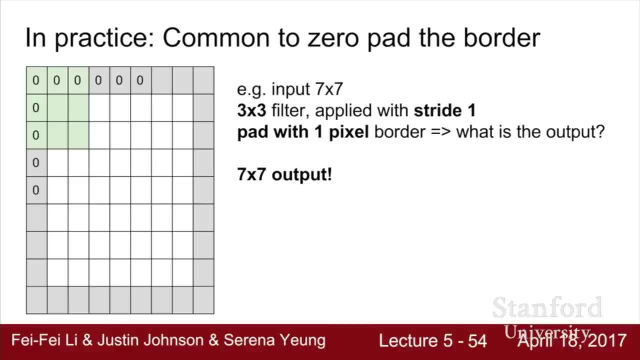 so our n now is not seven, it's nine. So if we go back here, we have n equals nine, minus the filter size of three, which gives six right divided by our stride, which is one, and so it's still six. 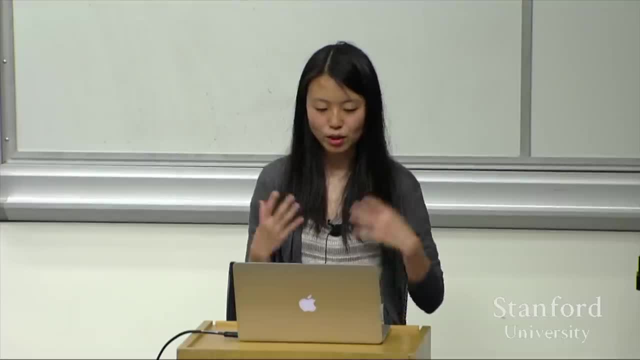 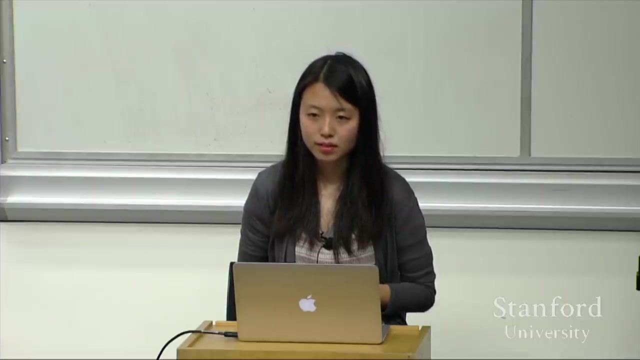 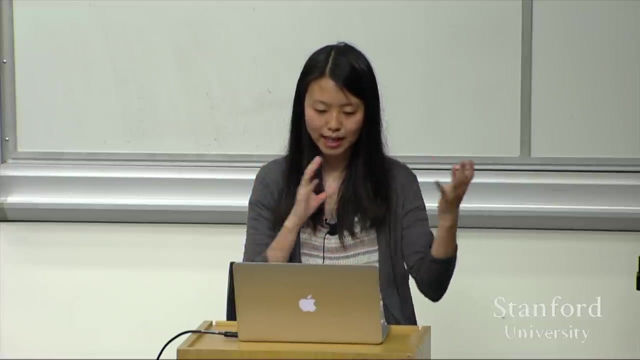 and then plus one, we get seven Right. and so, once you've padded it, you want to incorporate this padding into your formula. Yes, question Seven. Okay, so the question. so the question is: what's the actual output of the size? 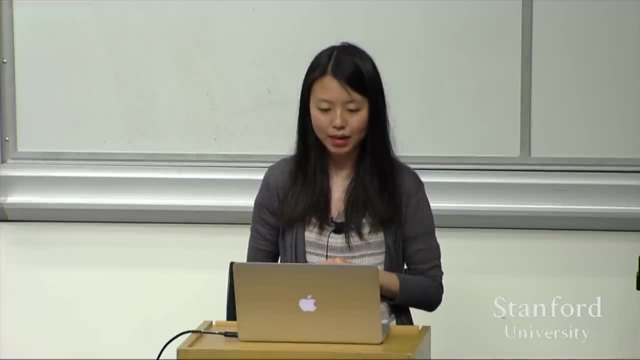 Is it seven by seven or seven by seven by three? The output is going to be seven by seven by the number of filters that you have. So remember, each filter is going to do a dot product through the entire depth of your input volume. 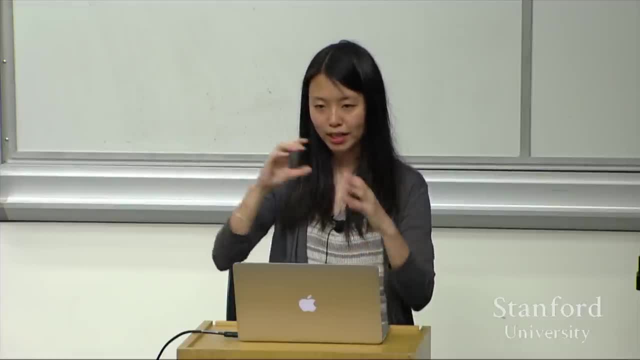 But then that's going to produce one number, right? So each filter is- let's see if we can well go back here- Each filter is producing a one by, you know, seven by seven, in this case activation map output. 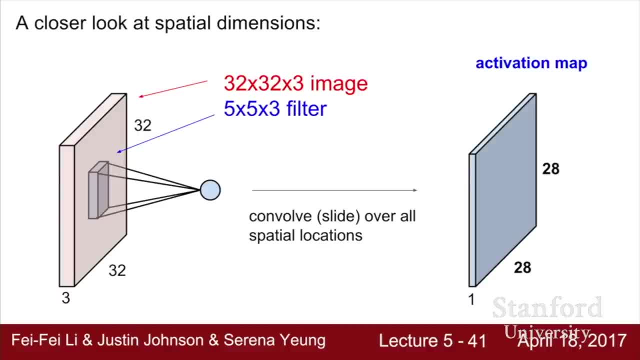 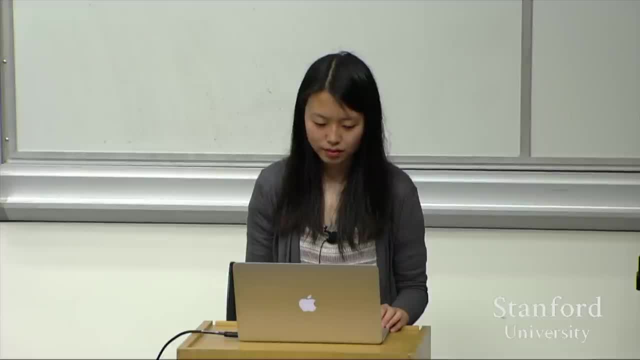 And so the depth is going to be the number of filters that we have. And let's see, since we've already used two or more filters, can we go back just a little bit? Sorry, let me just one second go back. 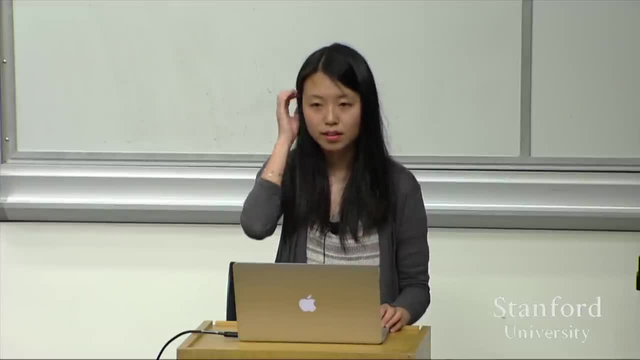 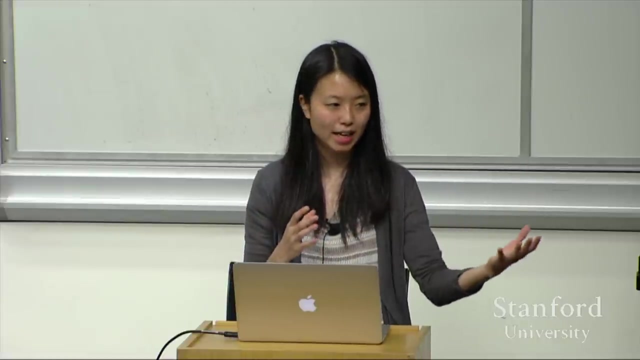 Okay, can you repeat your question again? Okay, so the question is: how does this connect to before, when we had a 32 by 32 by 3 input, right? So our input had depth and here in this example, I'm showing a 2D example with no depth. 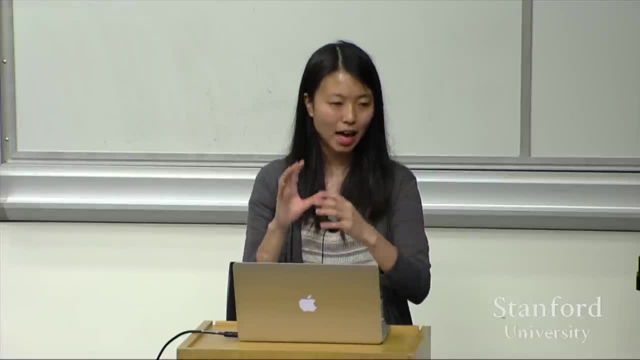 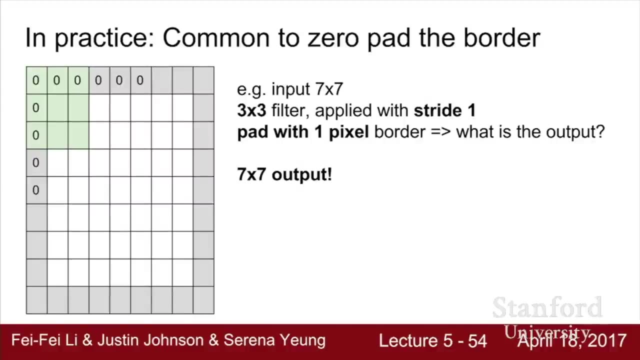 And so, yeah, so I'm showing this for simplicity, but in practice, you're going to take your, you're going to multiply throughout the entire depth, as we had before. So you're going to. your filter is going to be, in this case, a 3 by 3 spatial filter. 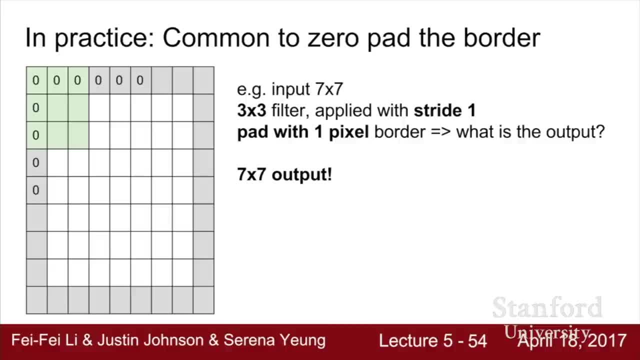 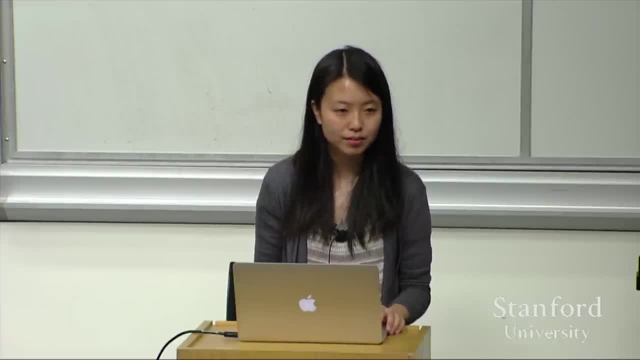 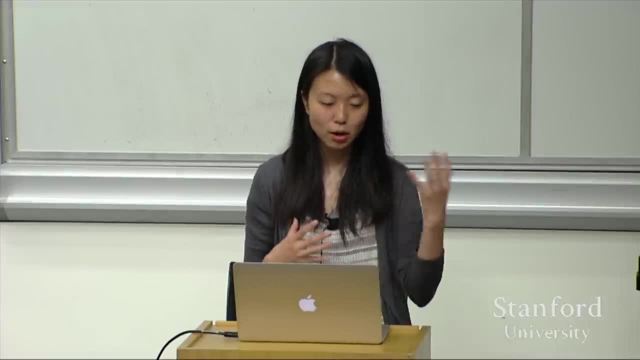 by whatever input depth that you had, so 3 by 3 by 3 in this case. Yeah, everything else stays the same. Yes, question, Yeah. so the question is: does the zero padding add some sort of extraneous features? 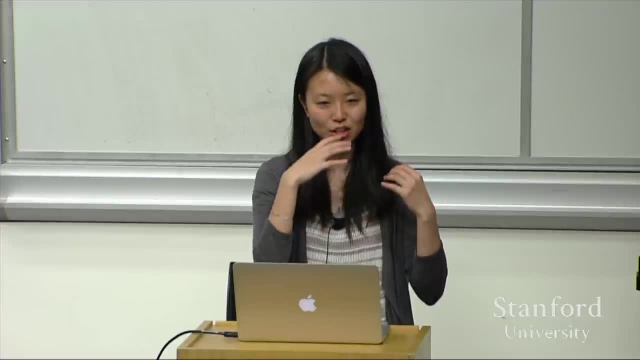 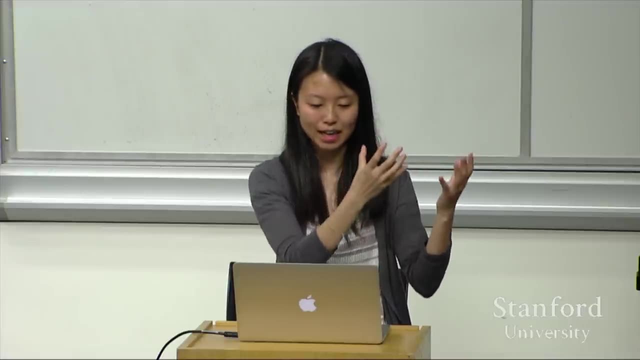 at the corners And yeah. so I mean we're doing our best to still, you know, get some value and do like process that region of the image And so zero padding. It's kind of one way to do this, where you know I guess we can. we are detecting part. 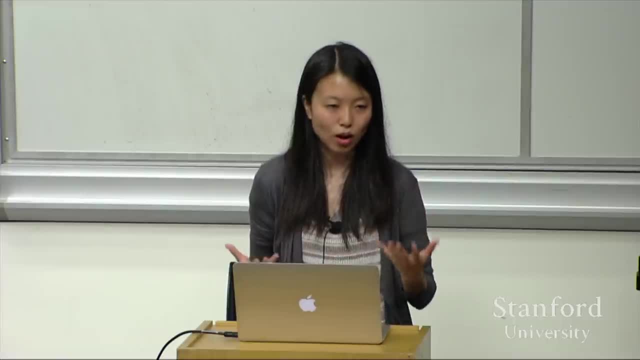 of this template in this region. There's also other ways to do this that you know. you can try and like, mirror the values here or extend them, And so it doesn't have to be zero padding, but in practice this is one thing that works. 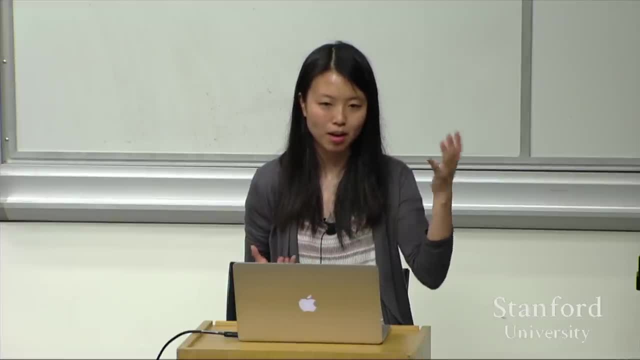 reasonably And so yeah, so there is a little bit of kind of artifacts at the edge and we- sort of just you- do your best to deal with it And in practice this works reasonably. I think there was another question. 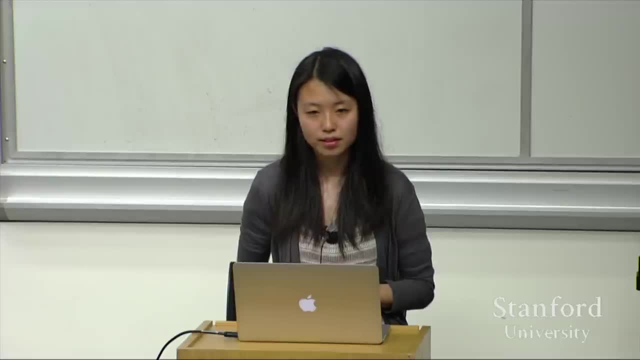 Yeah question. So if we have non-square images, do we ever use a stride that's different horizontally and vertically? So I mean, there's nothing stopping you from doing that You could, but in practice we just usually take the same stride. 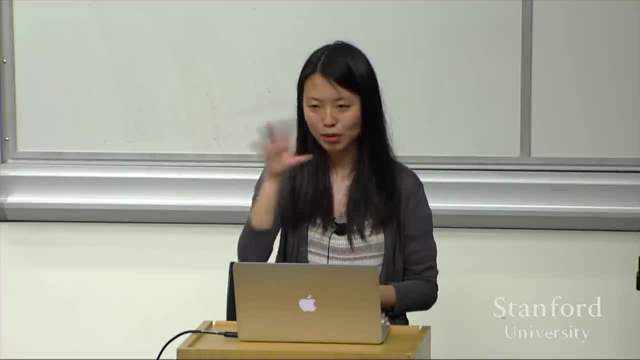 We usually operate over square regions and we just- yeah, we usually just take the same stride everywhere. So, like, in a sense, it's a little bit like, it's a little bit like the resolution at which you're, you know, looking at this image, 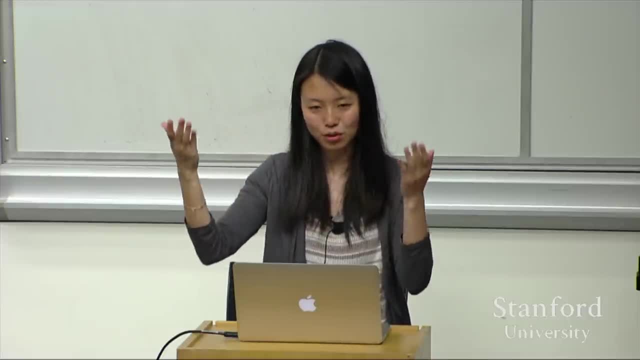 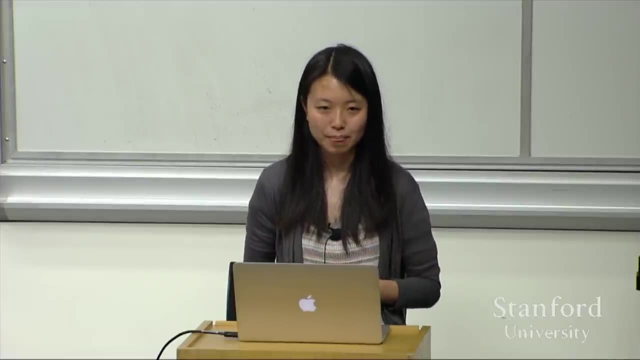 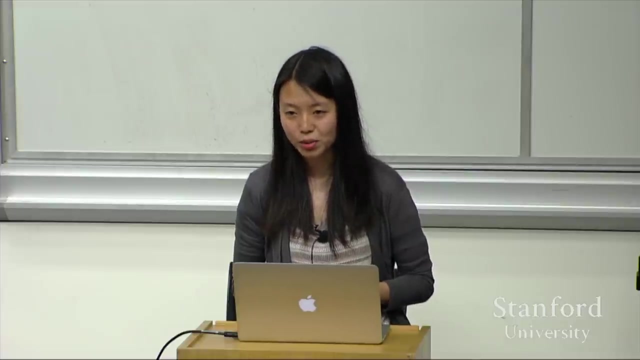 And so usually there's kind of you might want to match sort of your horizontal and vertical resolutions, But yeah, so in practice you could, but really people don't do that. Okay, another question: Why so? the question is, why do we do zero padding? So the way we do zero padding is two things. One is you know. you have to have you know, you have to have you know, you have to have a lot of you know, you have to have a lot of you know, you have to have a lot of you know. 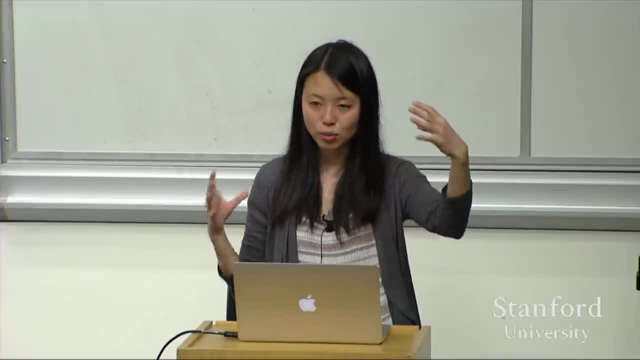 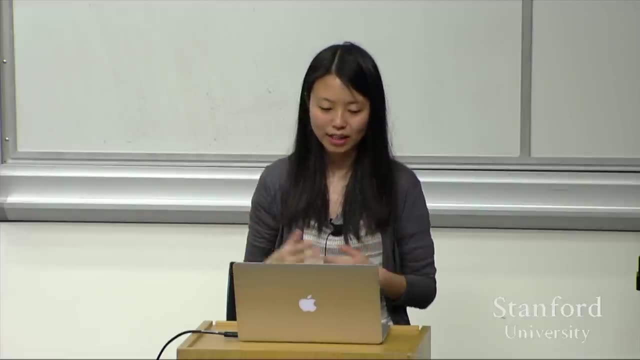 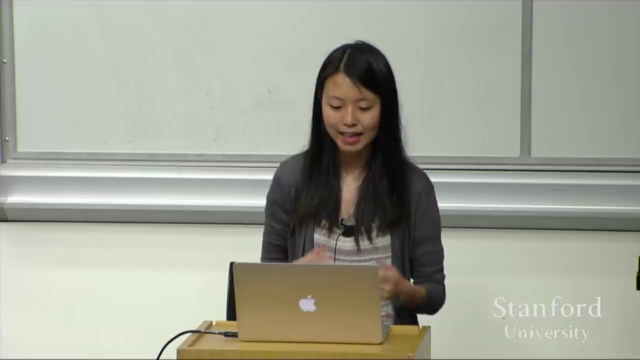 you have to have. you know you have to have a lot of. you know you have to have a lot of preserve time between your three rows of threads. So we juegos like because of the same reason, we know that there are three rows of content. 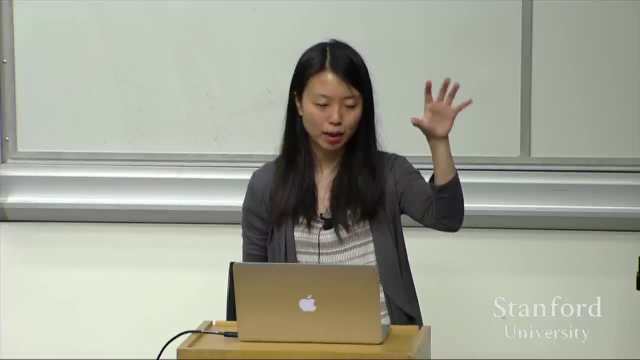 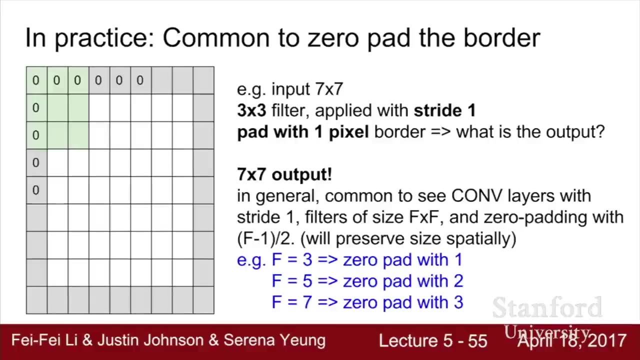 and one color, Okay, Okay, as apply your filter at these corner regions and edge regions. And so, in general, in terms of choosing your stride, your filter size, your stride size, zero padding, what's common to see is filters of size three by three, five by five, seven by seven. 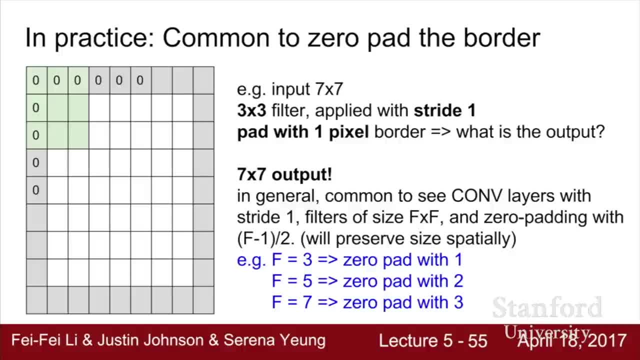 These are pretty common filter sizes, And so, each of these for three by three, you will want to zero pad with one in order to maintain the same spatial size. If you're going to do five by five, you can work out the math, but it's going to come out to 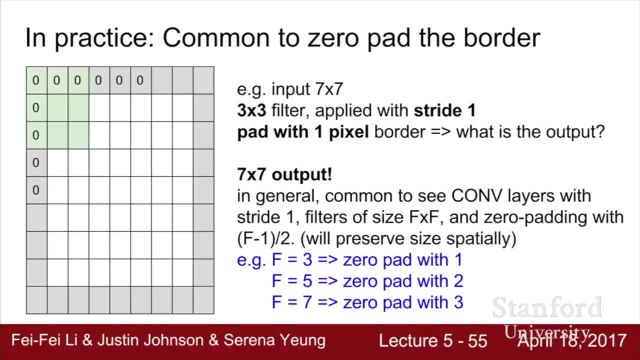 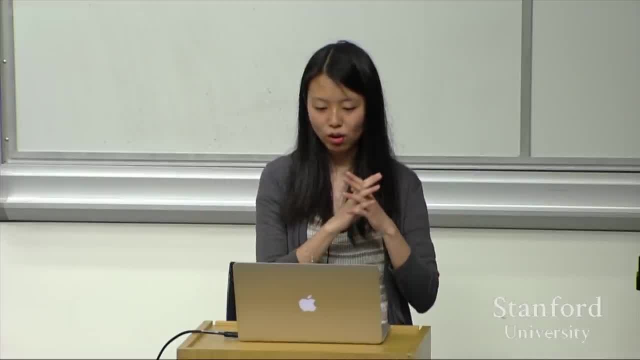 you want to zero pad by two, and then for seven you want to zero pad by three. Okay, and so again the motivation for doing this type of zero padding and trying to maintain the input size. So we kind of alluded to this before. 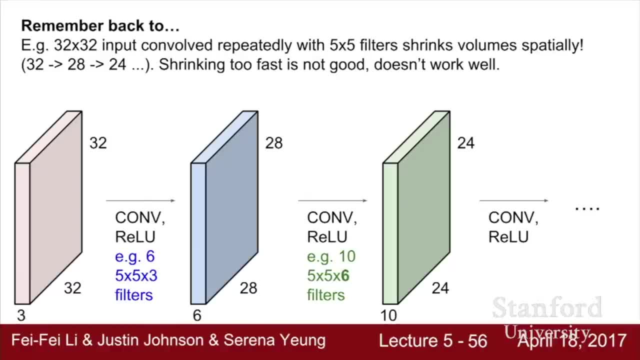 but if you have multiple of these layers stacked together, so if you have multiple of these layers stacked together, you'll see that if we don't do this kind of zero padding or any kind of padding, we're going to really quickly shrink the size of the outputs that we have. 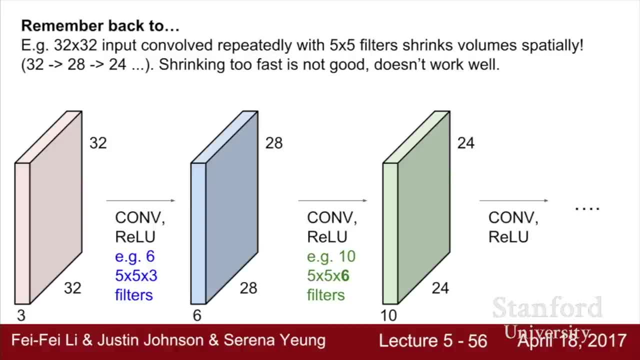 And so this is not something that we want. Like you can imagine, if you have a pretty deep network, then very quickly the size of your activation map is going to shrink to something very small, And this is bad both, because now we're kind of losing out. 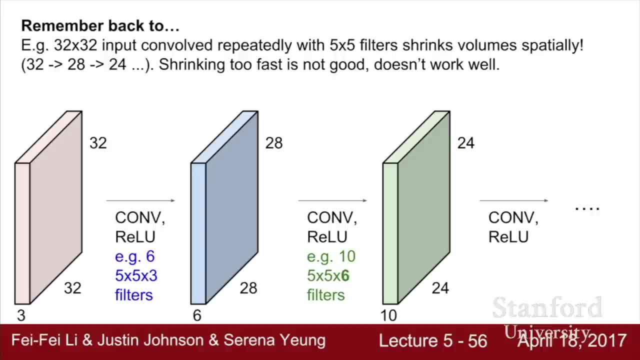 on some of this information. right Now, you're using a much smaller number of values in order to represent your original image, So you don't want that, And then at the same time, also as we talked about earlier- you're also kind of losing some of this edge information. 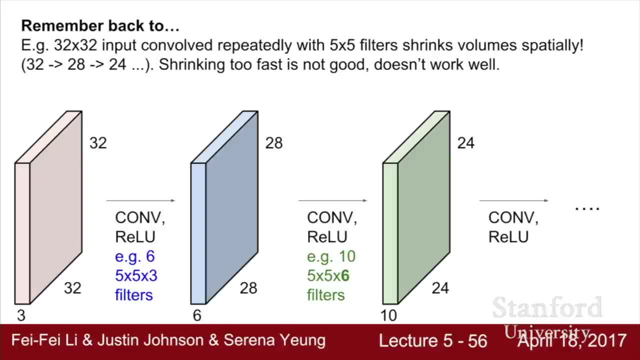 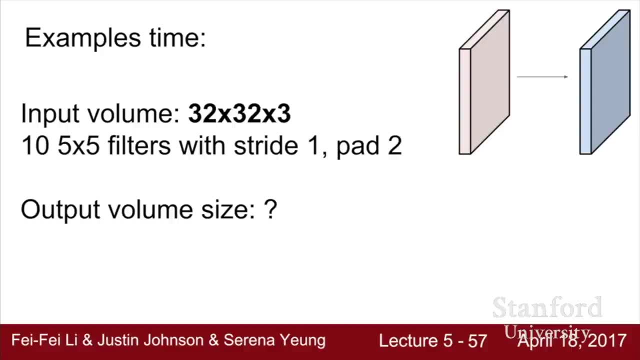 corner information that each time we're losing out and shrinking that further. Okay, so let's go through a couple more examples of computing some of these sizes. So let's say that we have an input volume which is 32 by 32.. 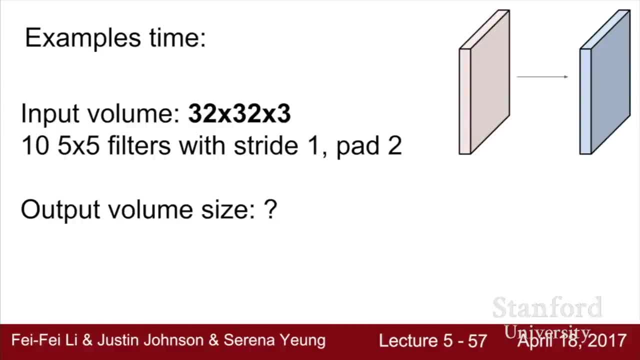 32 by 32.. 32 by 32.. And here we have 10 five by five filters. Let's use stride one and pad two. And so who can tell me what's the output volume size of this? So you can think about the formula earlier. 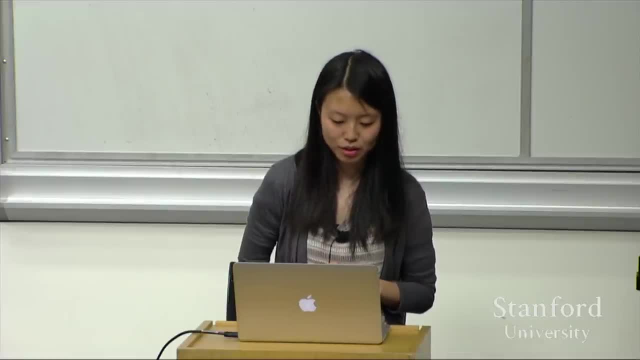 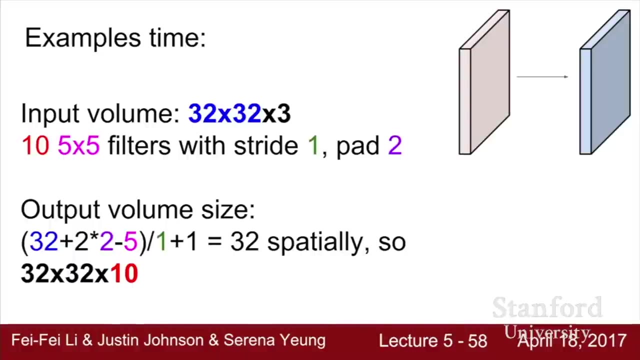 Sorry, what was it? 32 by 32 by 10.. 32 by 32 by 10.. Yes, that's correct, And so the way we can see this right is: so we have our input. size F is 32.. 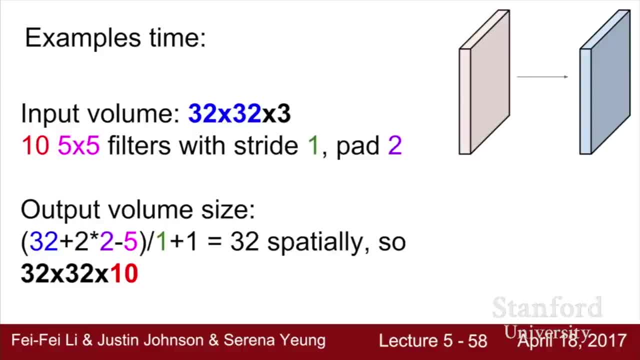 And in this case we want to augment it by the padding that we added onto this. So we padded two in each dimension, so we're actually gonna get total width and total height is gonna be 32, plus four on each side And then minus our filter size five. 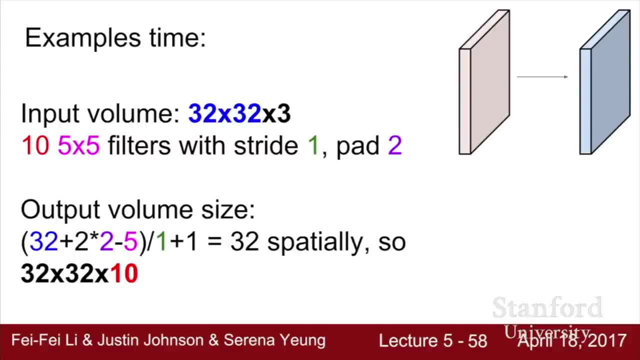 divided by one plus one and we get 32.. So our output is going to be 32 by 32 for each filter, And then we have 10 filters total. So we have 10 of these activation maps And our total output volume is going to be: 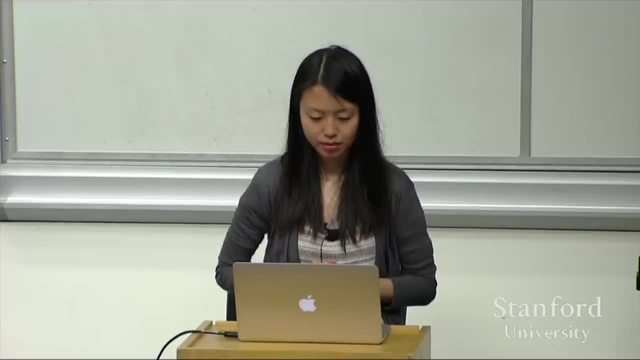 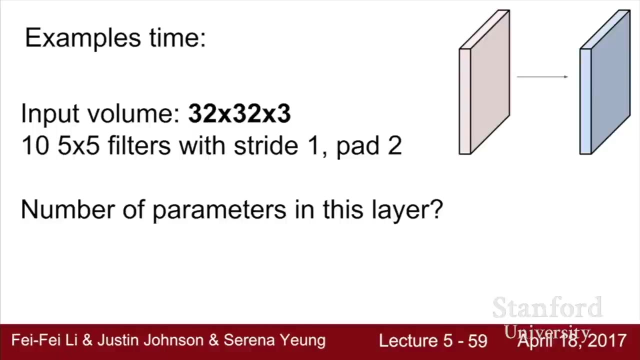 32 by 32 by 10.. Okay, next question: So what's the number of parameters in this layer? So remember, we have 10 five by five filters. I kind of heard something, but it was quiet. 245.. 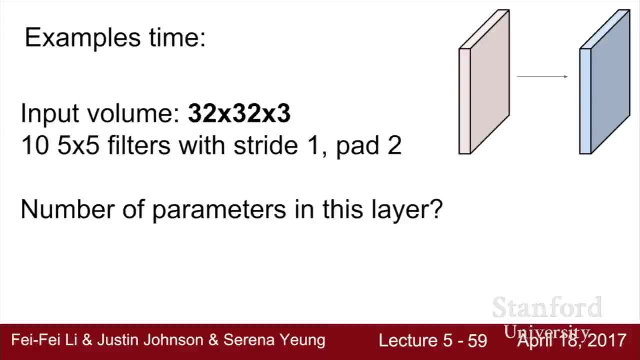 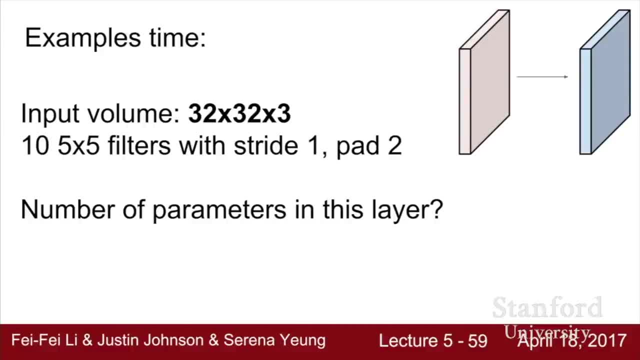 245. 245. 245.. Okay, so I heard 250,, which is close, But remember that we're also our input volume. each of these filters goes through by depth, So maybe this wasn't clearly written here, because each of the filters is five by five. 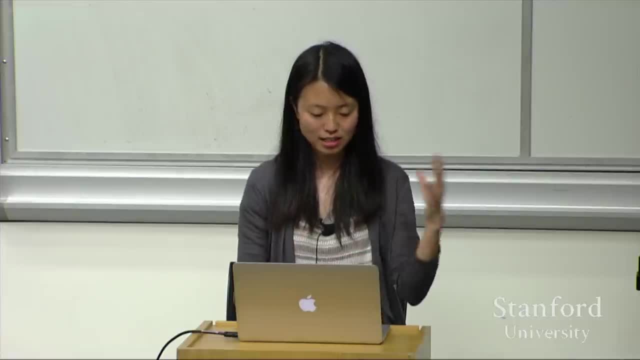 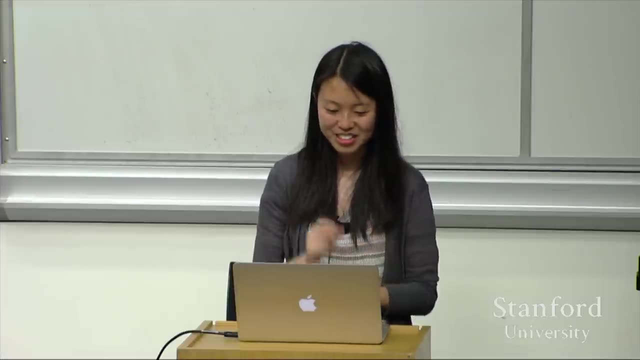 spatially, But implicitly, we also have the depth in here. right, It's gonna go through the whole volume. So I heard, yeah, 750, I heard Almost there. this is kind of a trick question because, also, remember, we usually always have. 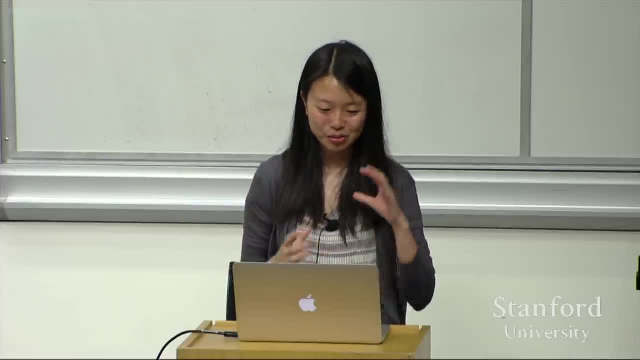 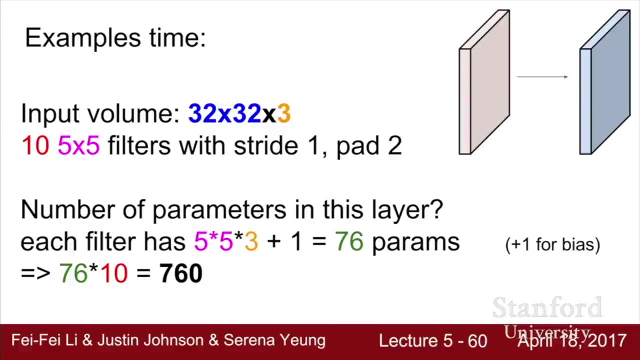 a bias term, right? So in practice each filter has a bias. So each filter has five by five, by three weights plus our one bias term. we have 76 parameters per filter, and then we have 10 of these total, and so there's 760 total parameters. 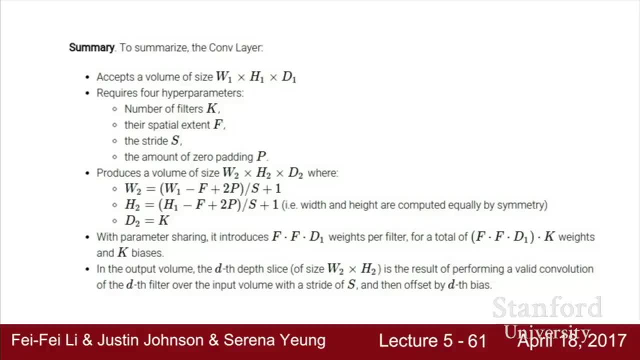 Okay, and so here's just a summary of the convolutional layer that you guys can read a little bit more carefully later on. but we have our input volume of a certain dimension, we have all these choices, we have our filters right. we have number of filters, the filter size. 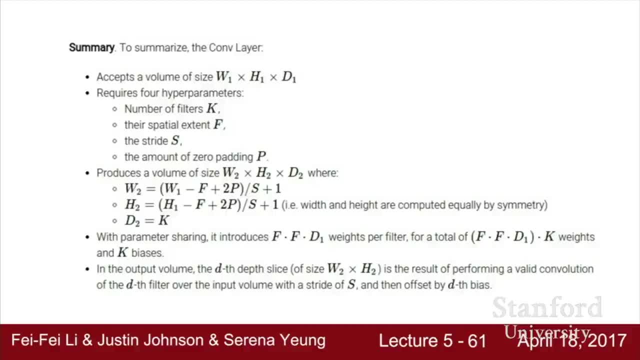 the stride of the size, the amount of zero padding, and you basically can use all of these. go through the computations that we talked about earlier in order to find out what your output volume is actually going to be and how many total parameters that you have. 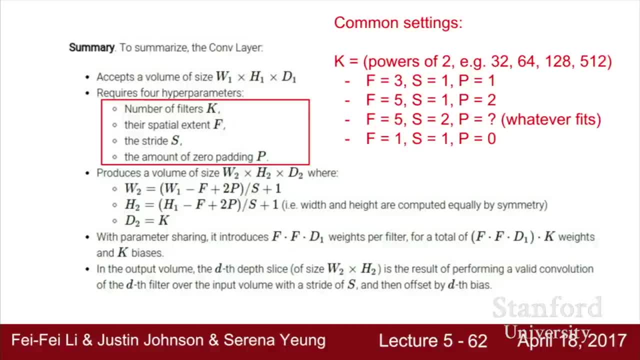 And so some common settings of this. you know, we talked earlier about common filter sizes of three by three, five by five. stride is usually, you know, one and two is pretty common, And then you're padding, P is going to be whatever fits. 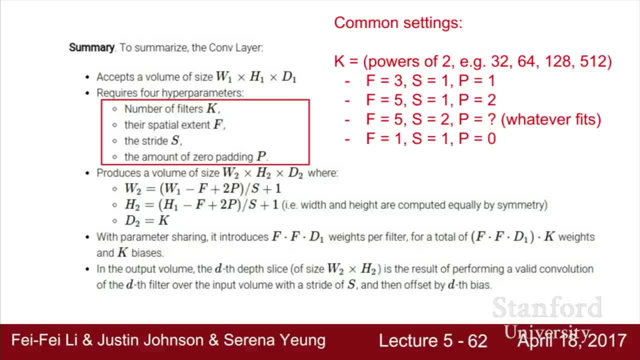 like. whatever you know will preserve your spatial extent is what's common. And then the total number of filters, K. usually we use powers of two, just to be nice. so you know 32,, 64,, 128, and so on 512,. 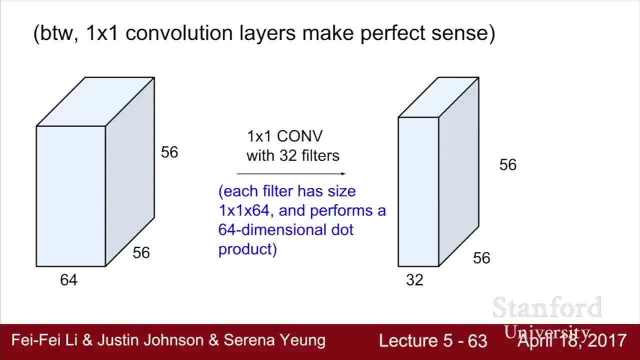 these are pretty common numbers, that you'll see. And, just as an aside, we can also do a one by one convolution. this still makes perfect sense where, given a one by one convolution, we still slide it over each spatial extent. but now the you know, the spatial region. 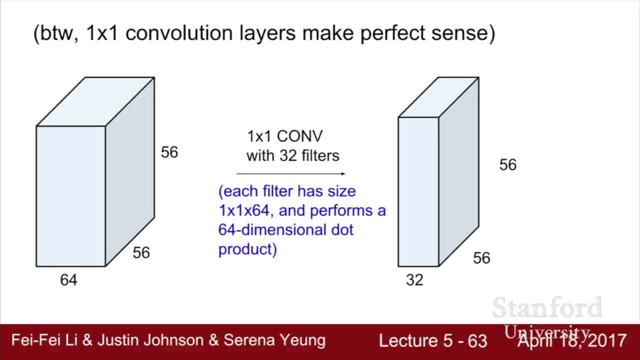 is not really five by five, it's just kind of the trivial case of one by one, but we are still, you know, having this filter go through the entire depth, right. So this is going to be a dot product through the entire depth of your input volume. 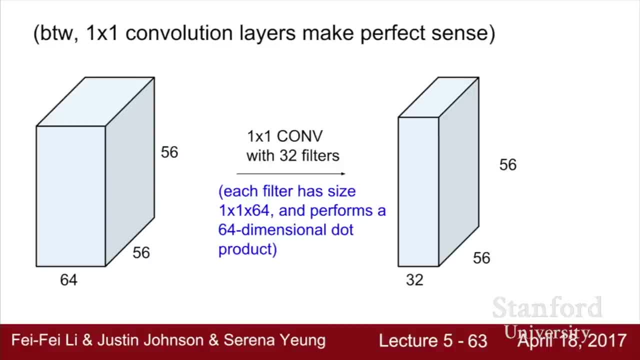 And so the output here right? if we have an input volume of 56 by 56 by 64 depth and we're going to do one by one convolution with 32 filters, then our output is going to be 56 by 56, by our number of filters, 32.. 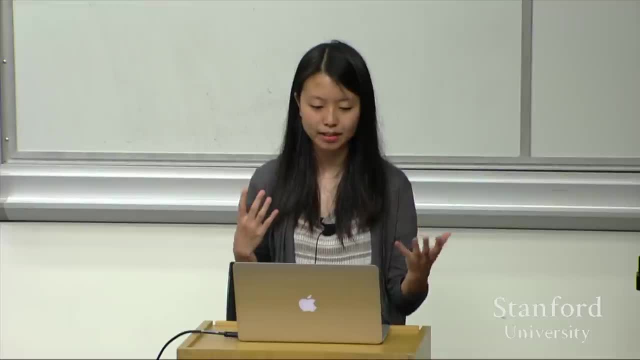 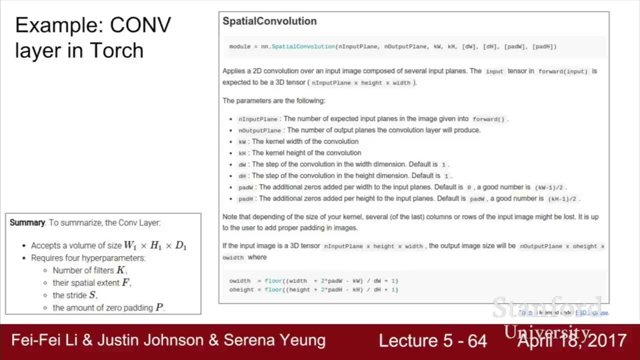 Okay, and so here's an example of a convolutional layer in, you know, TORCH deep learning framework, and so you'll see that in the last lecture we talked about how you can go into these deep learning frameworks. you can see these definitions of each layer, right. 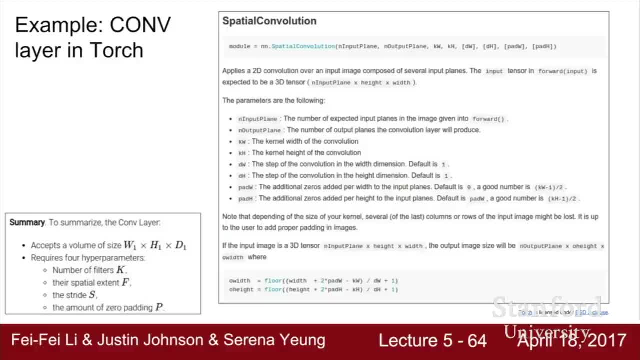 Where they had kind of the forward pass and the backward pass implemented for each layer. And so you'll see, you know, convolution, that kind of stuff, immольше There are certain Spatial convolution is going to be just one of these. 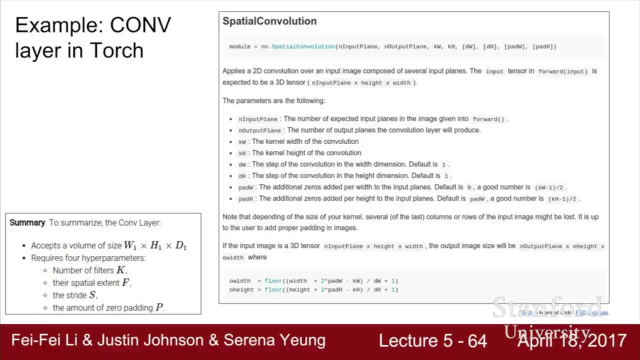 And then the arguments that it's going to take are going to be all of these design choices of you know, I guess, your input and output sizes, but also your choices of, like, your kernel width, your kernel size, padding and these kinds of things. 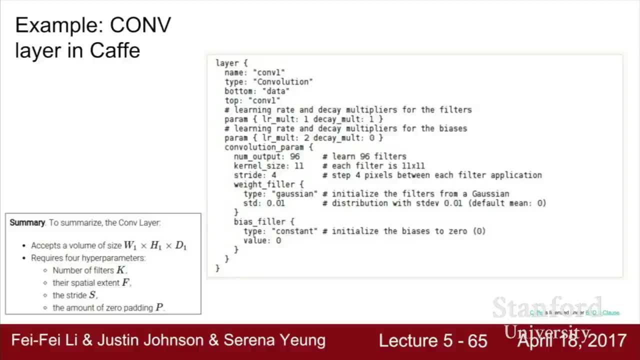 Right, and so if we look at another framework- CAFE- you'll see something very similar, where again, now, when you're defining your network, you define networks in CAFE using this kind of you know- prototext file where you're specifying. 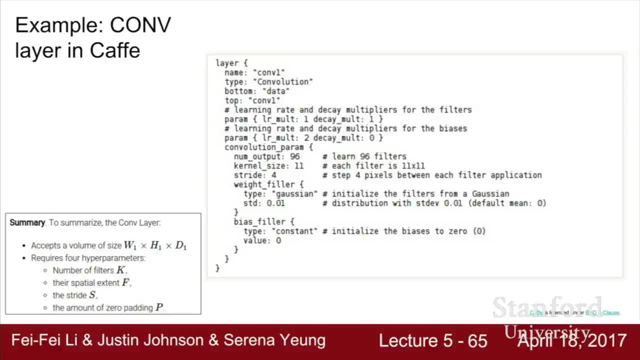 each of your design choices for your layer and you can see for a convolutional layer. we'll say things like: you know the number of outputs that we have. this is gonna be the number of filters for CAFE, as well as the kernel size and stride and so on. 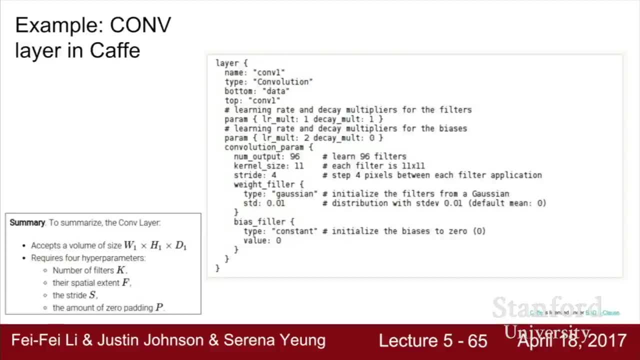 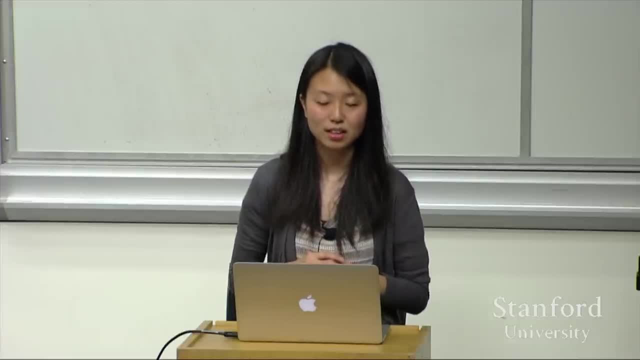 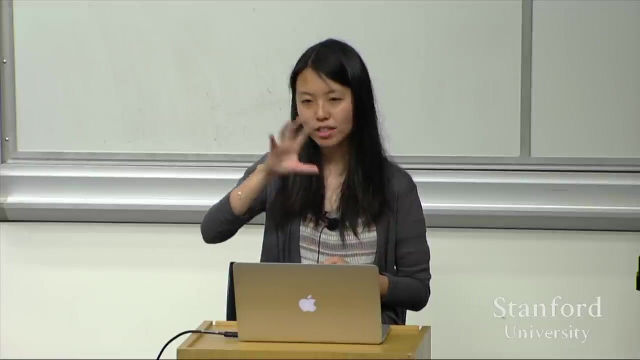 Okay, and so I guess, before I go on any questions about convolution, how the convolution operation works, Yes, Yeah. so the question is: what's the intuition behind how you choose your stride? And so at one sense it's kind of the resolution at work. 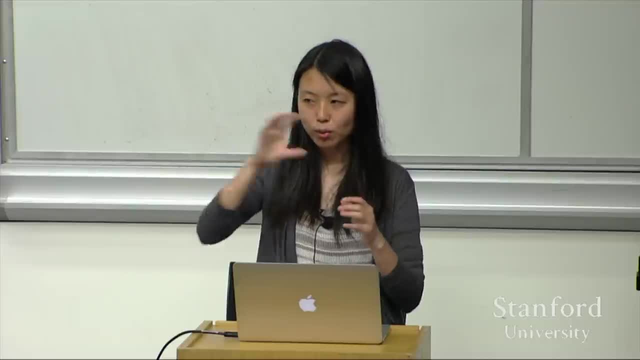 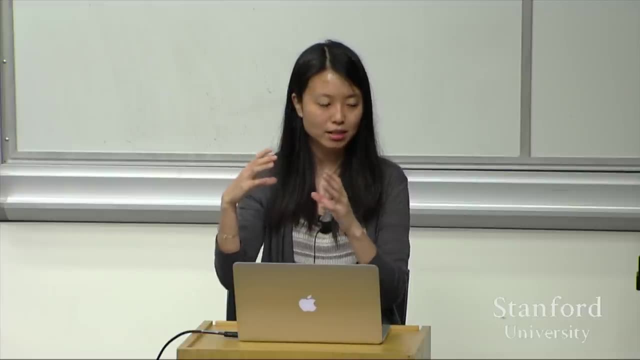 which you slide it on, and usually the reason behind this is because, when we have a larger stride, what we end up getting as the output is a down-sampled image. right, And so what this down-sampled image lets us have is. 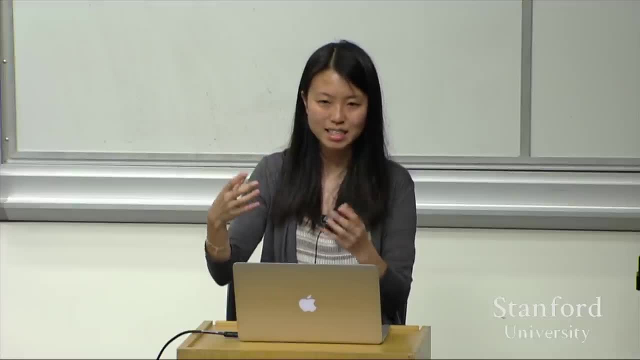 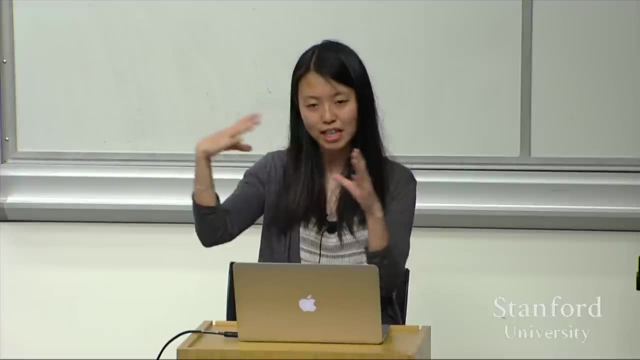 you know both. it's a way it's kind of like pooling in a sense, but it's just a different- and sometimes works better- way of doing. pooling is one of the intuitions behind this right, Because you get the same effect of down-sampling your image. 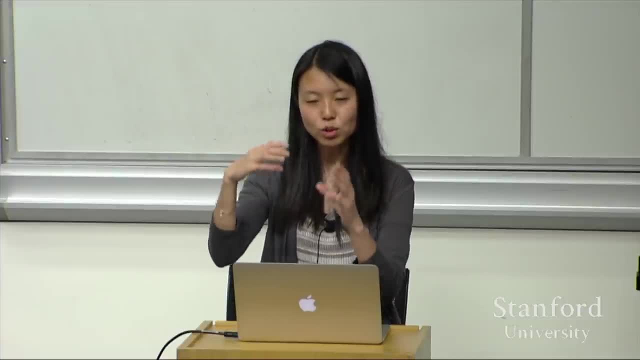 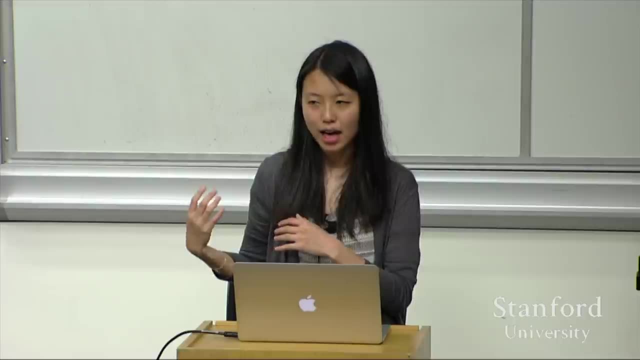 And then also, as you're doing this, you're reducing the size of the activation maps that you're dealing with at each layer, right, And so this also affects later on the total number of parameters that you have, because, for example, at the end of all your conv layers, 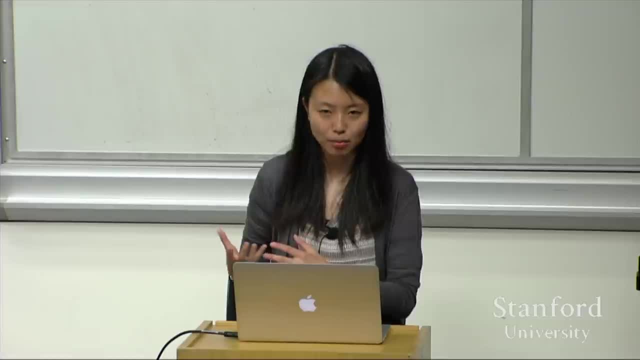 now you might put on fully connected layers on top, for example, and now the fully connected layer is gonna be connected to every value of your convolutional output, right? And so a smaller one will give you smaller number of parameters. And so now you can get into like: 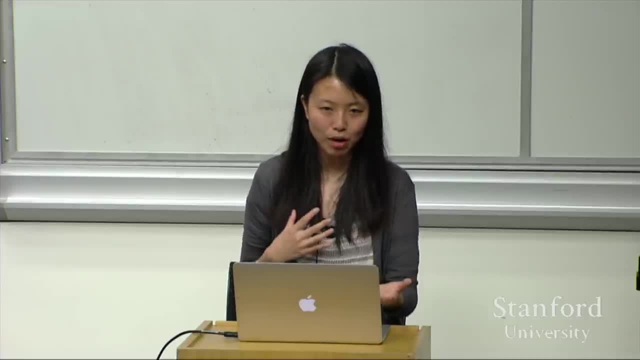 basically thinking about trade-offs of you know number of parameters. you have the size of your model overfitting things like that, And so, yeah, these are kind of the some of the things that you wanna think about with choosing your stride. 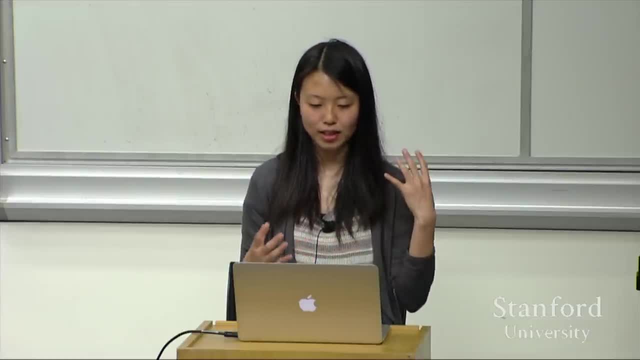 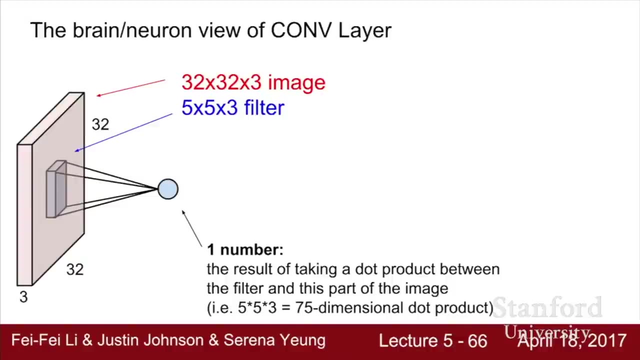 Okay, so now if we look a little bit at kind of the- you know, brain neuron view of a convolutional layer, similar to what we looked at for, you know, the neurons in the convolutional layer in the last lecture. so what we have is that: 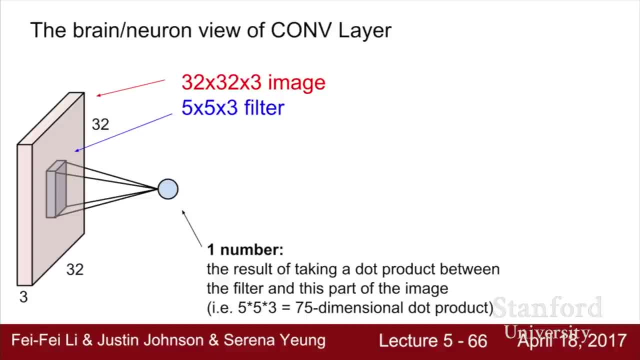 at every spatial location. we take a dot product between a filter and a specific part of the image right And we get one number out from here, And so this is the same idea of doing these types of dot products right, taking your input. 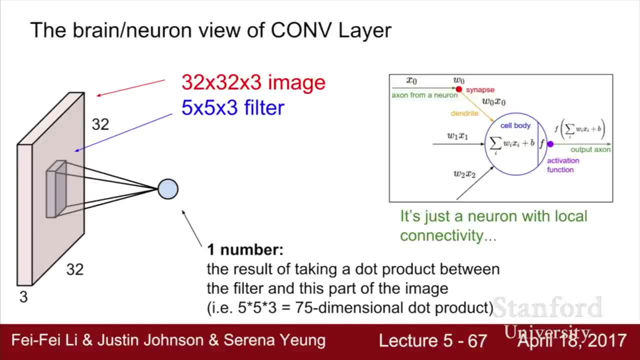 weighting it by these Ws right values of your filter, these weights that are the synapses, and getting a value out. But the main difference here is just that now your neuron has local connectivity, So instead of being connected to the entire input, 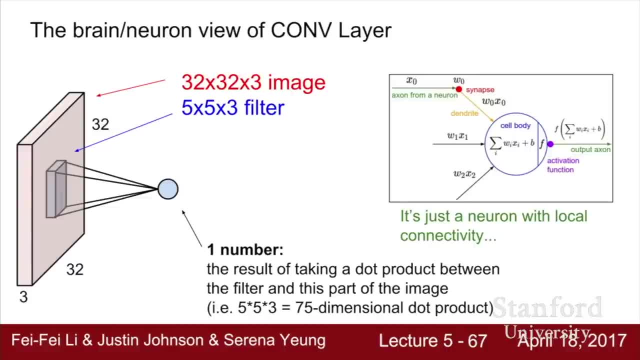 it's just looking at a local region spatially of your image, And so this looks at a local region and then now you're going to get kind of you know this, how much this neuron is being triggered at every spatial location in your image, right? 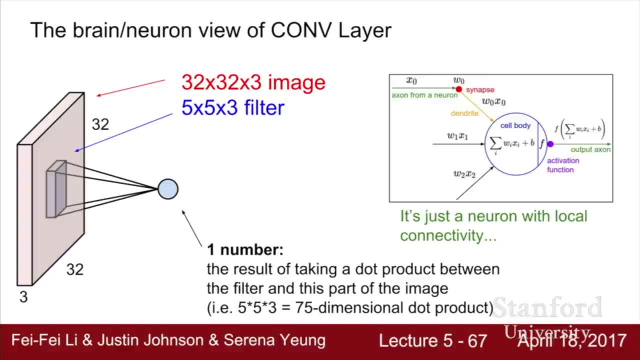 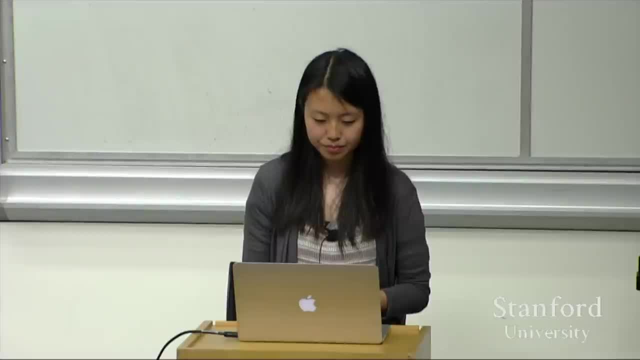 So now you preserve the spatial structure and you can say, you know, be able to reason on top of, on top of these kinds of activation maps in later layers, And just a little bit of terminology again for you know. 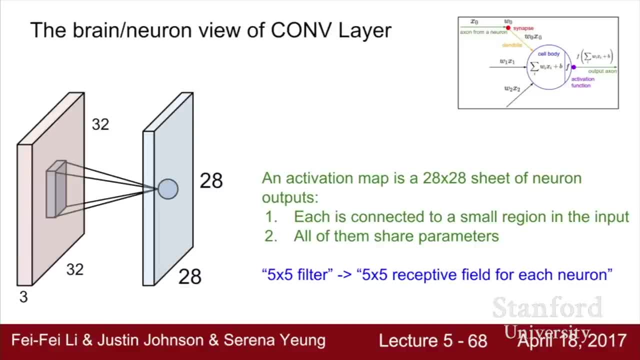 we have this five by five filter. We can also call this a five by five receptive field for the neuron, because this is the receptive field is basically the- you know- input field that this field of vision, that this neuron is receiving right. 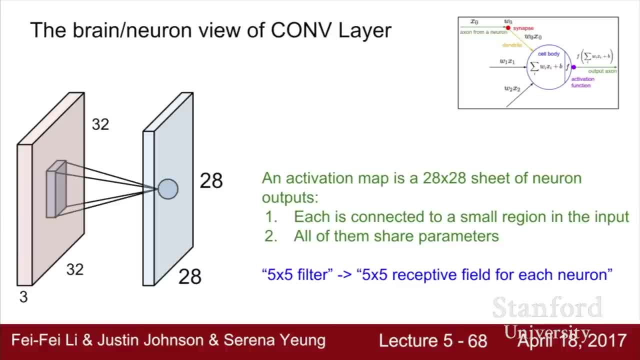 And so, yeah, so that's just another common term that you'll hear for this. And then again, remember each of these five by five filters. we're sliding them over to the spatial locations, but they're the same, you know. 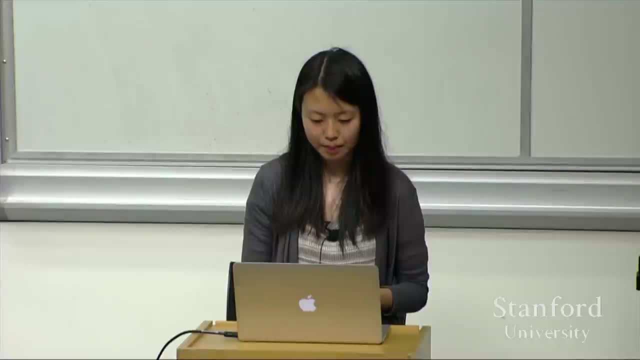 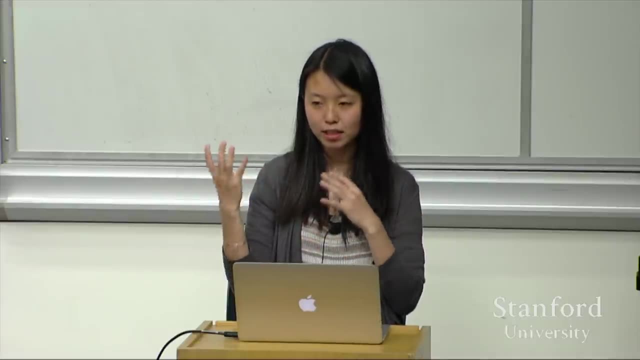 set of weights. They share the same parameters. Okay, and so you know, as we talked about, like, what we're going to get at this output is going to be this volume, right Where spatially we have, you know, let's say, 20 by 28,. 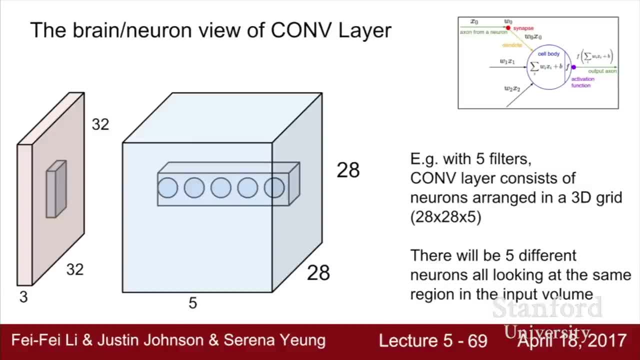 and then our number of filters is the depth, And so, for example, with five filters, what we're going to get out is this 3D grid that's 28 by 28 by five, And so if you look at the filters across in, you know one spatial location. 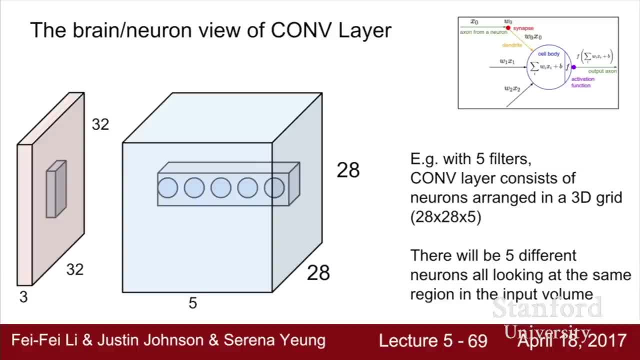 of the activation volume and going through depth. these five neurons, all of these neurons. basically, the way you can interpret this is they're all looking at the same region in the input volume, but they're just looking for different things, right? So there are different filters applied to the same spatial location in the image. 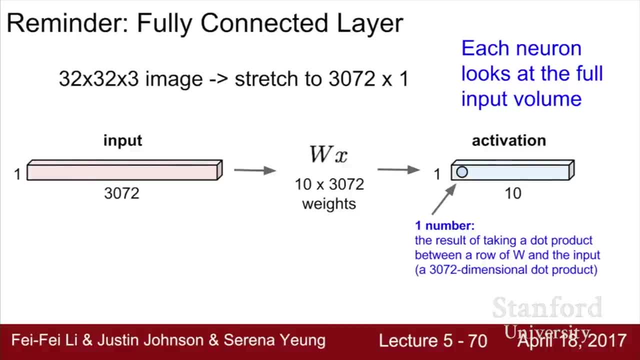 And so just a reminder again, kind of comparing with the fully connected layer that we talked about earlier. in that case, right, if we look at each of the neurons in our activation or output, Each of the neurons was connected to the entire stretched out input. 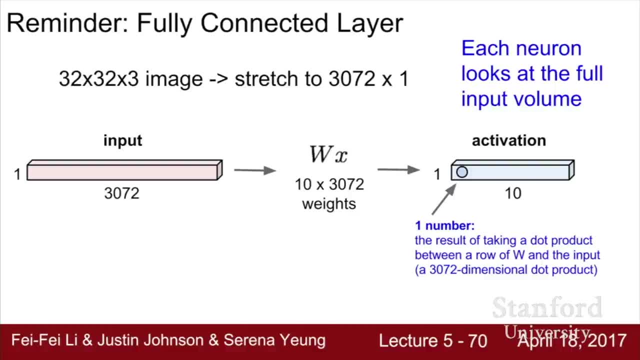 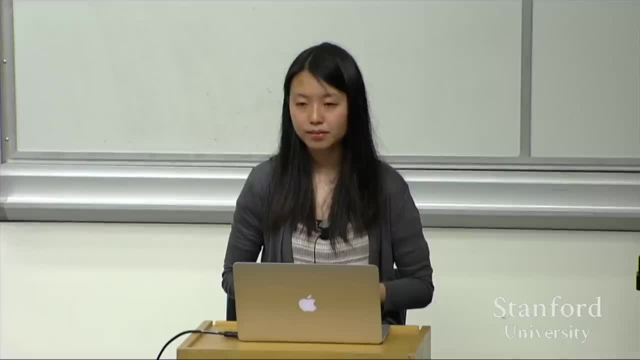 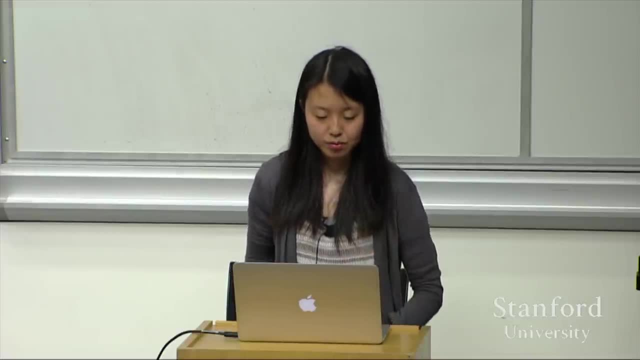 So it looked at the entire full input volume, compared to you know now where each one just looks at this local spatial region Question. Okay, so the question is: within a given layer, are the filters completely symmetric? So So what do you mean by symmetric exactly? I guess? 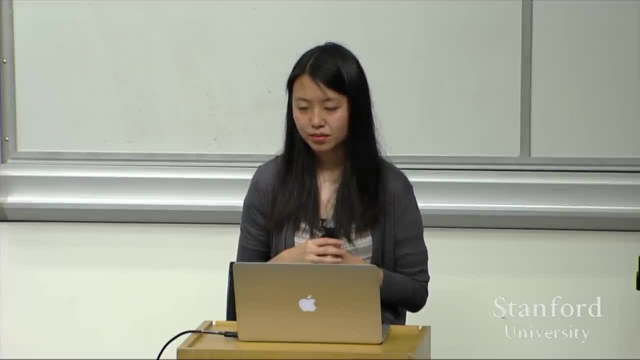 So okay. so the filters, you know, are the filters doing the same dimension, the same calculation? Yes, Okay. so is there anything different other than they have the same parameter values? No, so you're exactly right, right. 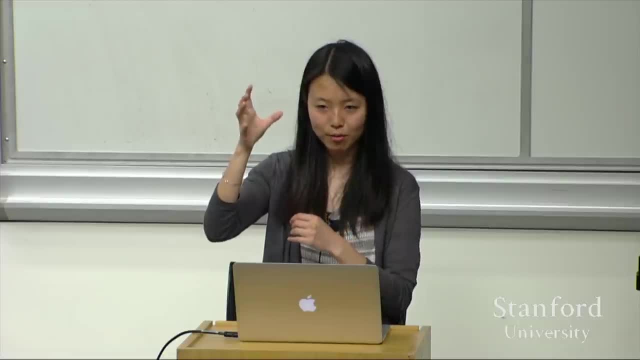 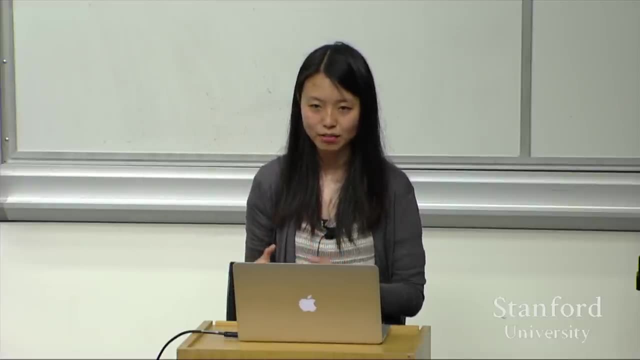 We're just taking a filter with a given set of, you know, five by five, by three parameter values and we just slide this in exactly the same way over the entire input volume to get an activation map. Okay, so you know, we've gone into a lot of detail on what these 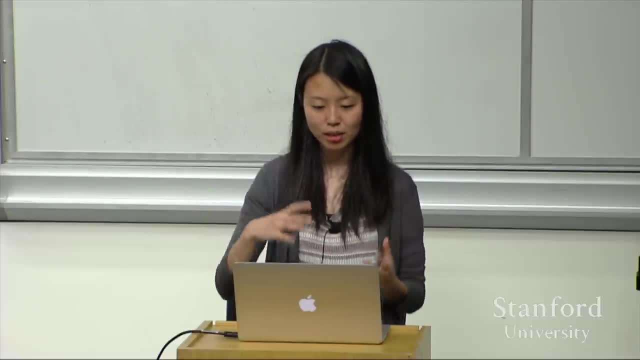 convolutional layers look like, And so now I'm just going to go briefly through the other layers that we have, that form, this you know, entire convolutional network, right? So remember again, we have convolutional layers interspersed with pooling layers. 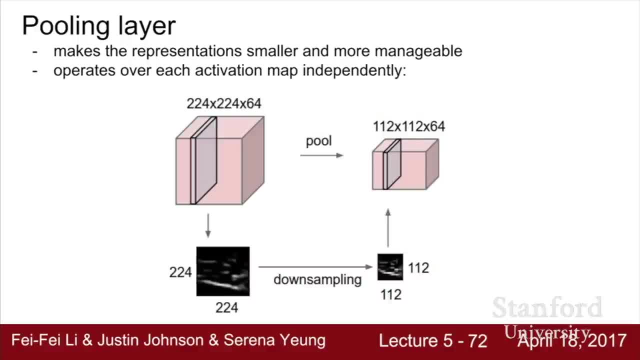 once a while, as well as these non-linearities. Okay, so what the pooling layers do is that they make the representations smaller and more manageable, right, So we talked about this earlier, when someone asked the question of why we would want to make the representation smaller. 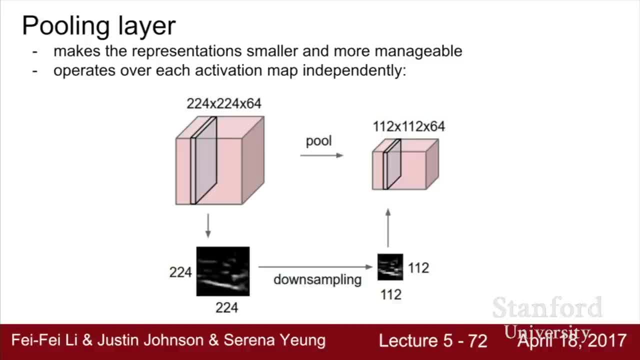 And so this is again for it to have you know fewer. it affects the number of parameters that you have at the end as well as, basically does some invariance over a given region, And so what the pooling layer does. 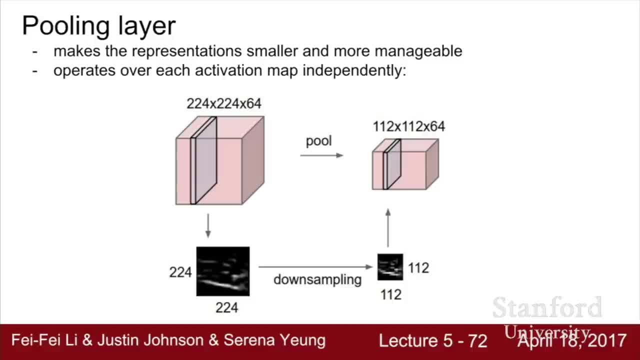 is, it does exactly just down samples and it takes your input volume- so, for example, 224 by 224 by 64, and spatially down samples this. So in the end you'll get out 112 by 112.. And it's important to note. 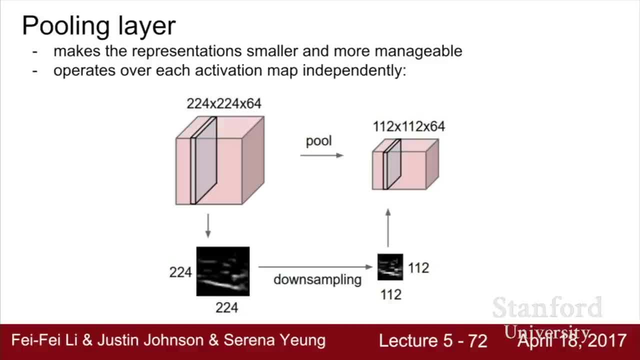 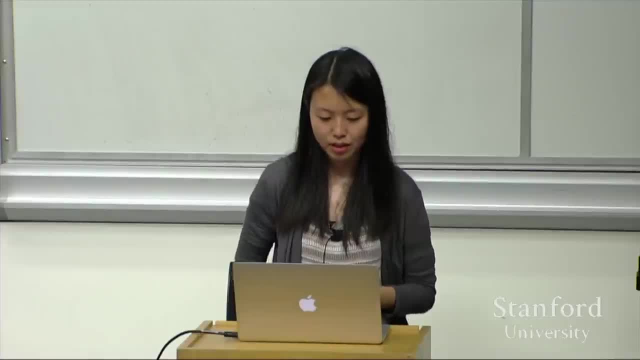 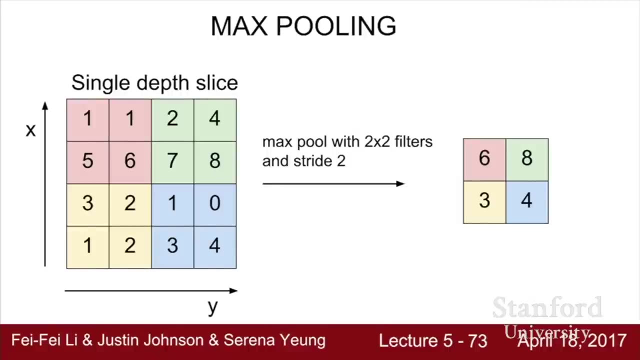 this doesn't do anything in the depth. We're only pooling spatially, So the number of your input depth is going to be the same as your output depth, And so, for example, a common way to do this is max pooling. So in this case, our pooling layer also has a filter size. 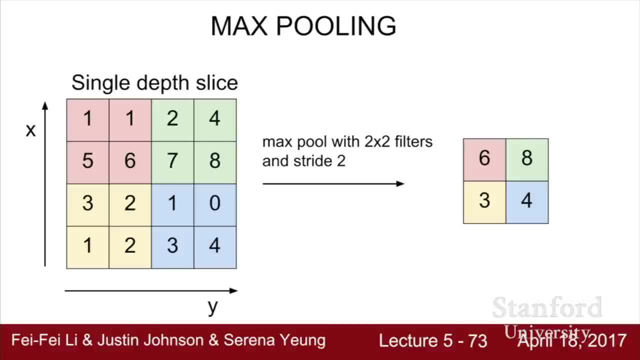 And this filter size is going to be the region at which we pool over. So in this case, if we have two by two filters, we're going to slide this, And so here we also have stride two in this case, So we're going to take this filter. 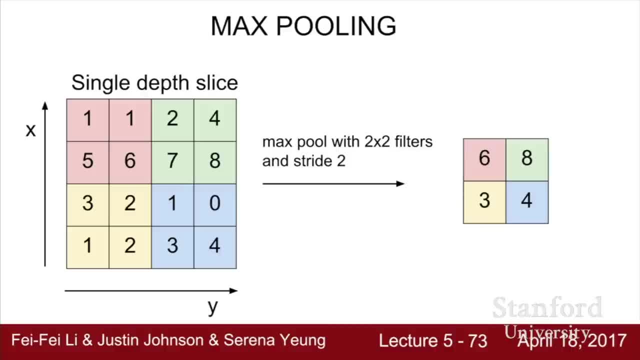 and we're going to slide it along our input volume in exactly the same way as we did for convolution, But here, instead of doing these dot products, we just take the maximum value of the input volume in that region, Right. so here, if we look at the red values, 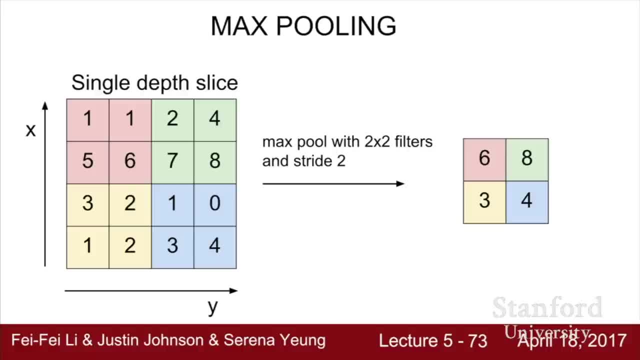 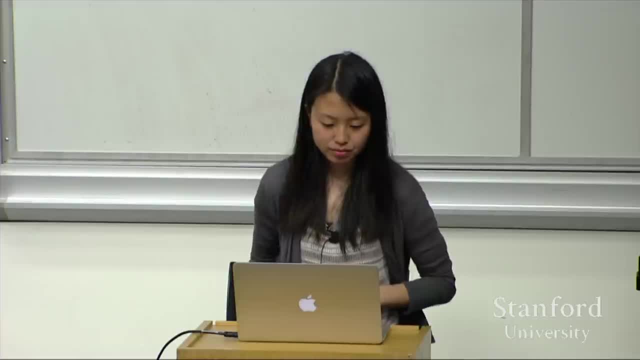 the value of that will be: six is the largest. If we look at the greens, it's going to give an eight and then we have a three and a four. Yes, question, Yeah. so the question is: is it typical to set up the stride so that there isn't an overlap? 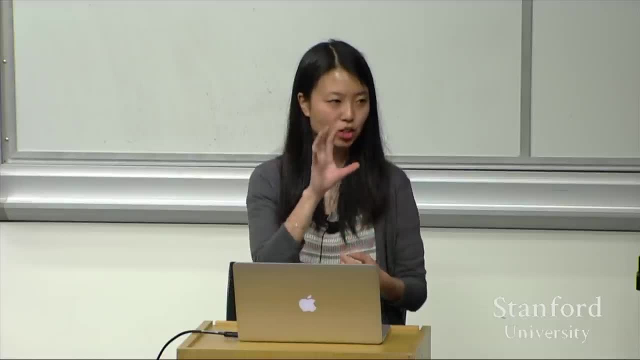 And yeah, so for the pooling layers it is, I think the more common thing to do is to have them not have any overlap, And I guess the way you can think about this is: you know, basically we just want a down sample. 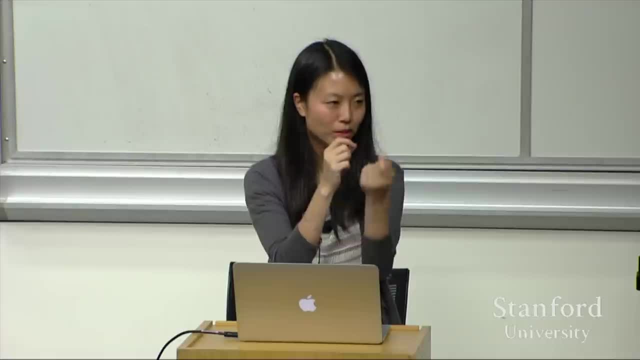 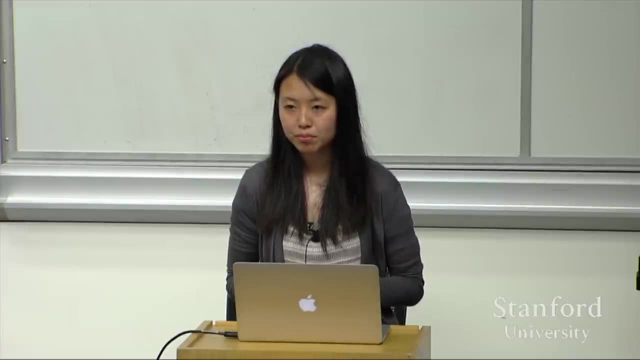 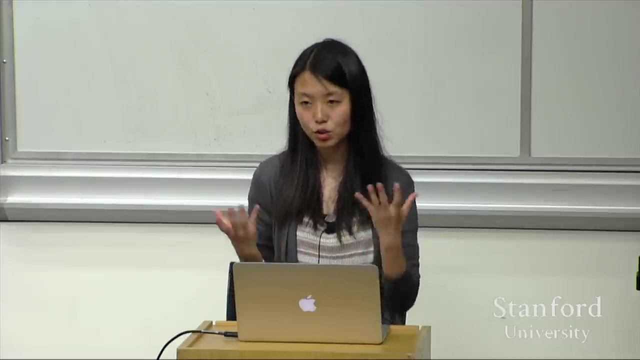 And so it makes sense to kind of look at this region and just get one value to represent this region, And then just look at the next region and so on. Yeah, Next question. So the question is: why is max pooling better than just taking the? 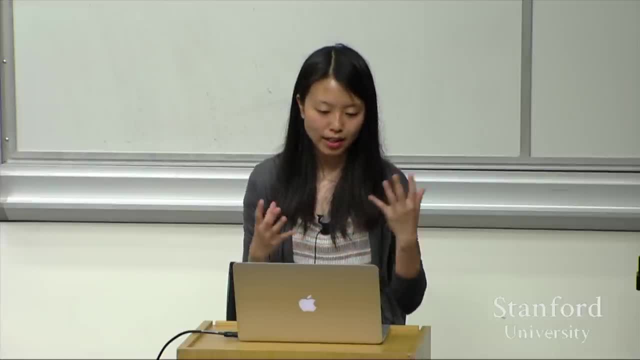 doing something like average pooling. Yes, that's a good point. Like average pooling is also something that you can do. An intuition behind why max pooling is commonly used is that you can have this interpretation of you know. if this is, these are. 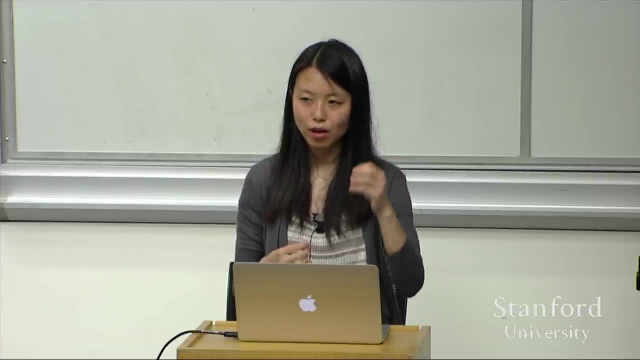 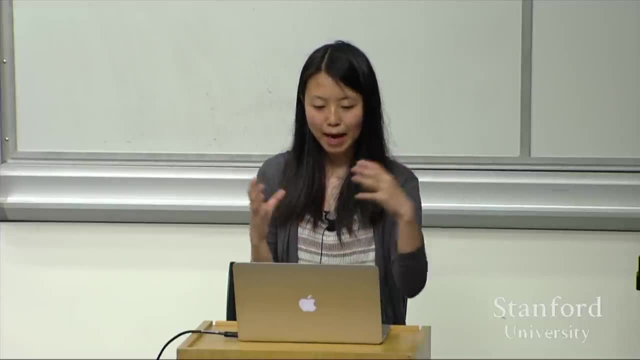 these are activations of my neurons, right, And so each value is kind of how much this part, this neuron, fired in this location, how much this filter fired in this location, And so you can think of max pooling as saying, you know, giving a signal of how. 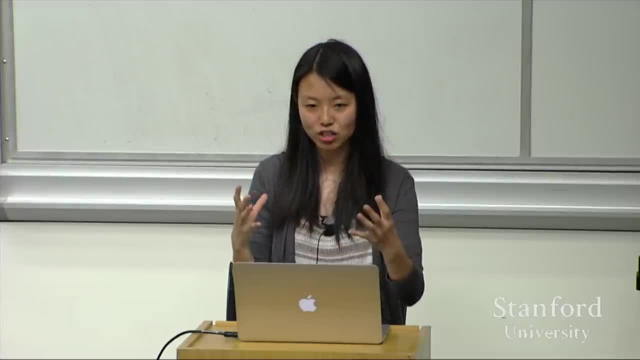 much did this filter fire at any location in this image? right, And if we're thinking about detecting, you know doing recognition, this might make some intuitive sense where you're saying, well, you know whether a light or whether some aspect of your image that you're looking for. 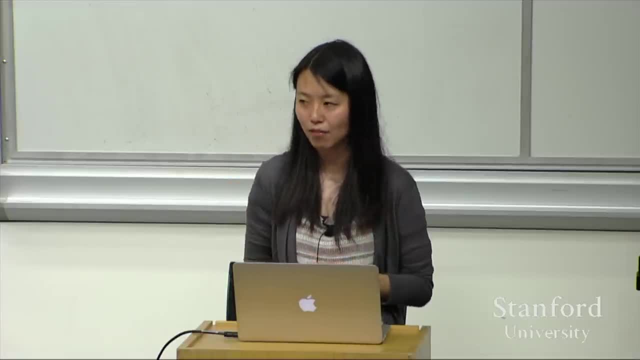 whether it happens anywhere in this region. we want to fire it at with a high. yeah, by value, no question. So the question is: since pooling and stride both have the same effect of downsampling, can you just use stride instead of pooling and so on? 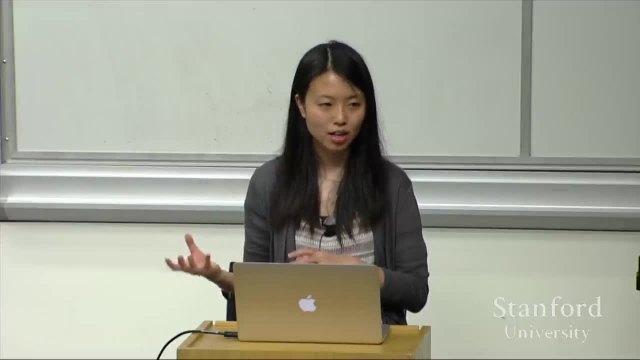 Yeah, and so in practice, I think, looking at more recent neural network architectures, people have begun to use stride more in order to do the downsampling instead of just pooling, and I think this gets into things like also fractional strides and things that you can do. 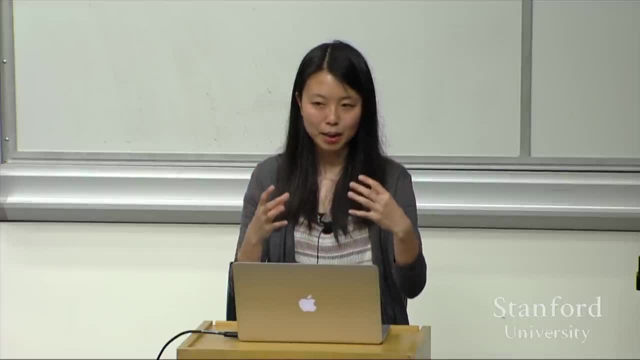 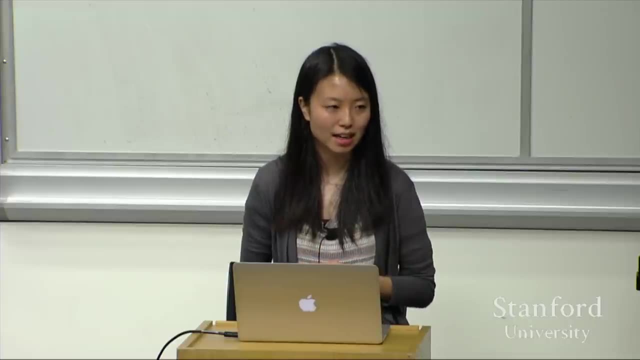 but in practice this in a sense, maybe has been a little bit better way to get better results using that. So, yeah, so I think using stride is definitely. you can do it and people are doing it. Okay, so let's see where were we. 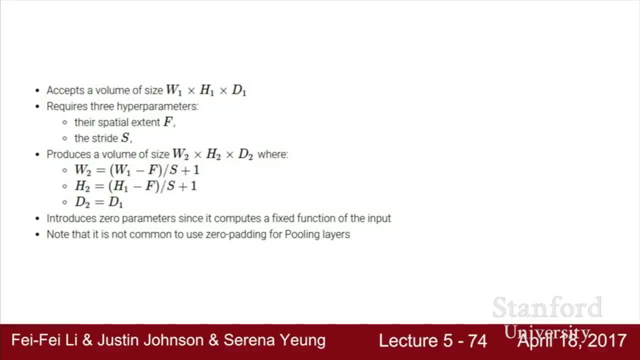 Okay, so, yeah, so with these pooling layers, we've got some basic information about so, again, there's some design choices that you make. You take this input volume of w by h, by d, and then you're going to set your hyperparameters. 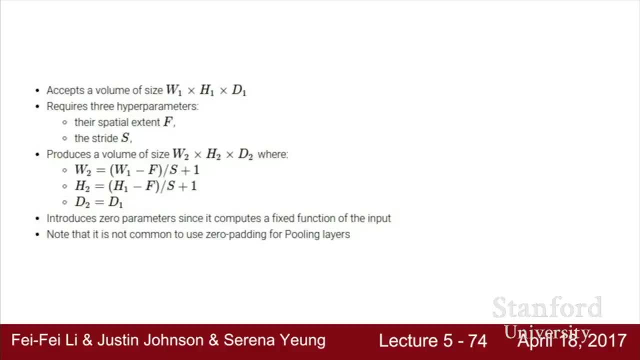 for design choices of your filter size with a spatial extent over which you're pooling, as well as your stride, and then you can again compute your output volume using the same equation that you used earlier for convolution. it still applies here, So we still have our w total extent minus filter size, divided by stride plus a. 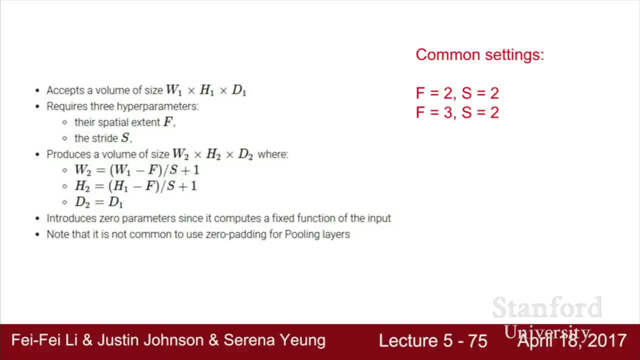 So that's one, Okay, and so just one other thing to note. it's also typically people don't really use zero padding for the pooling layers, because you're just trying to do a direct downsampling. So there isn't this problem of like. 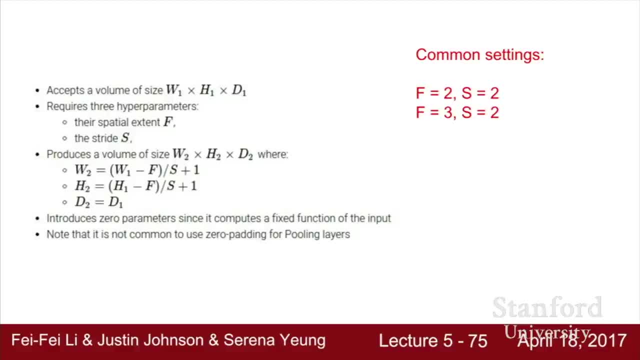 applying a filter at the quarter and having some part of the filter go off your input volume, And so for pooling, we don't usually have to worry about this and we just directly downsample. So some common settings for the pooling layer is the filter size of two by two or three by three. 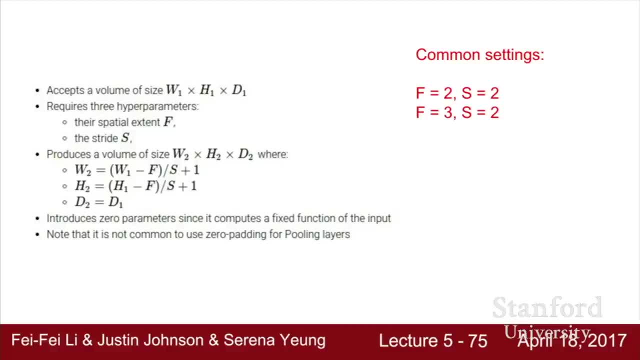 strides two by two, you know you can have. also you can still have pooling of two by two, even with the stride of, even with the filter size of three by three. I think someone asked that earlier. but in practice it's pretty common just to have. 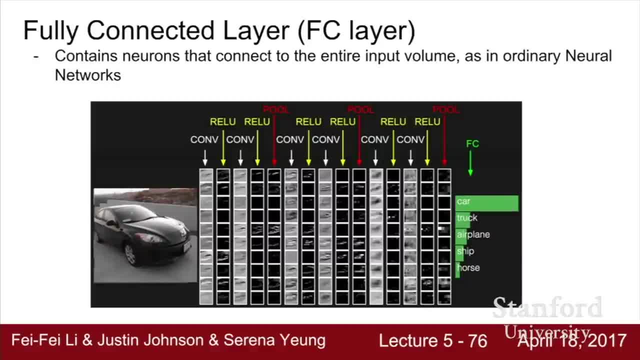 yeah, two by two. Okay, so now we've talked about these convolutional layers. The Rayleigh layers were the same as what we had before with the, with the, you know, just the base neural network that we talked about last lecture. 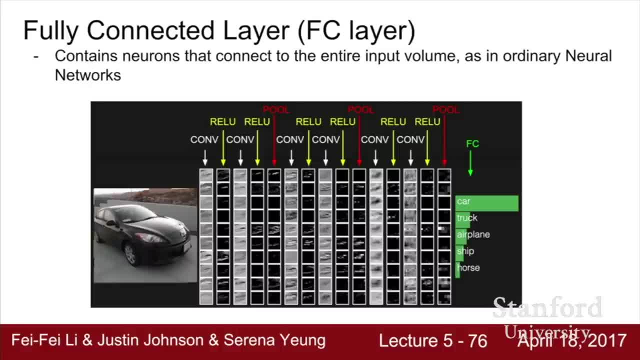 So we intersperse these and then we have a pooling layer, every you know, once in a while when we feel like downsampling, right, And then the last thing is that at the end, we want to have a fully connected layer, And so this will be just exactly the same. 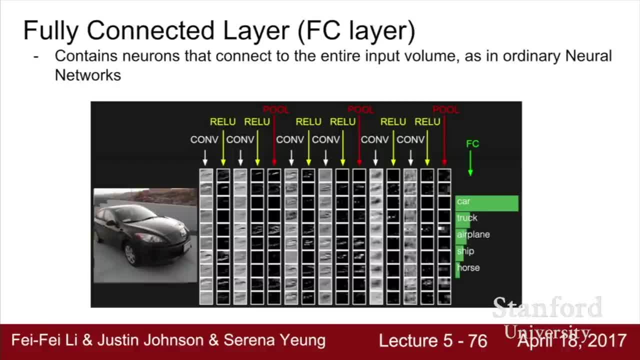 as the fully connected layers that you've seen before. So in this case, now, what we do is we take the convolutional, convolutional network output. We, the last layer, we have some volumes that we're gonna have width by height, by some depth. 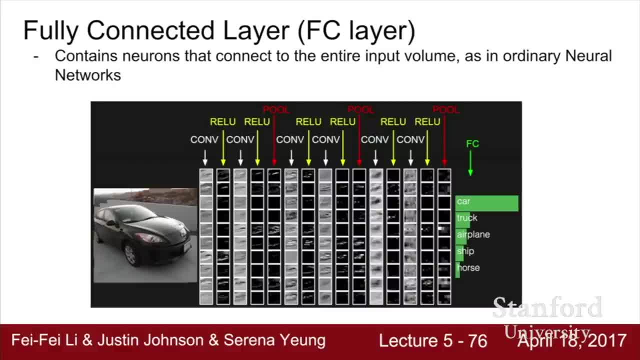 And we just take all of these and we essentially just stretch these out, right, And so now we're going to get the same kind of- you know, basically 1D input that we're used to for a vanilla neural network, And then we're going to apply. 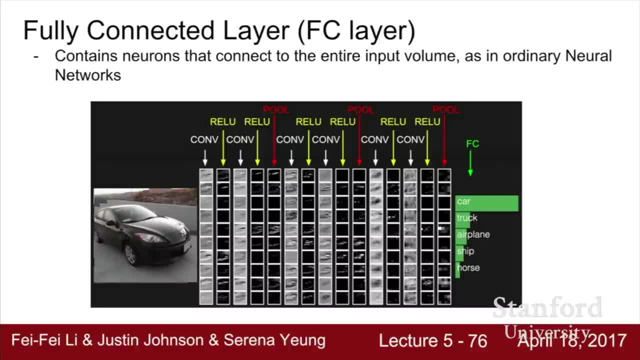 this fully connected layer on top. So now we're going to have connections to every one of these of these convolutional map outputs. So what you can think of this is basically now, instead of preserving- you know, before we were preserving spatial structure, right? 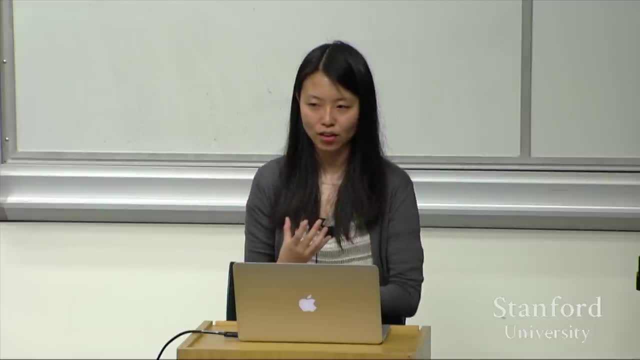 And so, but at the last layer, at the end, we want to aggregate all of this together and we want to reason basically on top of all of this, as we had before, And so what you get from that is just our- you know- score outputs, as we had earlier. 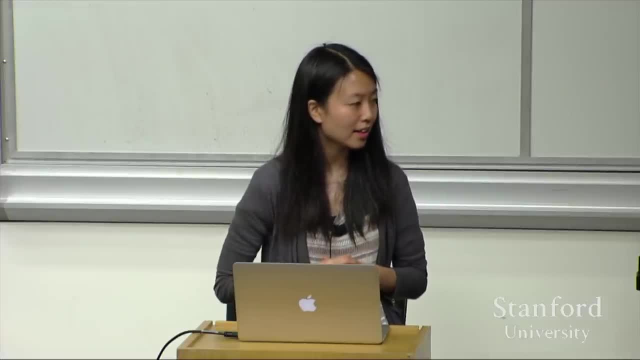 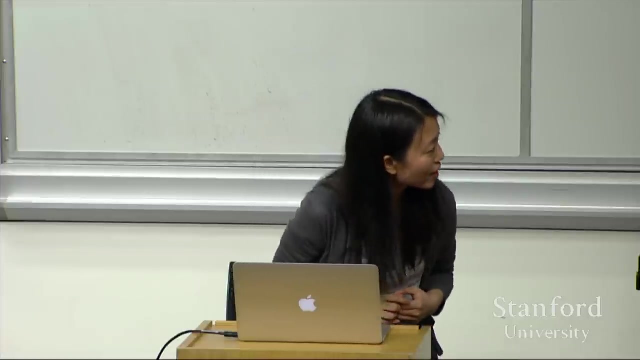 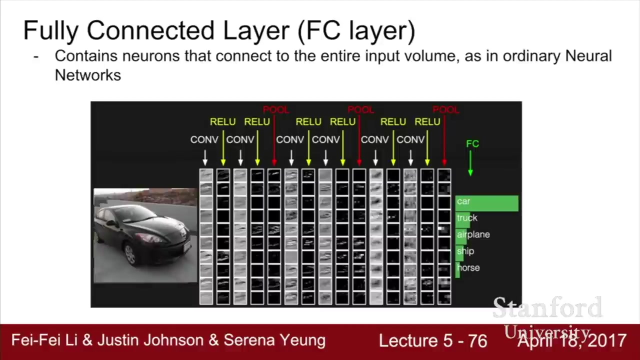 Okay, Okay. so the question is: what are the 16 pixels that are on the far right? Do you mean the Oh each column, The green ones or the black ones? The one with hold on pool? Oh, okay. 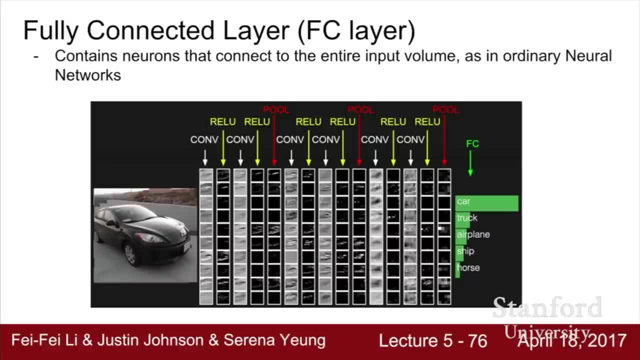 Yeah. so the question is, how do we interpret this column right, for example, at pool, And so what we're showing here is each of these columns is the output activation maps, right, The output from one of these layers. And so, starting from the beginning, 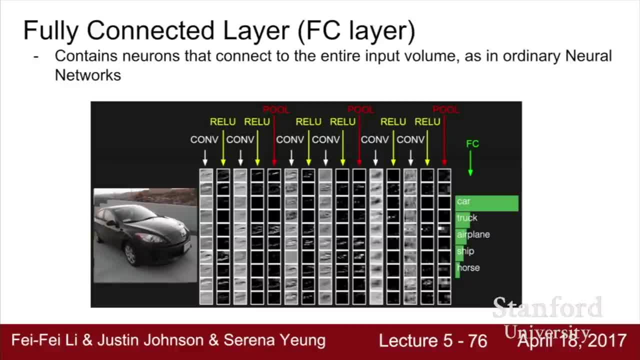 we have our car. after the convolutional layer, we now have these activation maps of each of the filters slid spatially over the input image. Then we pass that through a ReLU so you can see the values coming out from there and then going all the way over. 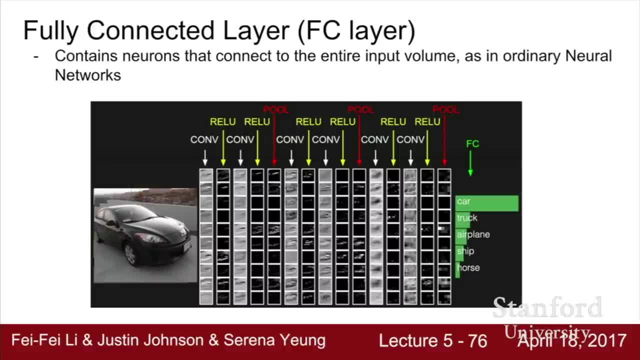 And so what you get for the pooling layer is that it's really just taking the output of the ReLU layer that came just before it, and then it's pooling it. So it's going to downsample it, right, And then it's going to take the max value. 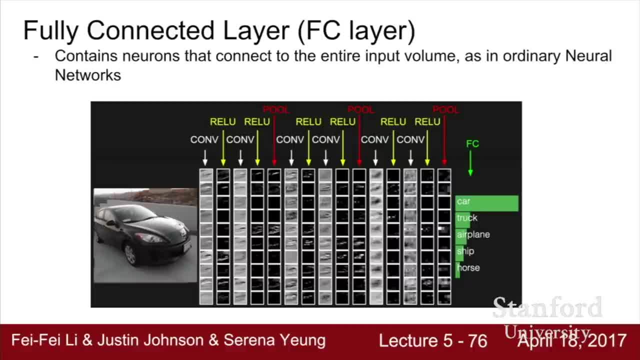 in each filter location. And so now, if you look at this pool layer output, like, for example, the last one that you were mentioning, it looks the same as this ReLU output, except that it's downsampled and that it has this kind of max value. 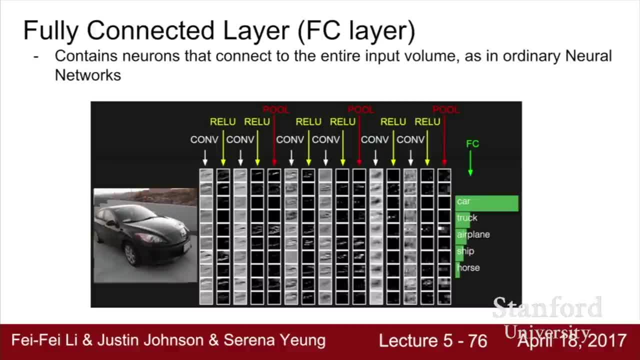 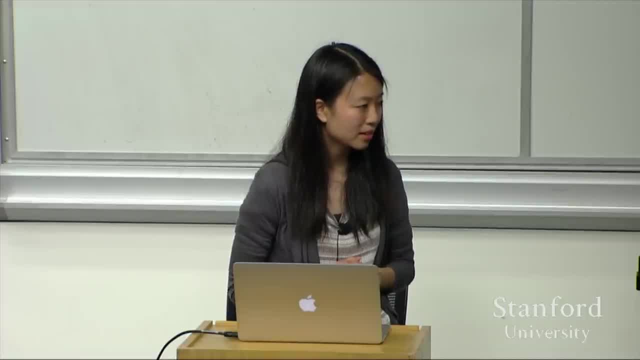 in every spatial location, And so that's the minor difference that you'll see between those two. So the question is now like: this looks like just a very small amount of information, right? so how can it know to classify from here? And so the way that you should think about this. 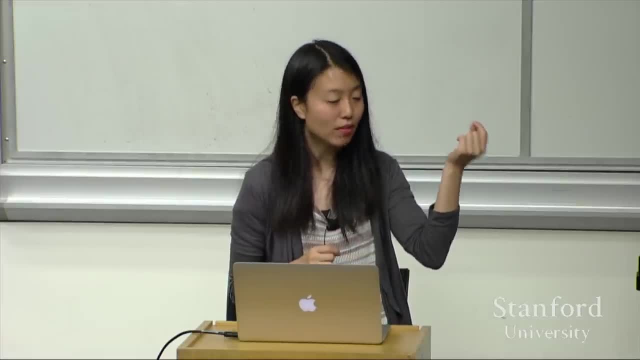 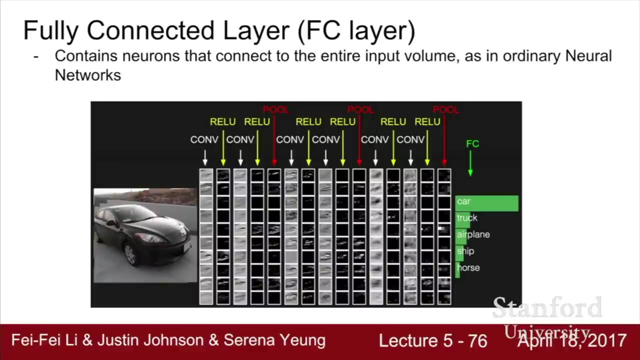 is that each of these values inside one of these pool outputs is actually- it's the accumulation of all the processing that you've done in the pool, You've done throughout this entire network, right? So it's at the very top of your hierarchy. 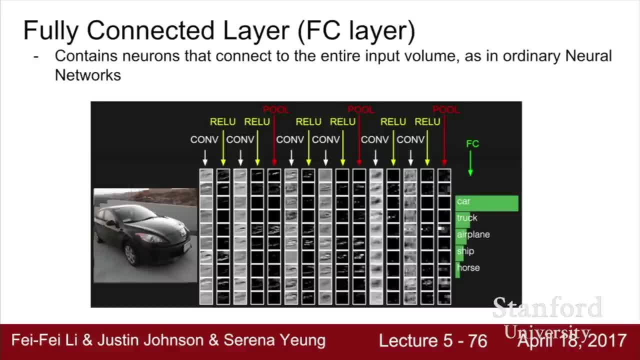 And so each actually represents kind of a higher level concept. So we saw before you know, for example, Hubel and Wiesel and building up these hierarchical filters where at the bottom level we're looking for edges, right Or things like very simple structures like edges. 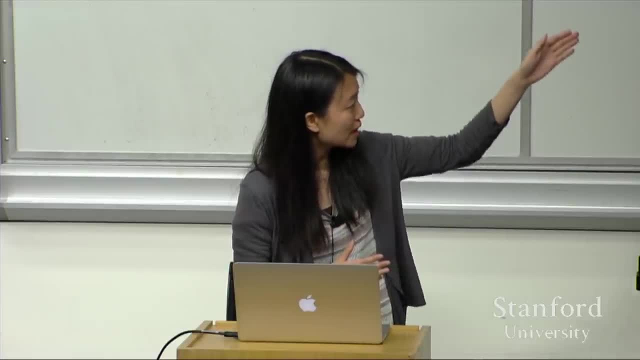 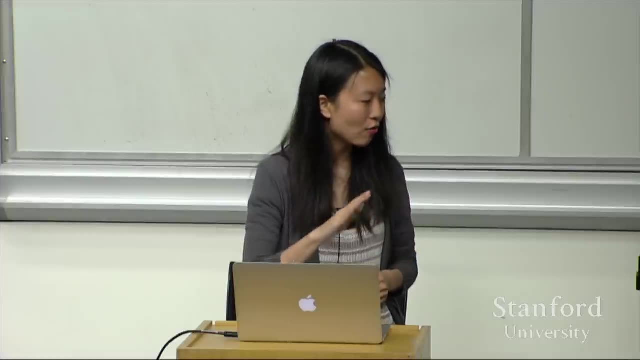 And so, after your convolutional layer, the outputs that you see here in this first column is basically: how much do specific, for example, edges fire at different locations in the image? But then as you go through you're gonna get more complex. 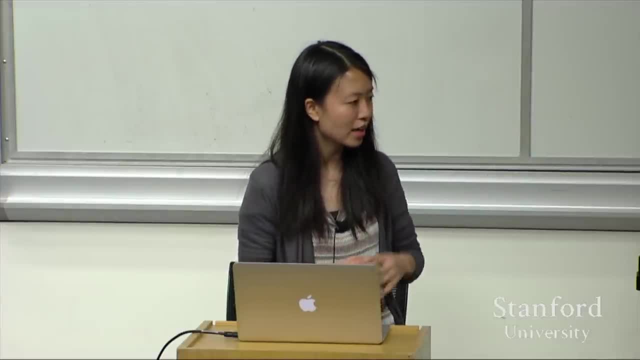 it's looking for more complex things, right? And so the next convolutional layer is going to fire at how much you know? let's say, certain kinds of corners show up in the image, right, Because it's reasoning. it's input is not the original image. 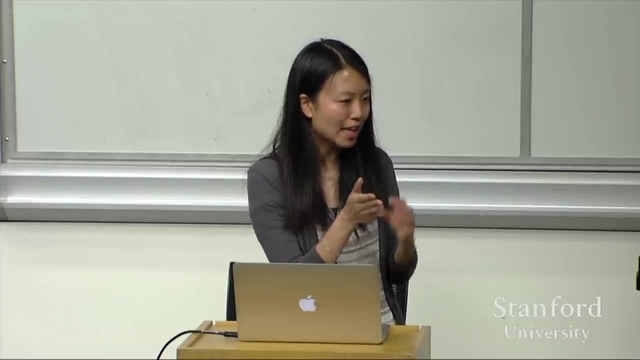 it's input is the output. it's already. you know the edge maps right, So it's reasoning on top of edge maps, And so that allows it to get more complex, detect more, more complex things, And so by the time you get all the way up. 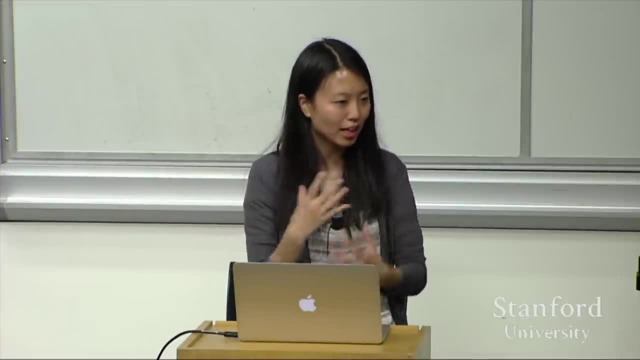 to this last pooling layer. each value is representing how much a relatively complex you know sort of template is firing right, And so because of that, now you can just have a fully connected layer. you're just aggregating all of this information together to get you know. 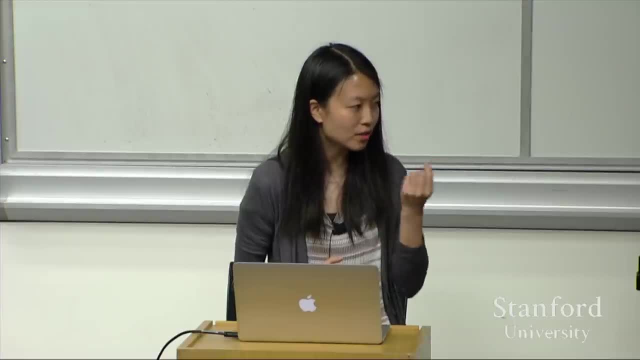 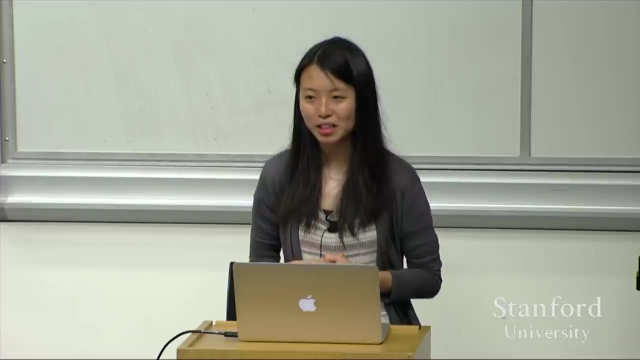 a score for your class. So each of these values is how much a pretty complicated, complex concept is firing. So that's kind of a question. So the question is, when do you know you've done enough pooling to do the classification? And the answer is: you just try and see. 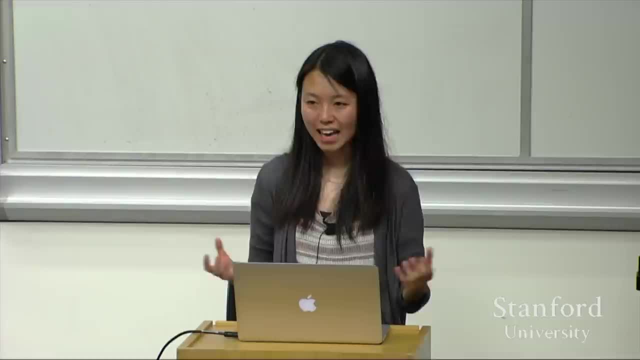 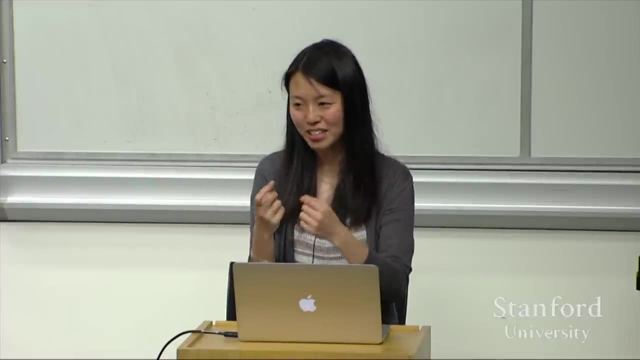 So in practice, you know these are all design choices and you know you can think about this a little bit intuitively. right, Like you want to pool, but if you pool too much you're going to have very few values. 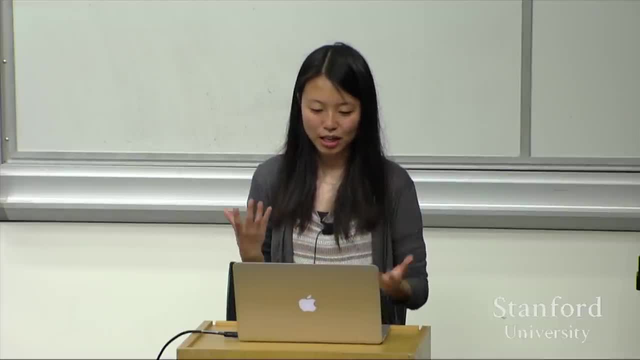 like representing your entire image and so on. So it's just kind of a trade off: something reasonable right, Something reasonable versus. people have tried a lot of different configurations, so you'll probably cross-validate right and try over different pooling sizes. 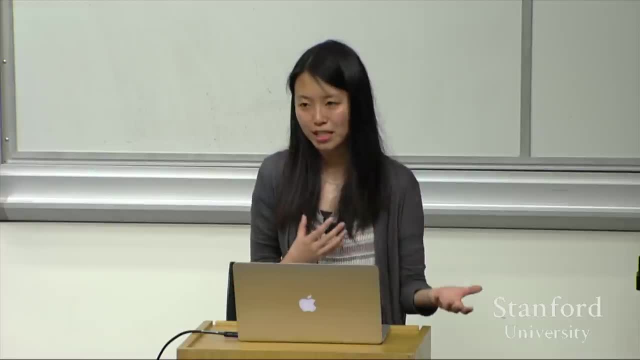 different filter sizes, different number of layers, and see what works best for your problem. Because, yeah, like every problem with different data is going to, you know, different set of these sorts of hyperparameters might work best. Okay, so last thing, just wanted to point you guys to this demo. 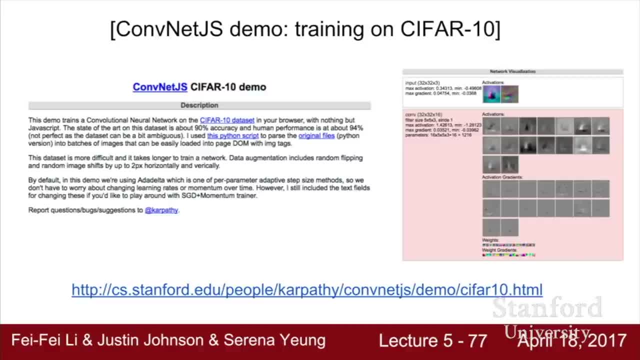 of training a comnet, which was created by Andrej Karpathy, the originator of this class, And so he wrote up this demo where you can basically train a comnet on CIFAR-10, the data set that we've seen. 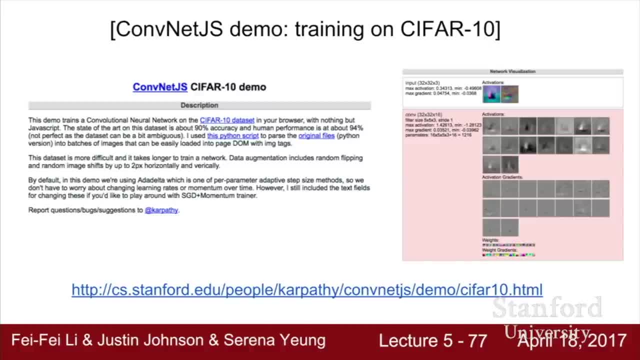 before right with 10 classes. And what's nice about this demo is you can. it basically plots for you what each of these filters look like, what the activation maps look like. so some of the images I showed earlier were taken from this demo. 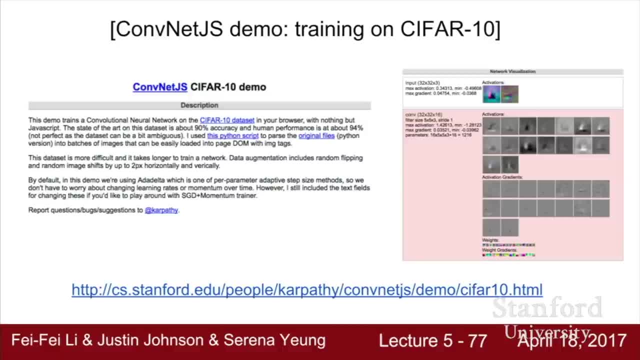 So you can go try it out, play around with it and you know, just go through and try and get a sense for what these activation maps look like. And just one thing to note: usually you know the first layer activation maps are. 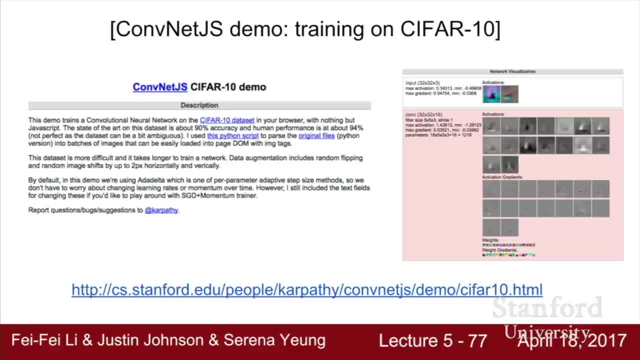 you can interpret them right because they're operating directly on the input image, so you can see what these templates mean. As you get to higher level layers it starts getting really hard like how do you actually interpret? what do these mean? 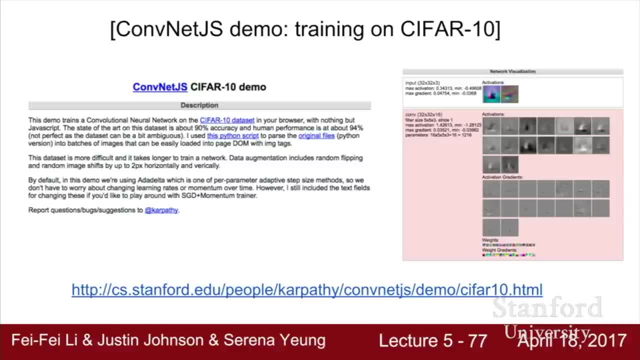 So for the most part, it's just hard to interpret, so you shouldn't? you know? don't worry if you can't really make sense of what's going on, but it's still not a problem. Okay, so I'm going to go ahead and show you guys some of these. 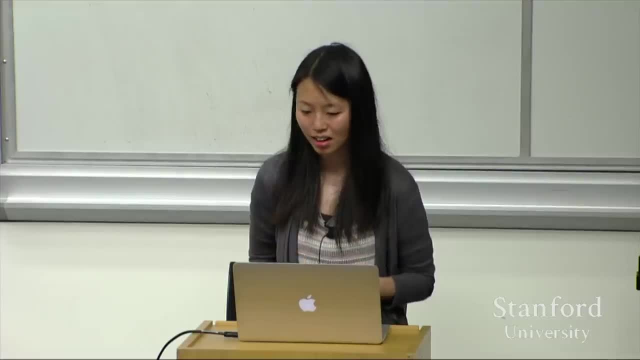 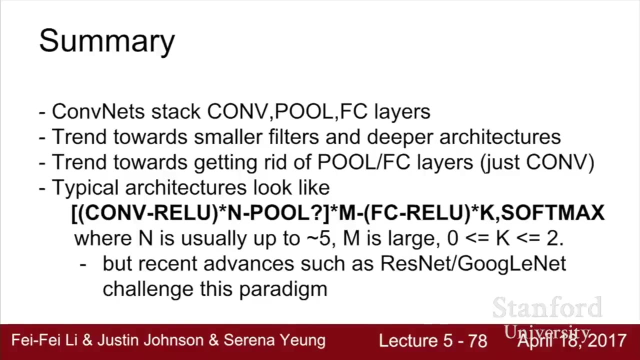 Okay, so I'm going to go ahead and show you guys some of these, And it's nice just to see the entire flow and what outputs are coming out. Okay, so, in summary, so today we talked about how convolutional neural networks work.